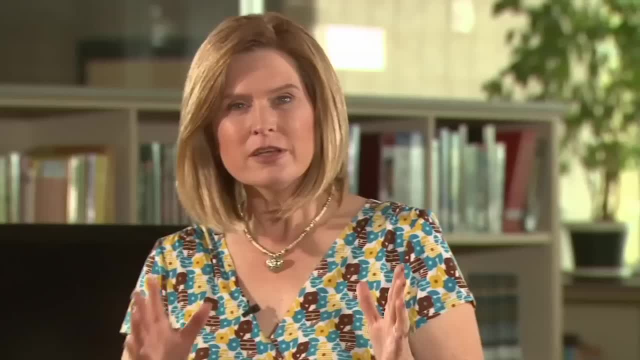 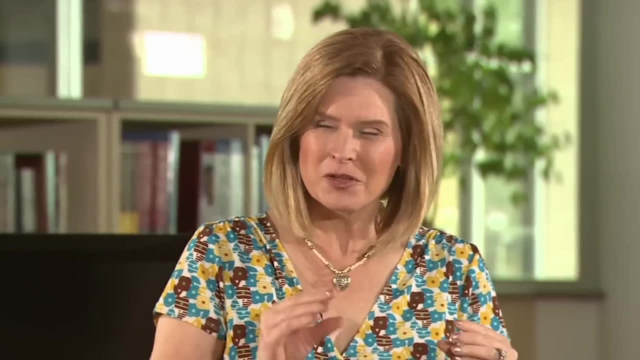 talk about the Emergent Literacy Skills. we always say: now, what are the Emergent Literacy Skills? They look at us like, hmm, I think I've remembered that or I think I've heard that, but I can't really remember what they are. This particular workshop we're going. 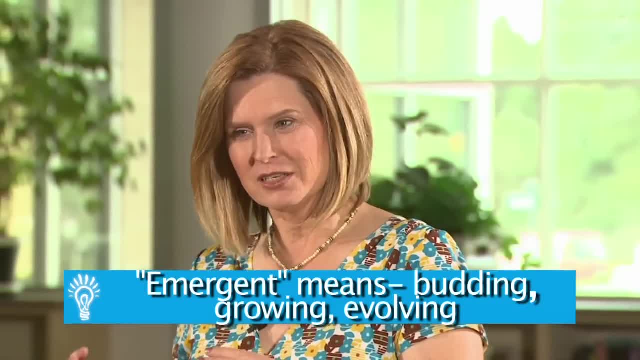 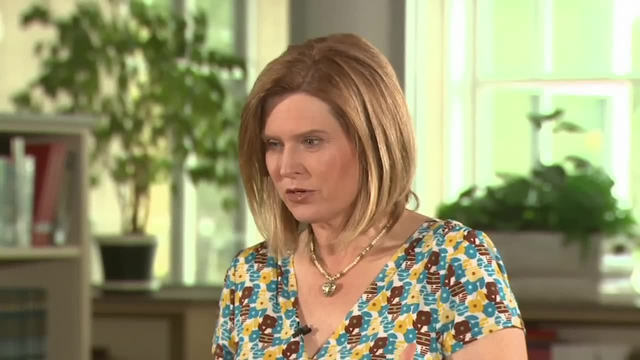 to talk about emergent literacy skills and what they are. To break that down, we're going to talk about what is emergent. Does anyone know what emergent is? What does emergent mean, Sharon? do you know what emergent means? 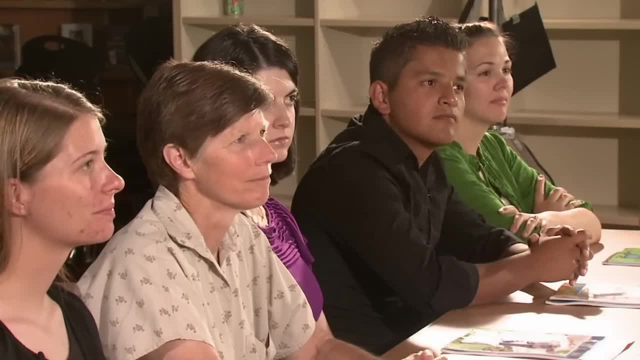 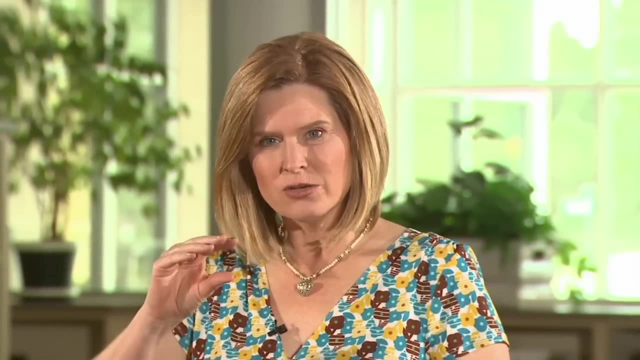 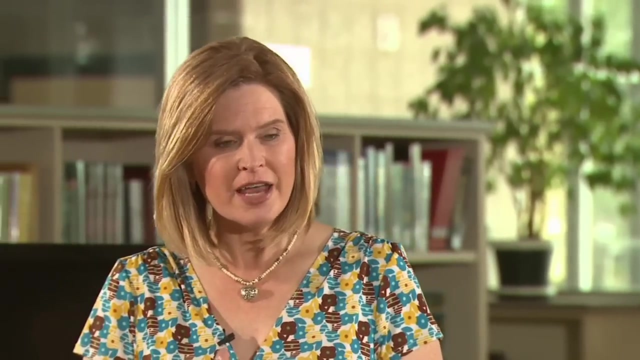 Just beginning. Yes, Thank you. Perfect answer Just beginning. We're not talking about being able to read. We're talking about what you can do so your child will be prepared, or when they go to school, that they can learn to read. There are five emergent literacy: 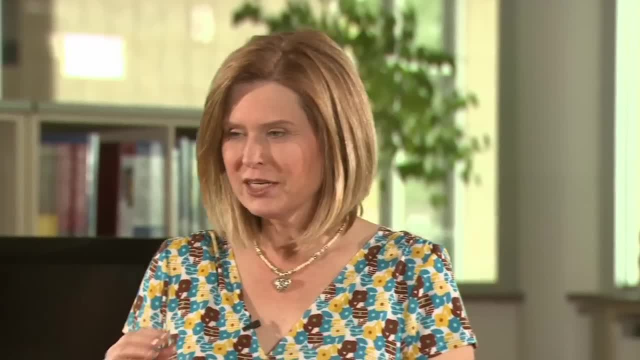 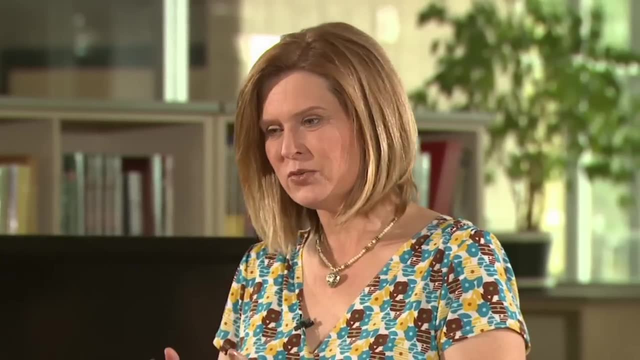 skills that we're going to break down today and really discuss. We're going to show some clips that actually back up the things that we're talking about. We're not going to be doing the learning triangle as much, but the clips that you'll 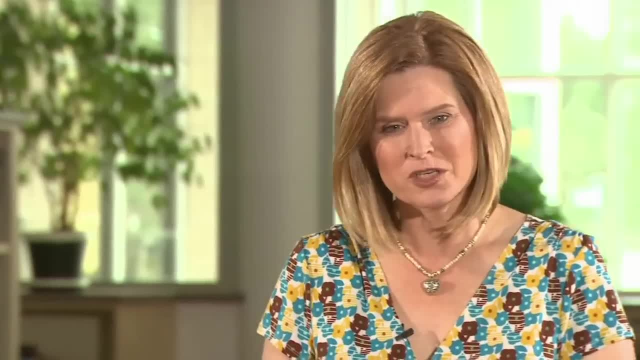 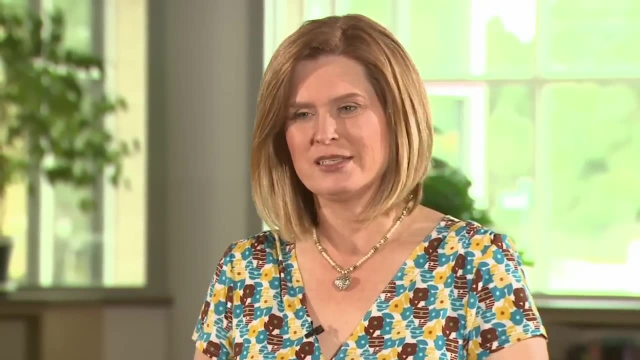 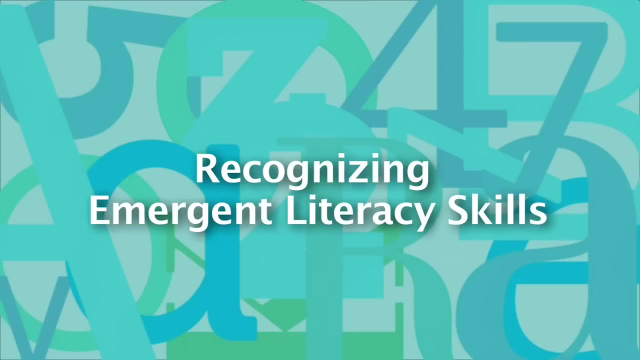 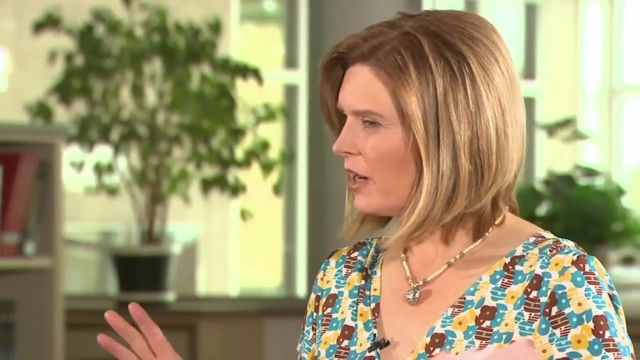 see from our PBS shows will just support the areas that we're talking about. Remember, emergent literacy skills. What can you do to start the learning process, Those five emergent literacy skills that we've talked about? I'm going to have you guys. 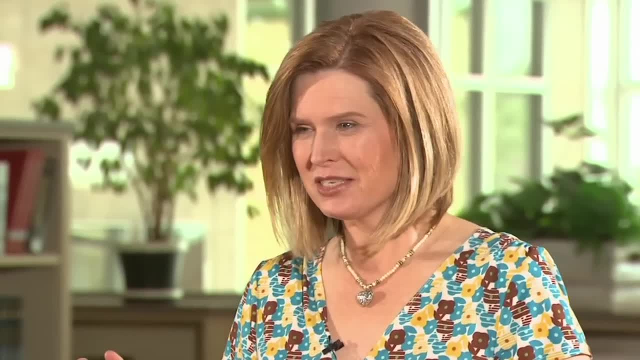 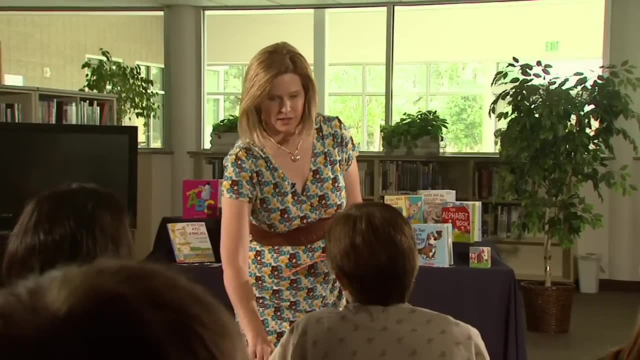 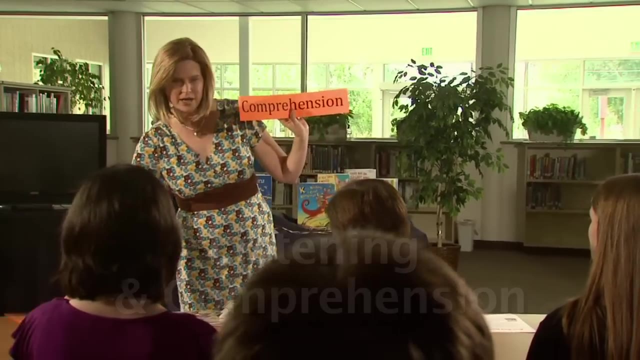 as a group, just silently, not silently, but I want you to discuss In these five areas- I've got writing, I've got decoding, I've got talking, listening and comprehension. I want you, as your table, to discuss what would come first for a child to learn how to read. 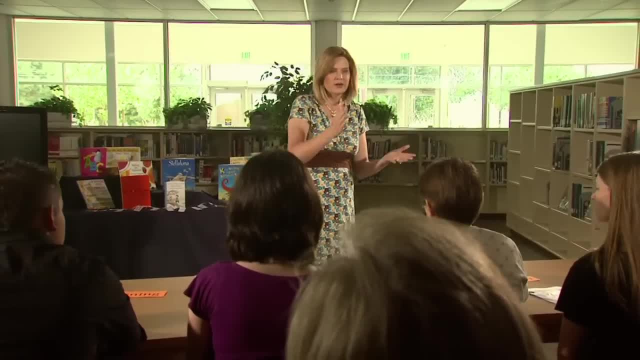 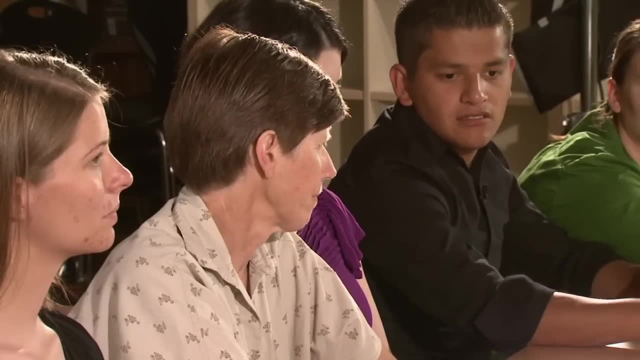 What would you need to do first so a child could eventually learn how to read once they enter school? So just take a few minutes and put those in order Once again. we've got listening, writing, decoding, talking and comprehension. I think it's them. 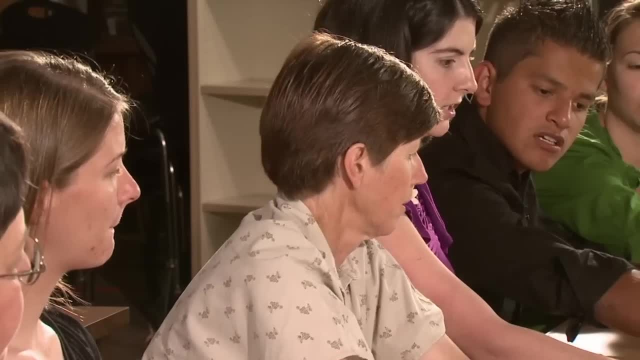 Yeah. And then I think writing: Oh, decoding, Decoding before talking. Yeah, I think you've got to get comprehension before writing. Yeah, Decoding is kind of like getting the point of the message right. Decoding- Maybe comprehension before talking too. 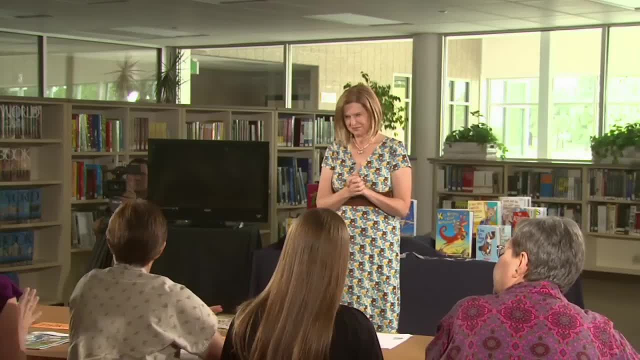 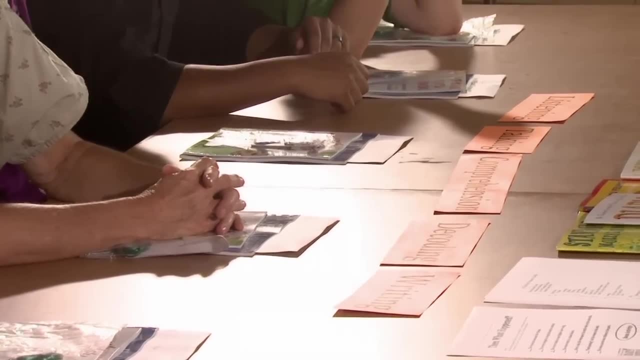 Comprehension, Yeah, I think comprehension Decoding the words. That's not the story. They can understand, Yeah, They can understand. Yeah, They can understand what you're saying. Well, but if you listen and know what the child is doing, then you start to talk back. 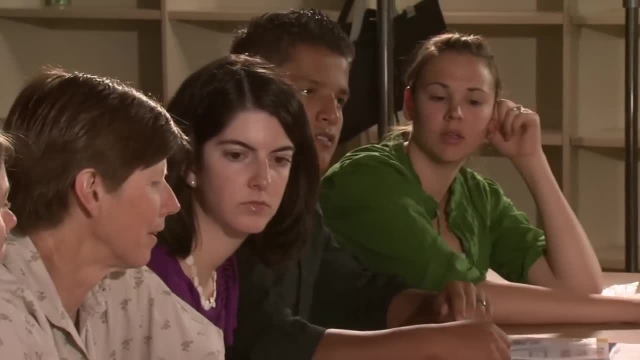 Is this what the child is doing? Oh, Or is it what the parent is doing? Gosh, I like this discussion. Is this the child? Yeah, This would be the child. This would be a child. I kind of say that decoding would be here. 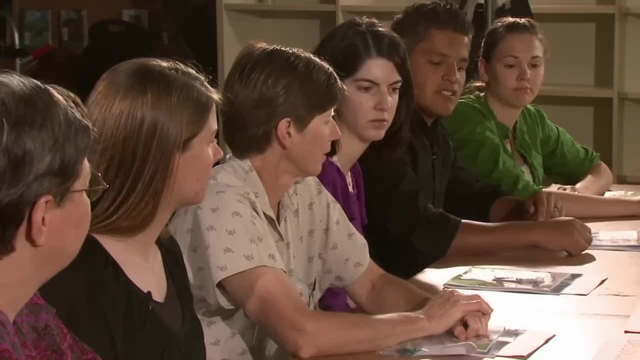 And I probably, you know, I've not given you enough definition of what each word means, so that could probably help. But I mean, like they can understand, like the story or something, before they're talking. Yeah, Yeah. 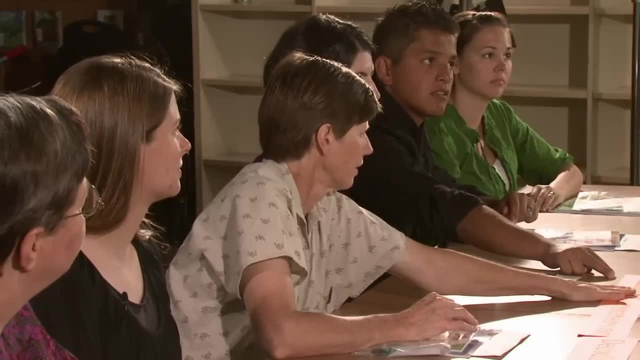 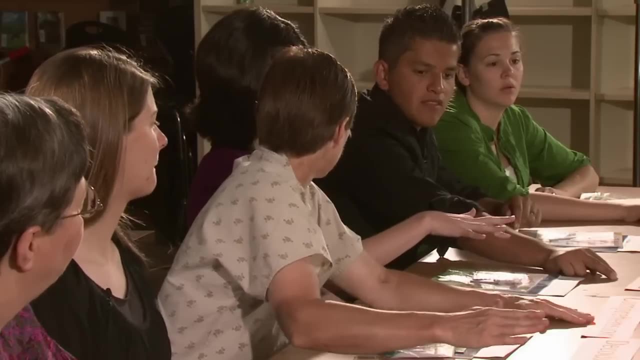 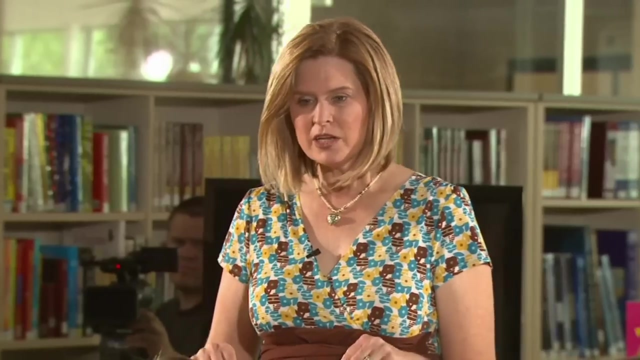 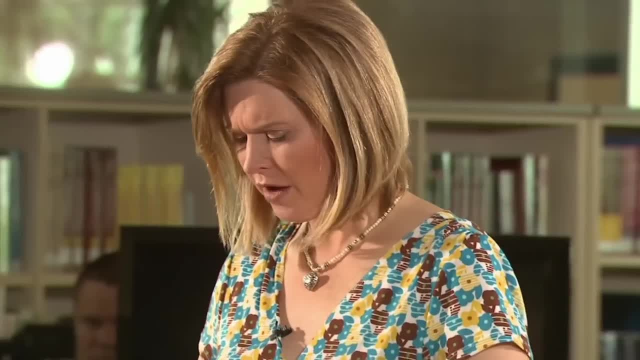 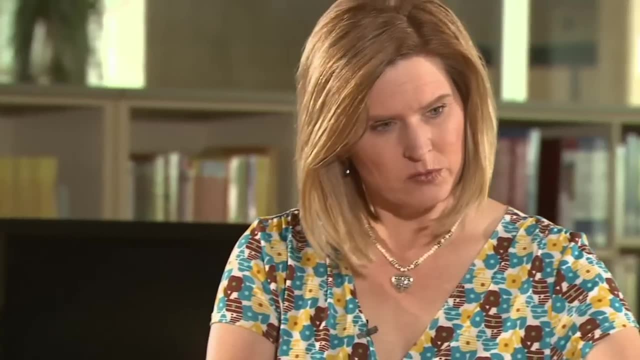 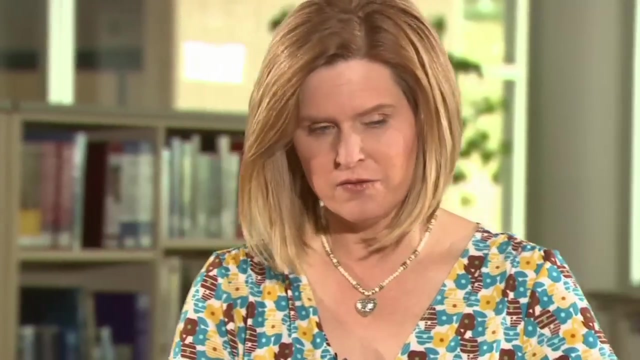 what does decoding really mean? What does decoding really mean? and well, you have to understand, because comprehension means understanding, And you would have to understand after each one, wouldn't you? And so, really, comprehension would be under each line. In our case, we're going to put it at the very end, but Nancy had a really good point. 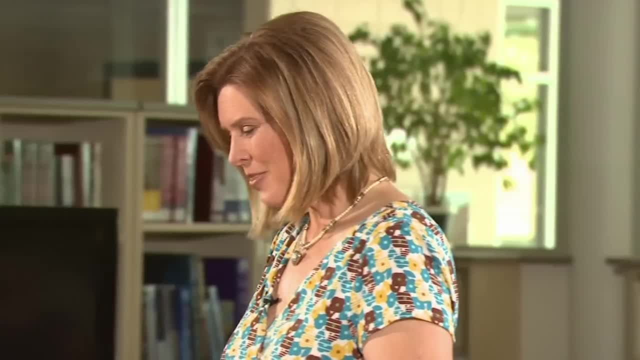 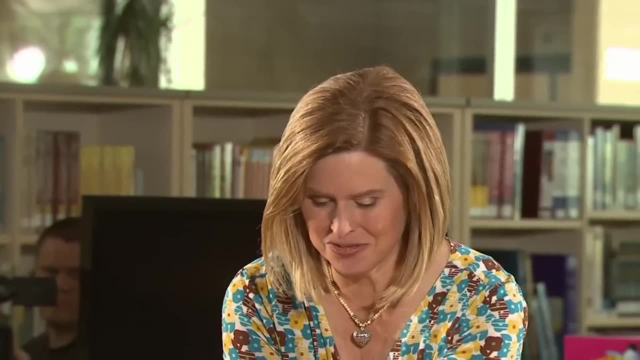 that you need to comprehend in each one. Now, having done that, you guys did a really good job. You've got listening, talking, and I'm just gonna switch these two: writing, decoding and then comprehension. Once again, remember what Nancy said, though. 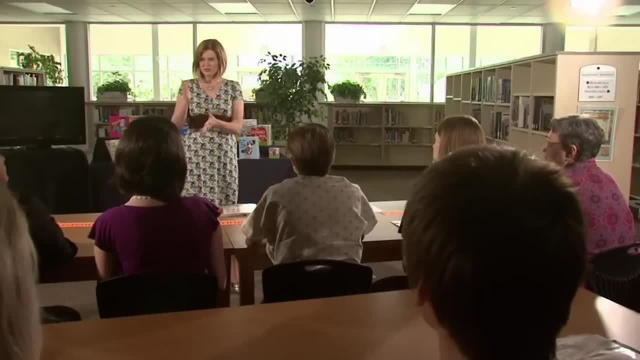 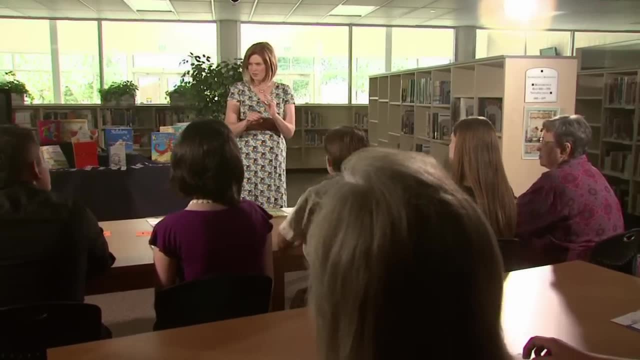 is, if a child understands what you're saying and then understands what he's saying, what he's writing, then decoding. Now a couple of you were like: well, what does decoding mean? Kasia was saying: well, what does that mean? 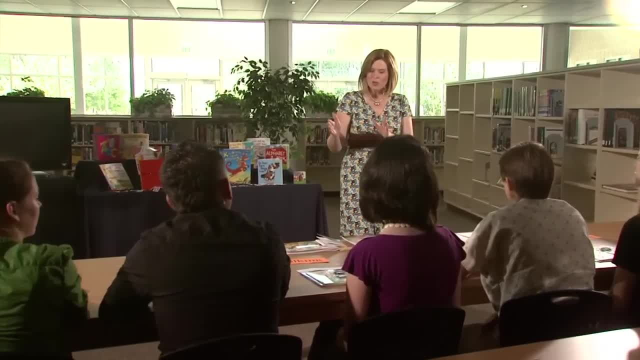 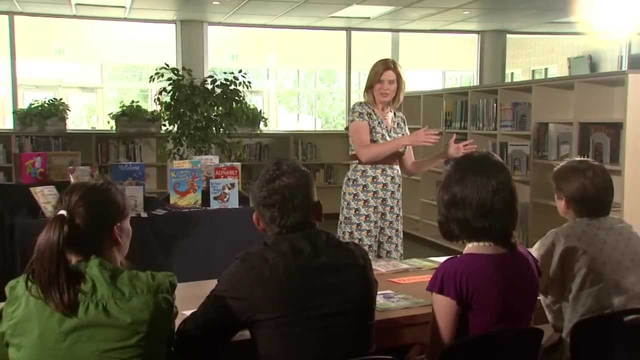 We need to find out, And so we're gonna talk about that right now. What does each one of these words mean, And how will that make my child actually learn to read one day? Because we're talking about emergent literacy skills. Everyone understood that listening. 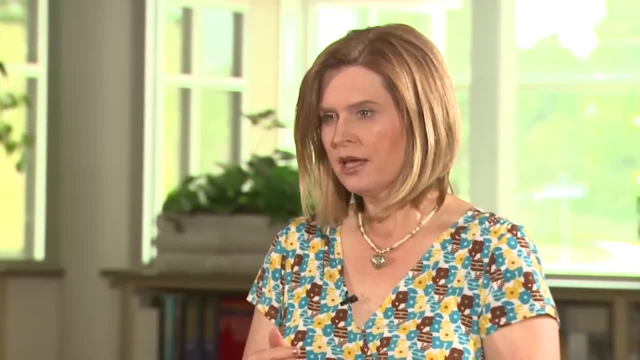 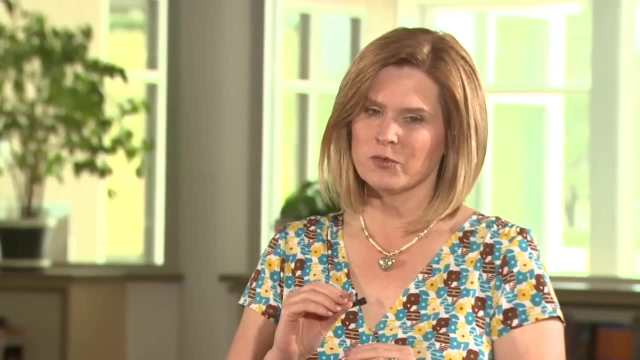 was the very first object in our emergent literacy skills And listening is very important. As we've talked about in nursery rhymes and storytelling and a lot of our other different workshops is listening. comprehension precedes reading comprehension. I just want to give you a study. 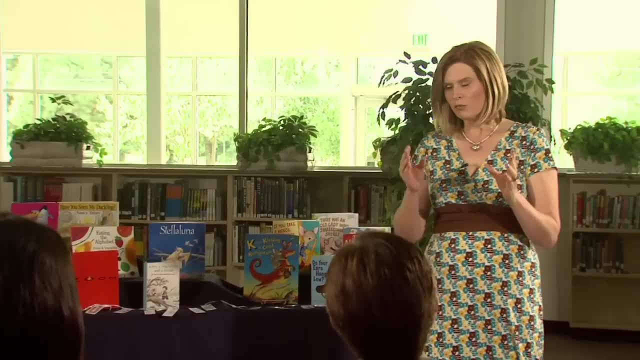 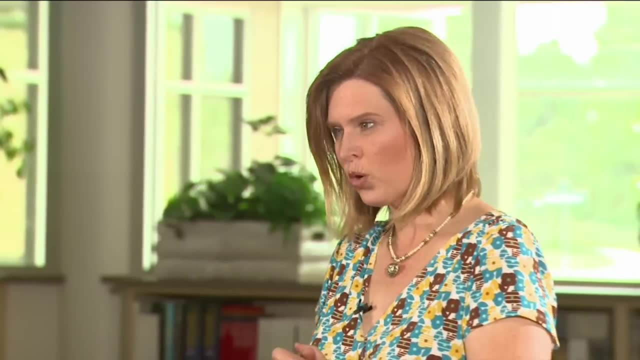 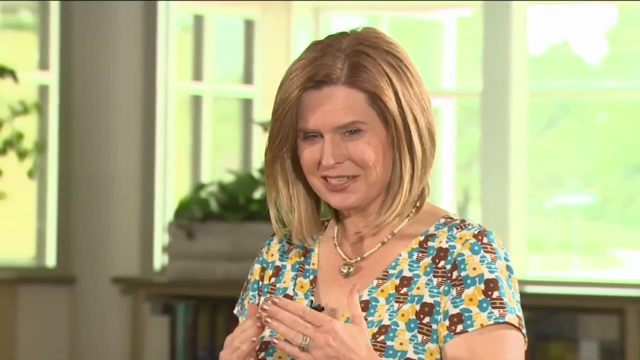 that the Department of Early Education conducted. that really cemented this to me as a parent. It talked about an 18-month-old child learns nine words a day. Nine words a day, an 18-month-old child, And so, as that child is learning nine words a day, 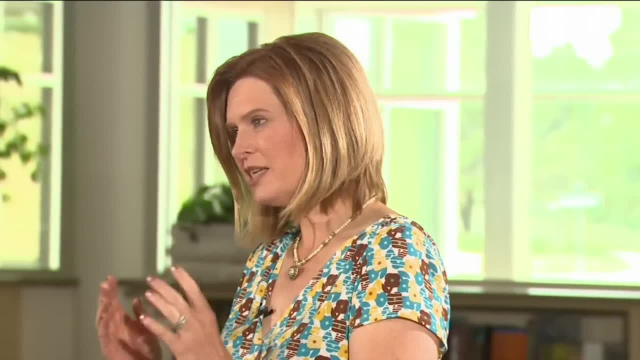 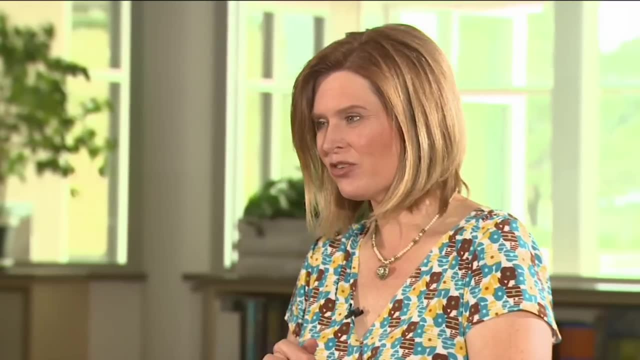 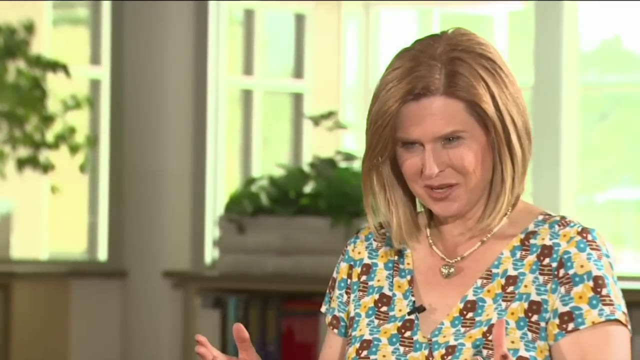 let's say, in a six-month amount of time. So that's about 180 days. If they're learning nine words a day, they're learning almost 1,700 words just in a six-month amount of time. Now, if you have or know an 18-month-old, 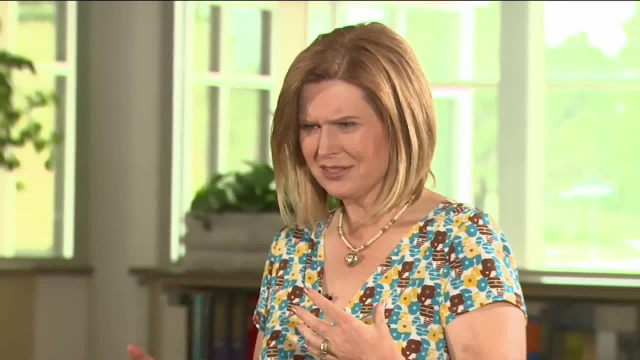 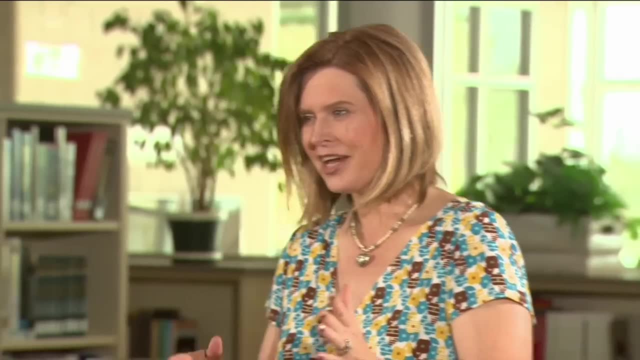 how many words do they speak? Can they speak 2,000 words? No, But, as Nancy said, they can comprehend that, They understand that. And I have a granddaughter. I have four grandchildren And my one granddaughter is in this stage, right now. 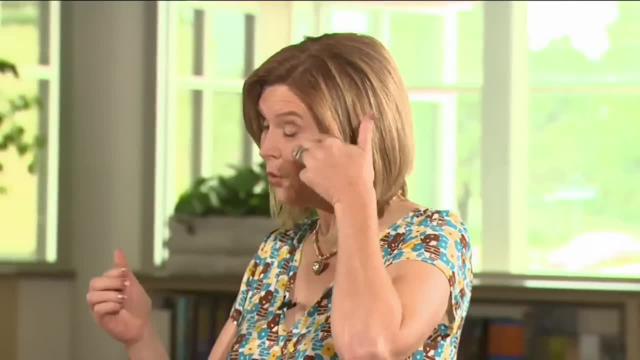 And we can talk to her and I can say: where are your eyes? And she points at him And then she points us right in the eyeball: Where's your shoes? We're going to go to the park. What are we going to do? 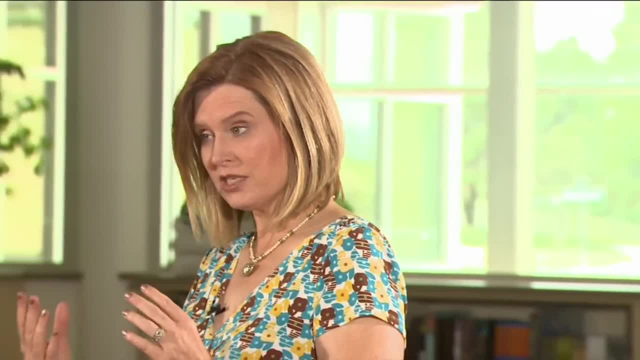 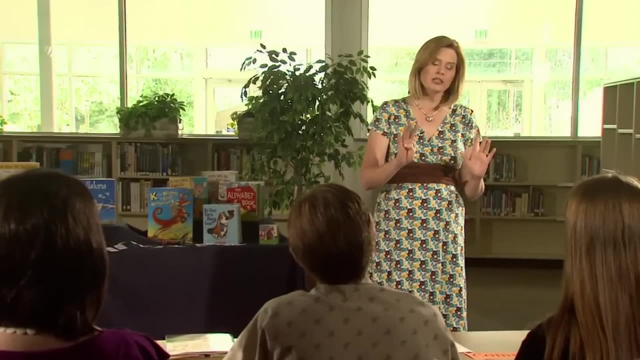 And she knows exactly what we're going to do, although she can't always say all those words. Now remember, those nine words a day come from a parent that talks to their child like they're going to talk back. That would really surprise you if your child 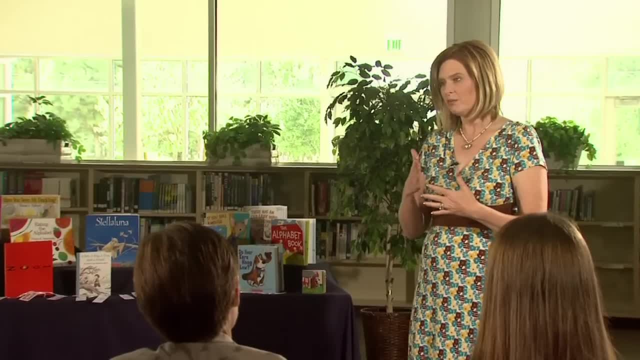 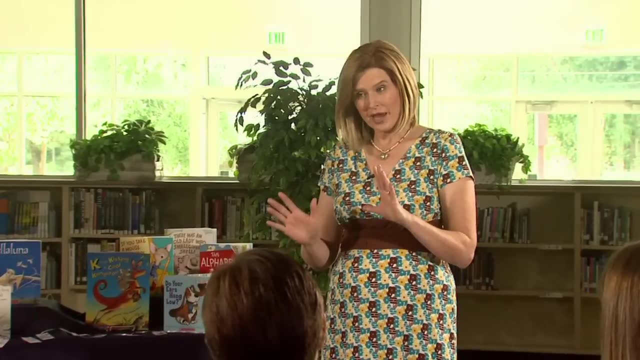 started talking back, But that's what we call conversation mode. Now a third of the children in the United States are talked to in what we call command. Now, as a parent, I do this myself, But I try to talk in both. 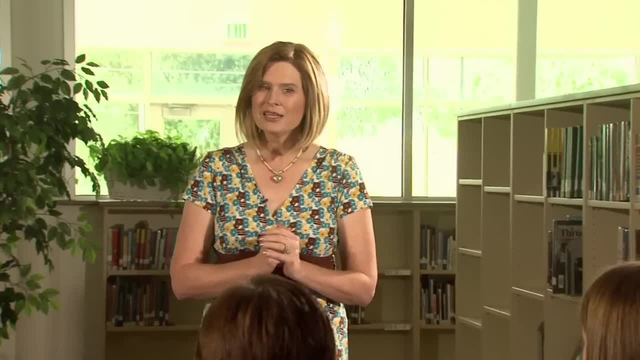 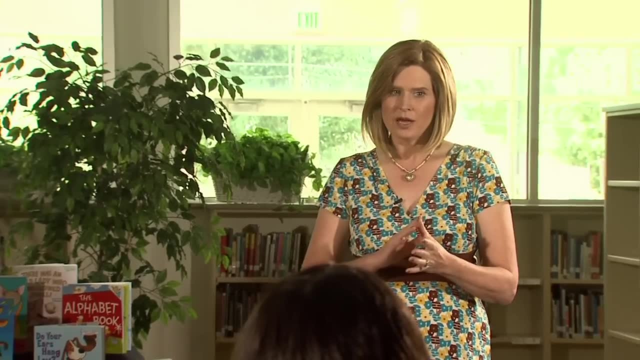 But for the most part we need to stay in conversation. Command is: don't hit your sister, Turn off your telephone, Eat your dinner, Brush your teeth, Go to bed. Can you imagine that some children only hear that over and over and over? 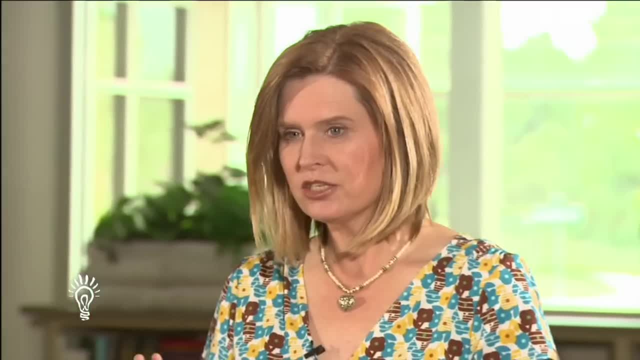 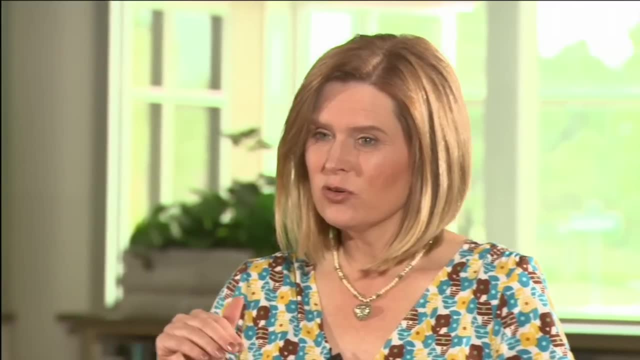 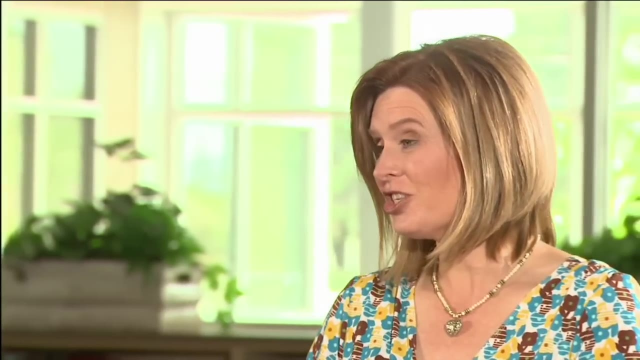 They never hear that conversation mode. That child is only learning three words. That child is only learning three words a day versus the nine words a day, And so they actually start school at a deficit because their vocabulary and their comprehension is less than the child that is just talked to. 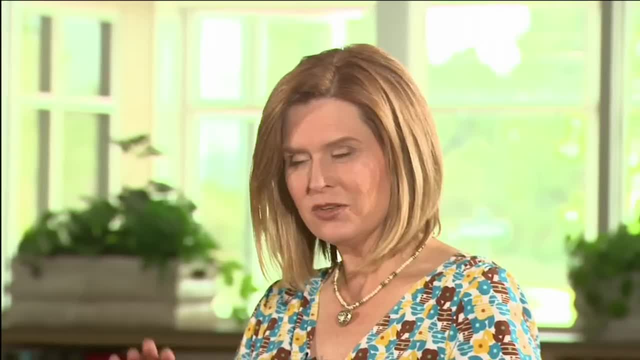 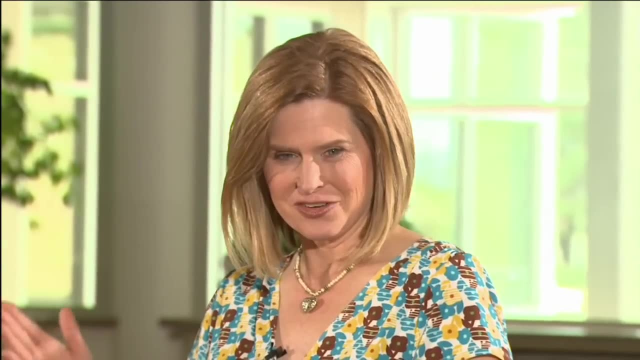 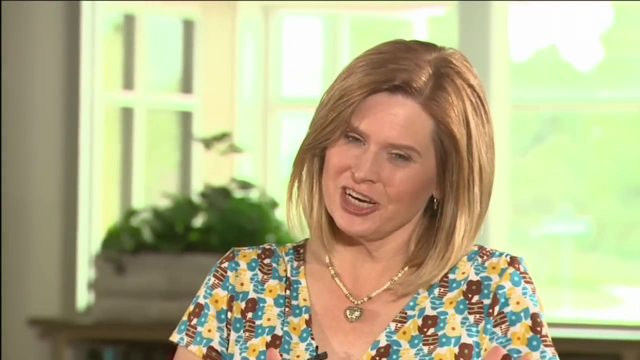 Along this study, it said that mothers that continue their education after high school that their children learn 12 words a day, versus the nine or the three. The higher or the more educated a parent is, the more vocabulary a child will have. Why would you think that, Sharon? 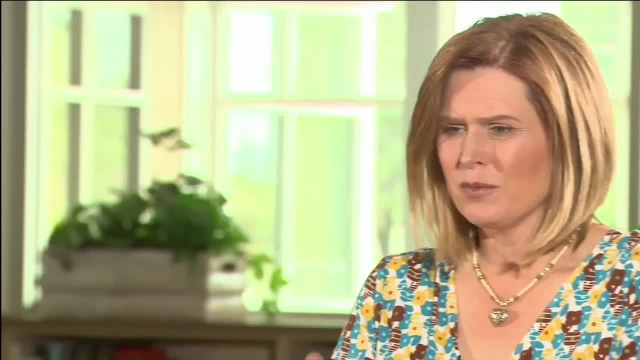 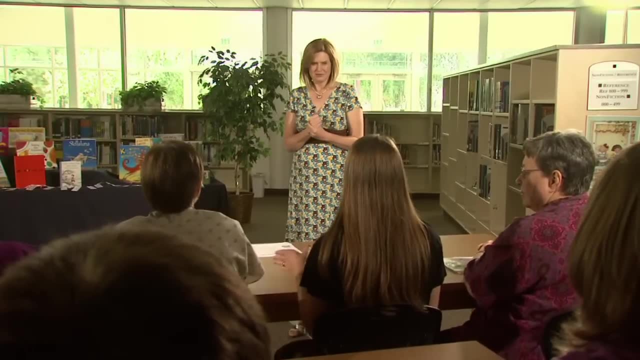 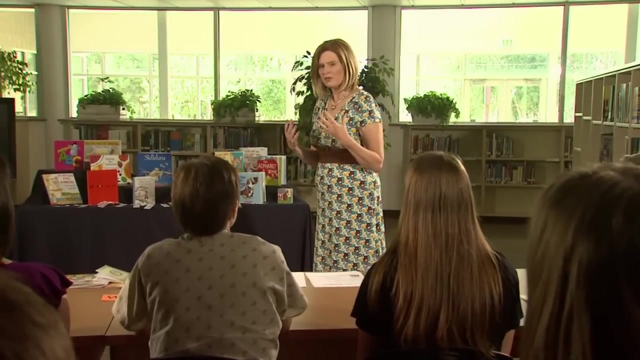 that a child would actually have a bigger vocabulary just because of the mother's or the father's education, Because they build upon their mother or father's education And that gives them a step up to even build upon that. OK, And as a mother- myself and every mother, 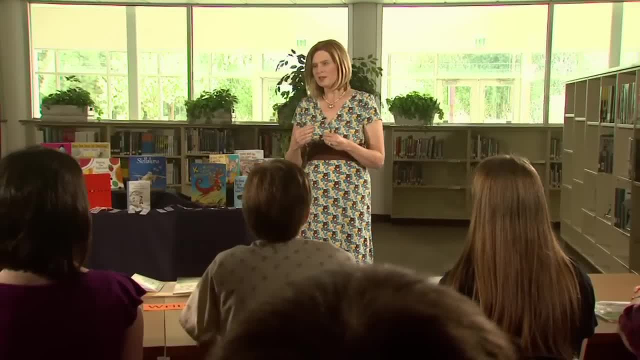 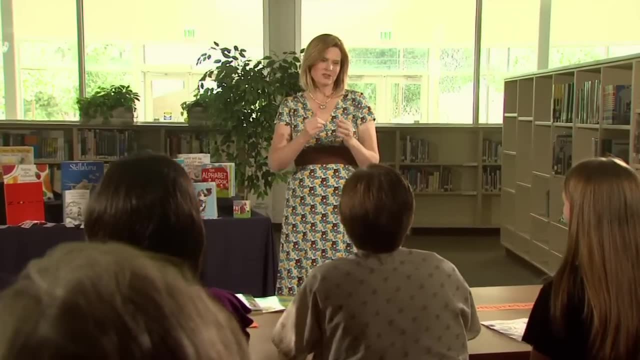 that I've ever worked with, or every parent that I've worked with, said I want better for my children than I had myself, And so the more that we know, the more that we can pass along to our children, And so education is a key component. 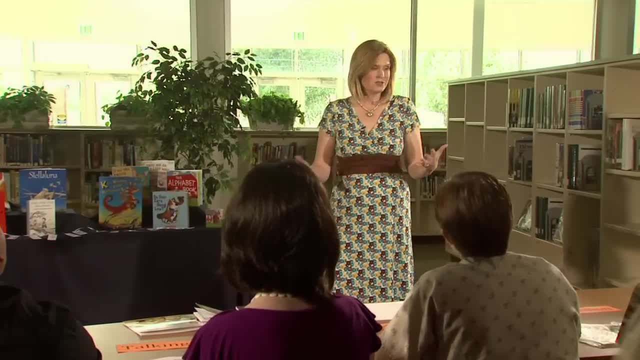 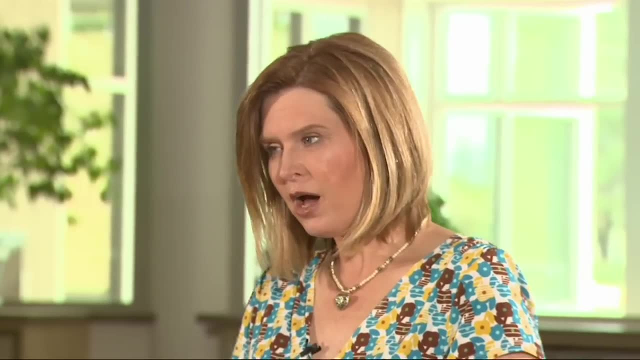 in helping your children. Now, some of us can't always go to school, but we can continue to educate ourselves. There's lots of ways you can continue to educate yourself, And so how important is that. Just think of those words, the nine words versus three words. 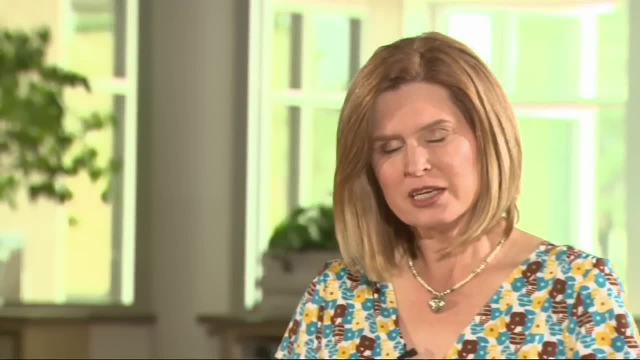 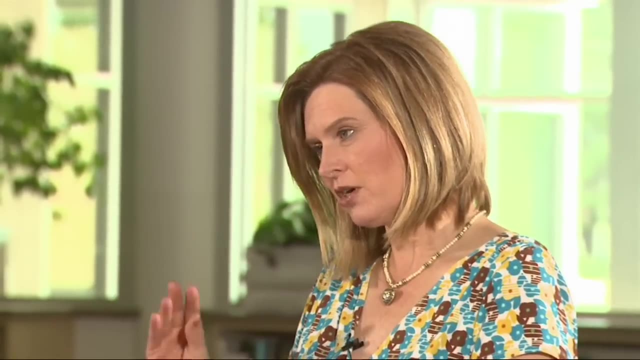 and 12 words. And a teacher gave me an interesting example one time. She said: you know, Not only does that affect their reasoning skills and their cognitive skills when they come to school, but it also is their social and emotional, Because the way they're talked to at home 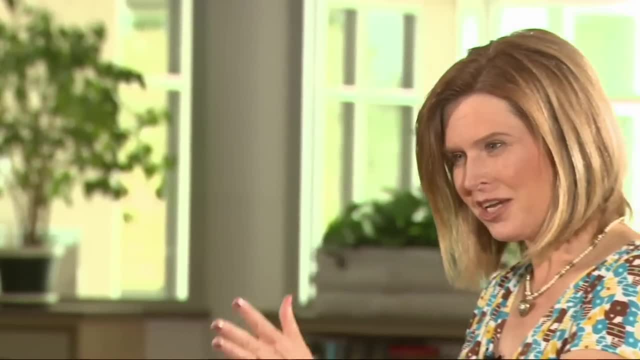 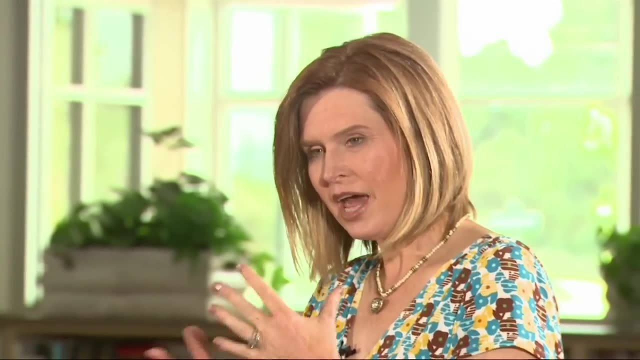 is the way that they talk to with their classmates, And so Erica, as a teacher, has probably seen this, where a child is usually commanding everyone to do things And what happens is then, as a social skill, children don't like to be around that child as much. 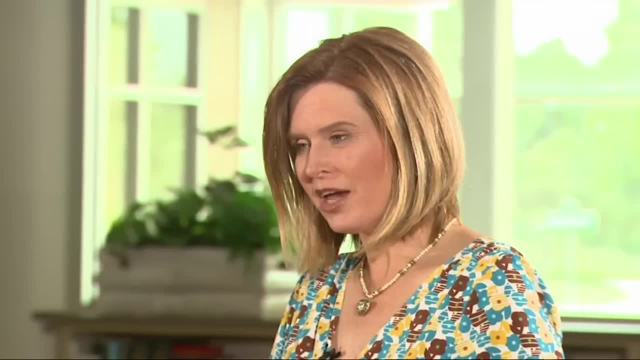 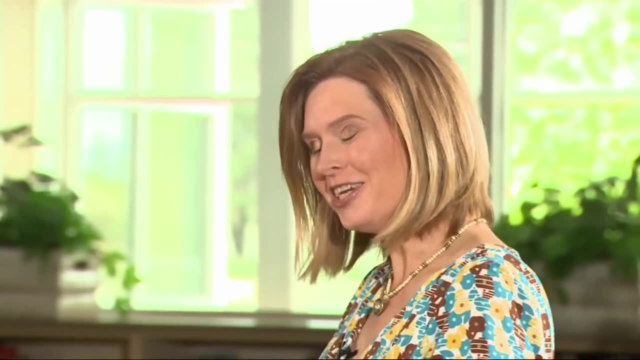 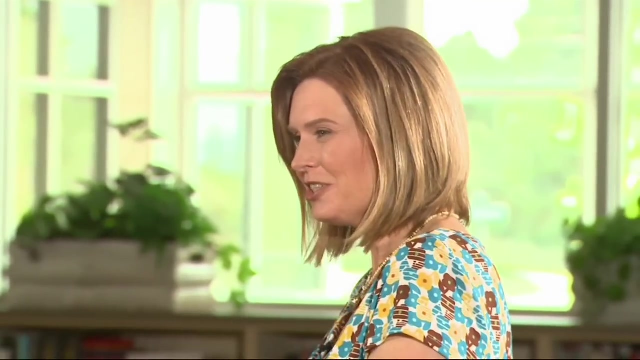 And so it really makes an all the way around effect in how that child interacts with other kids. In this clip I'm going to show you. it's a parent talking to their child with a lot of expression, a lot of gestures. but it's how we should be talking to our children. 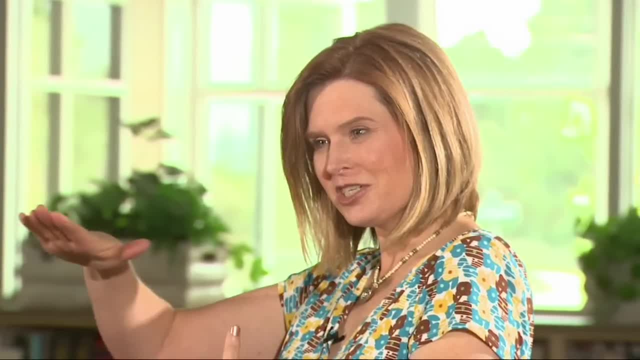 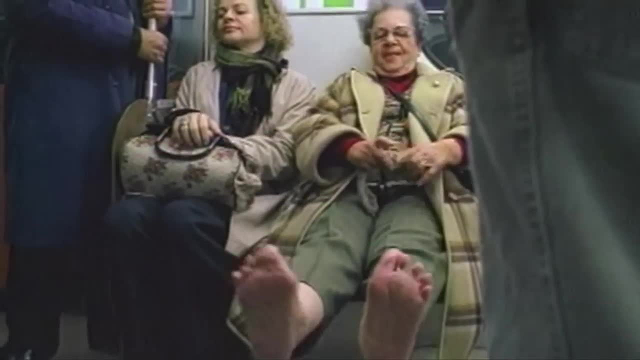 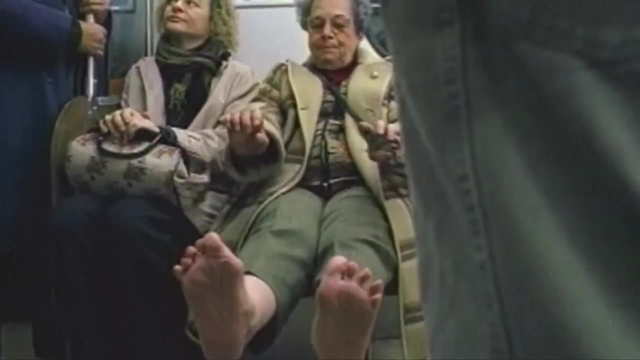 as babies, to set that foundation for them to learn to talk themselves: One, two, three, four, five, six, seven, eight, nine, 10, 10 little piggies ready to play, The big piggie's Pedro. 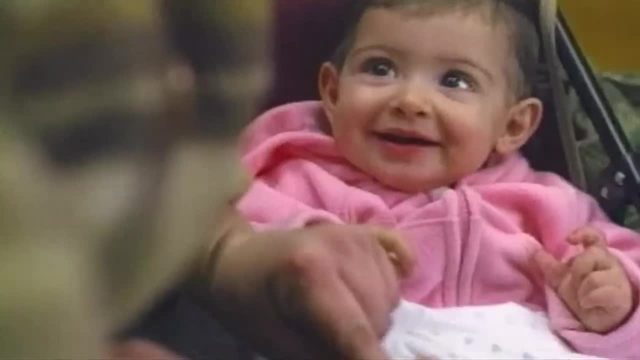 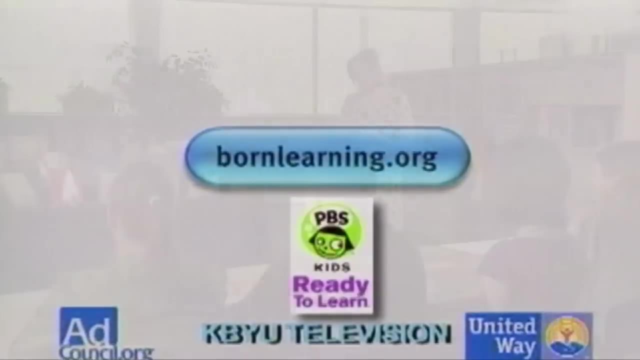 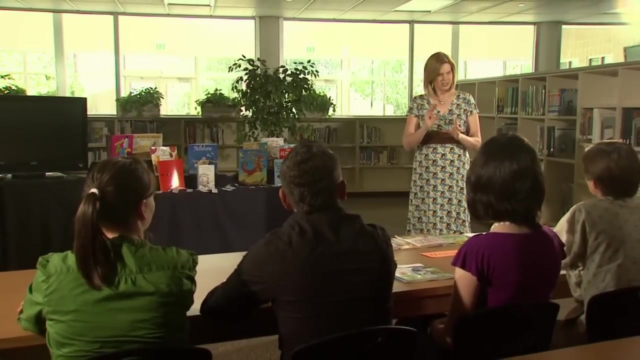 Pedro piggie, he's the big piggie. Everyday moments can become teaching moments, because learning starts long before school does. Give your child the start they need at bornlearningorg. Born Learning has great ideas for parents in this stage of what they can do with their children. 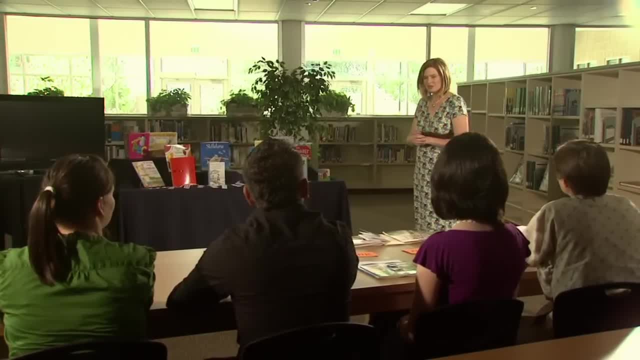 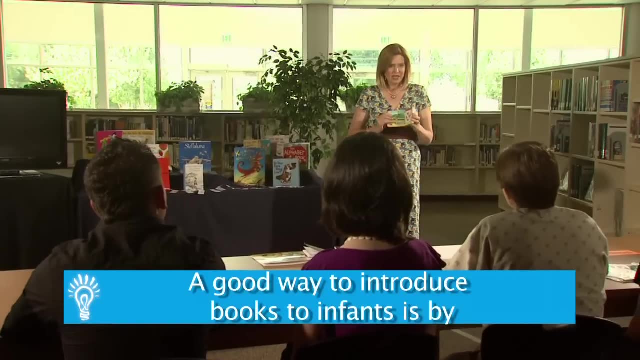 to help them eventually learn to read. Now, in this stage, what kind of books do we want? We want barn books. we want board books, where our children can chew on them, where they can handle them, where they're chunky and that they can turn the pages. 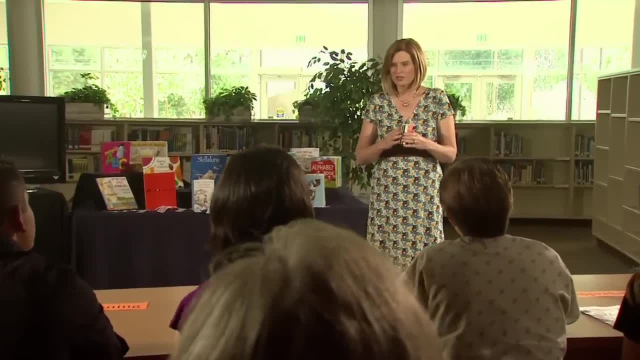 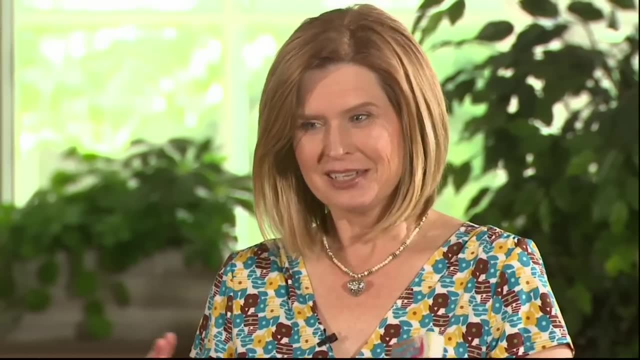 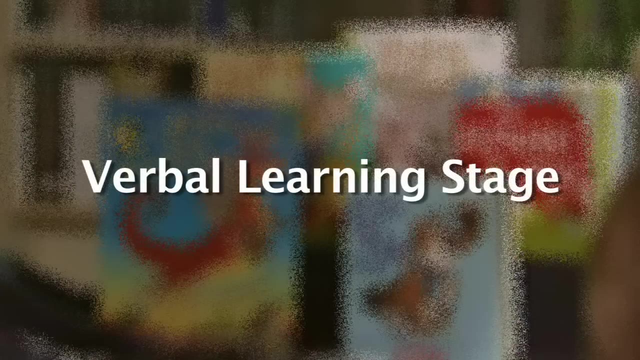 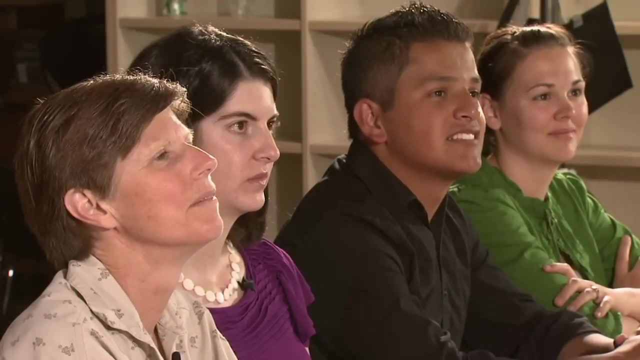 Don't worry as much about the words as just introducing the books. And the next topic we're going to talk about is talking. Children and talking goes hand in hand, doesn't it? If you've ever been around young children, you know they talk and talk, and talk. 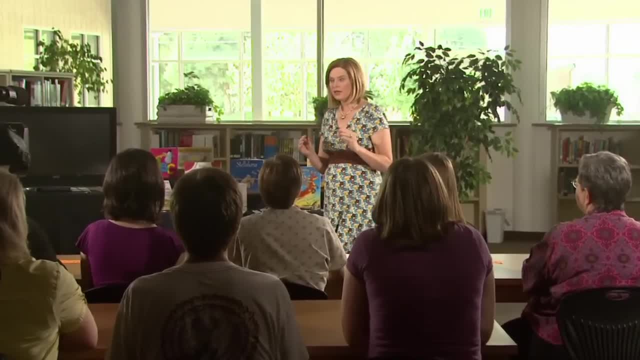 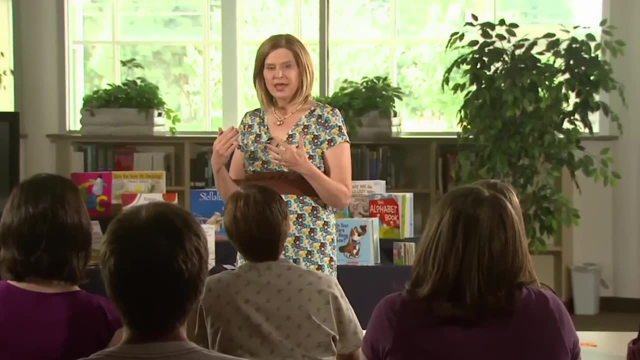 That is what we call the verbal learning stage. Children have to hear themselves talk to actually learn, And so it's very important for them in this stage to talk. I read in a professional journal once that when you ask a child to sit down and be quiet before the age of six, 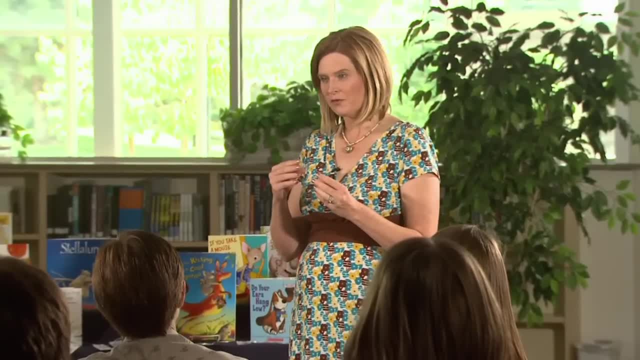 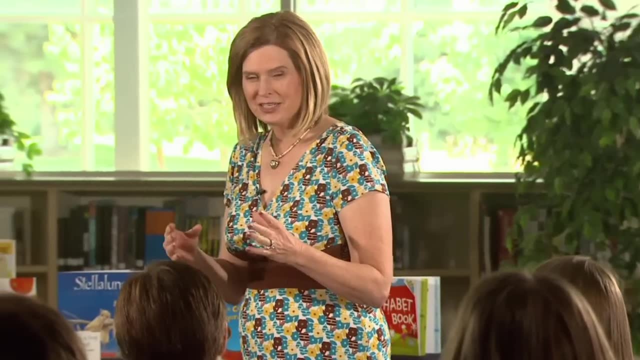 it's like asking them to sit down and not think. Now, having taught preschool, I've learned that when you ask a child to sit down and be quiet before the age of six, I do know that when you ask them to be quiet. 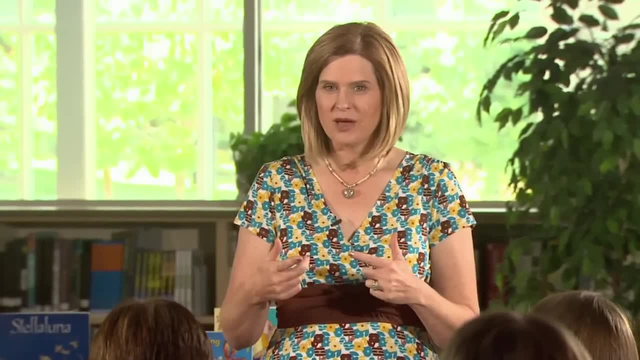 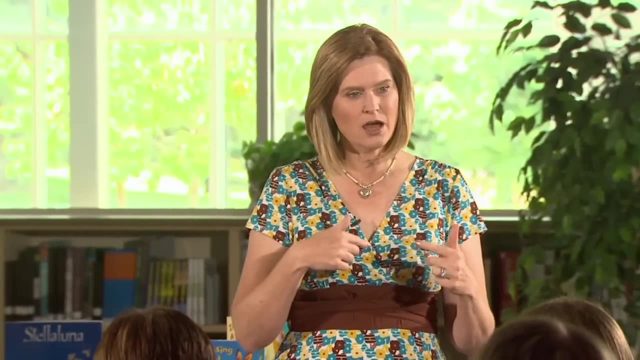 they're thinking, but they're not thinking about what you're saying. They're thinking about: hey, my mom said, or teacher, he's doing. but what we can do is the more that they can talk, the more they can learn. 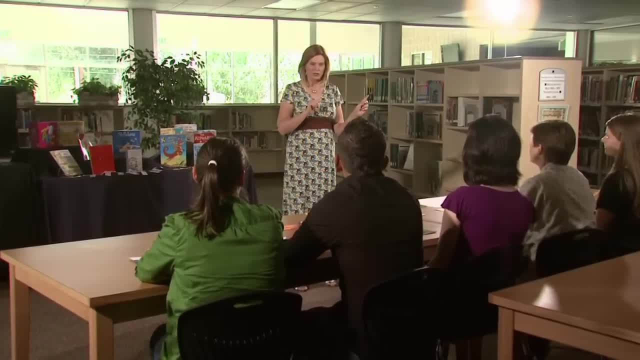 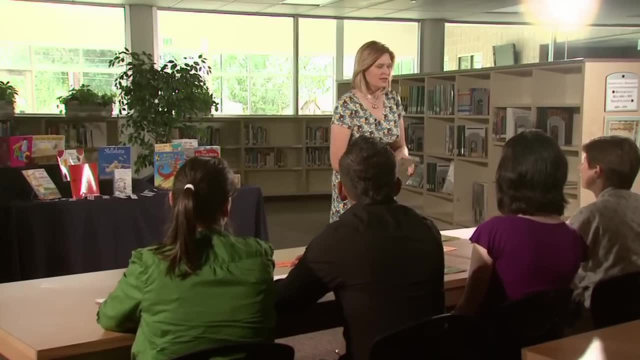 And so in this stage, where we call it a verbal learning, they need to be engaged, They need to use a lot of books where they can talk. as you're reading Now, this book is a very old book, but it's a great book. 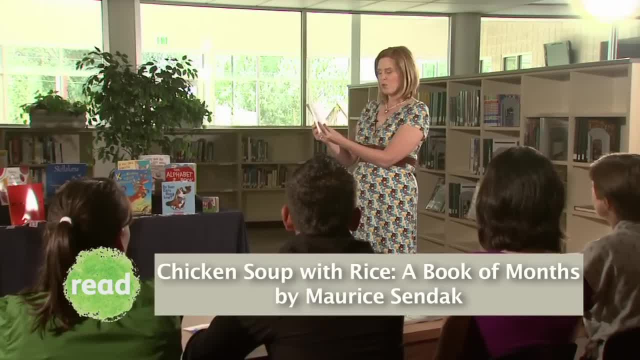 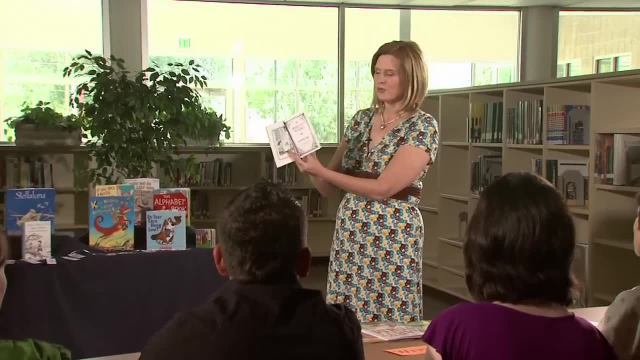 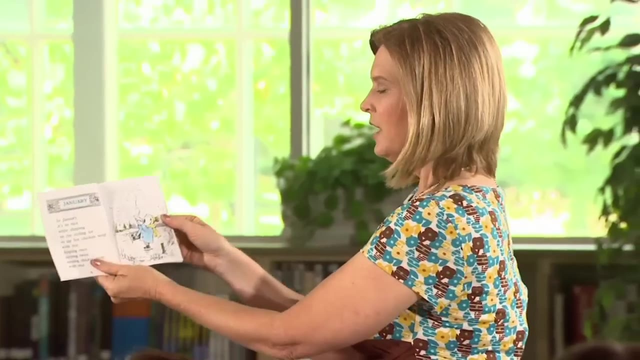 It's called Hot Chicken Soup with Rice, And I'm just gonna read a couple pages and you can see how a child can be talking or talking with you as you read this book. It's a book about the months actually. Oh, need to start with January. 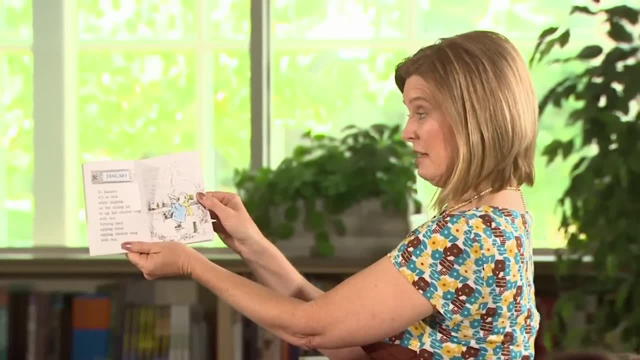 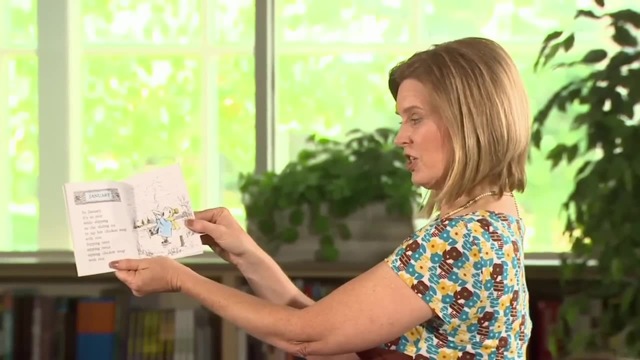 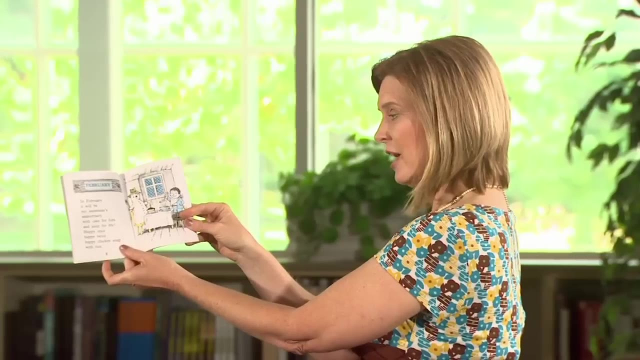 In January it's so nice, while slipping and sliding ice, to sip hot chicken soup with rice. Sipping once, sipping twice, sipping chicken soup with rice. In February, it will be my snowman's anniversary, with cake for him and hot soup for me. Happy once, happy twice. happy chicken soup with rice. See that repetition already In March. the wind blows down the door and spills my soup upon the floor. It laps it up and roars for more. Blowing once, blowing twice. 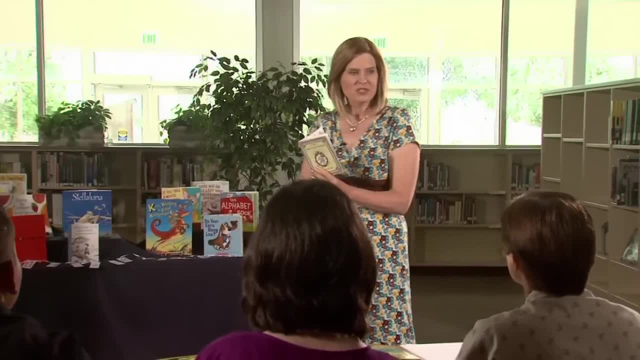 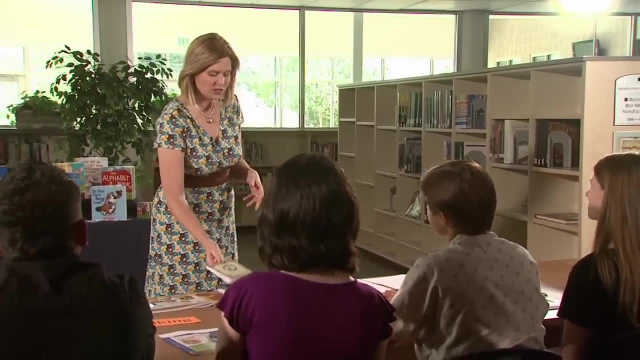 blowing chicken soup with rice. That kind of repetition for a child where they'll also be able to talk. a lot of rhyming books- I love Dr Seuss books because a child can actually read before they know how to decode the words. 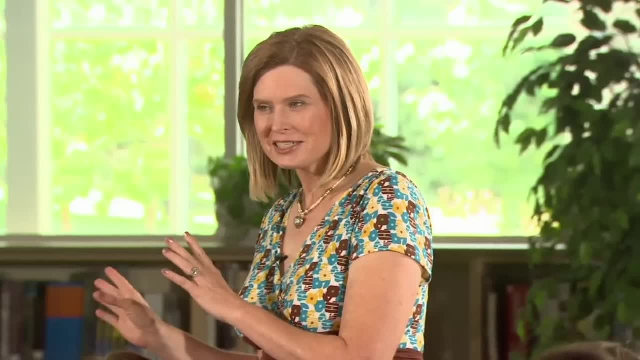 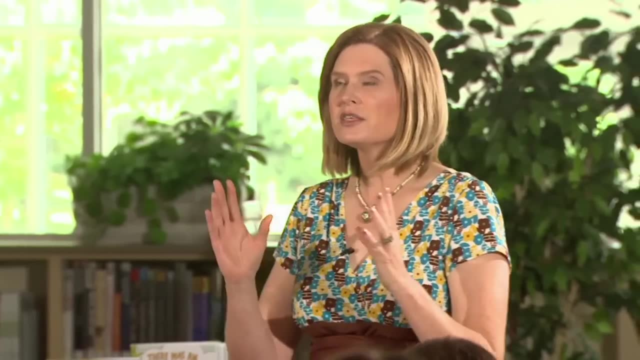 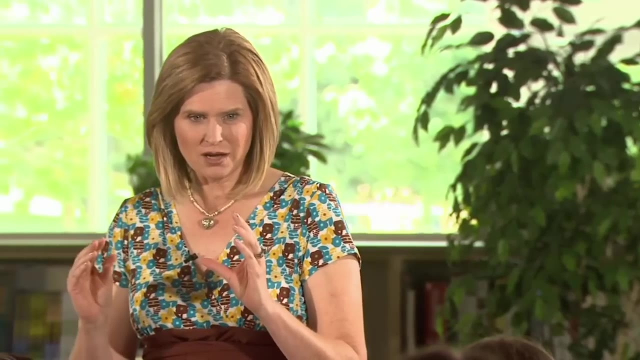 but they can repeat them as you go along. Now, this next clip is about a particular dog that lapped up some alphabet soup and all of a sudden he could do something that no other dog could do. Remember when your children talk and talk and talk and talk. 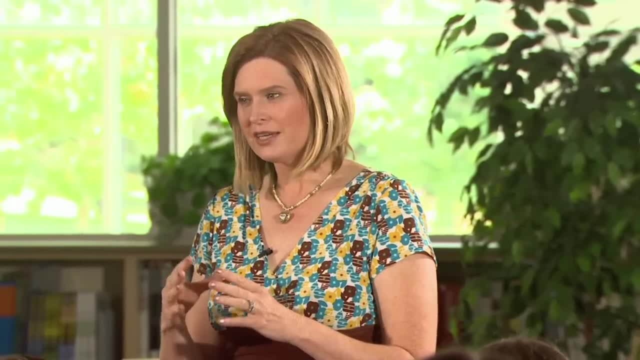 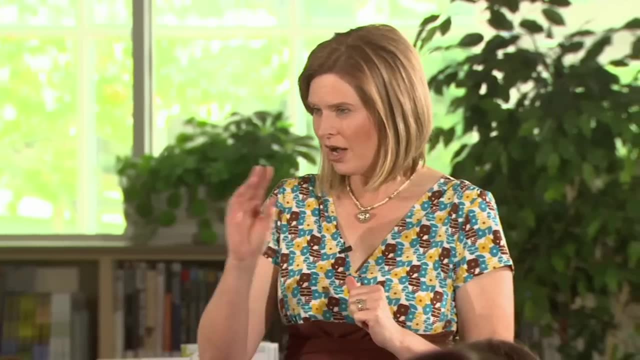 that they're learning, Encourage them to talk. I always say to parents: you might have a headache by the time you go to bed if you have more than one child in this stage, but they're actually talking and learning and encourage that. 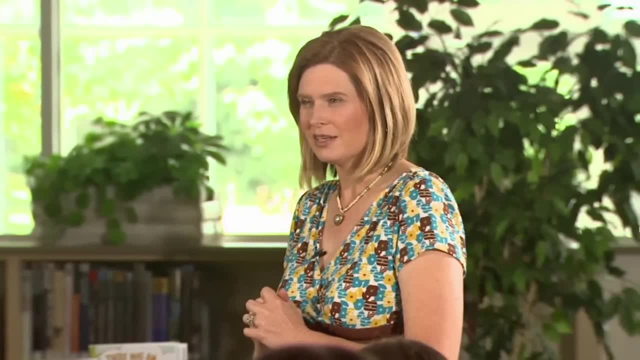 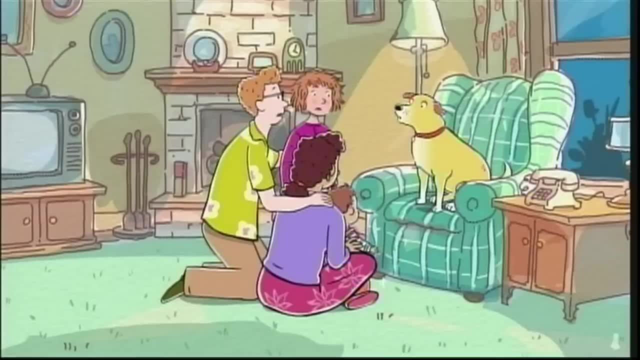 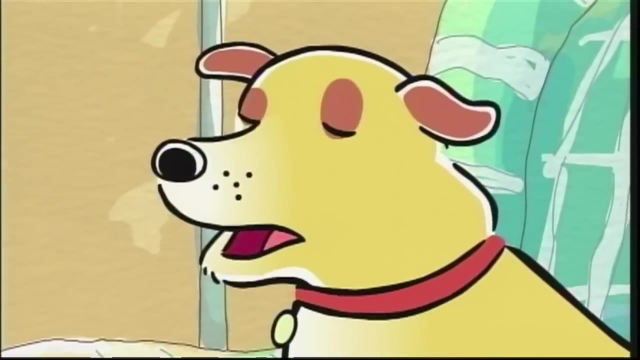 So let's show this clip about a particular dog that can do something no other dog can do. Have you always understood what we people were saying? You bet, and what dogs are saying too. How come you can suddenly speak? Hmm, Must be the alphabet. 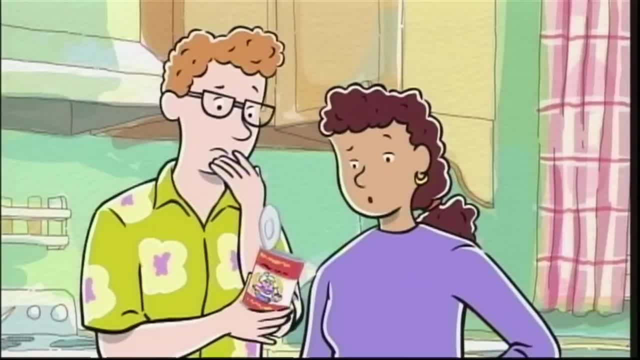 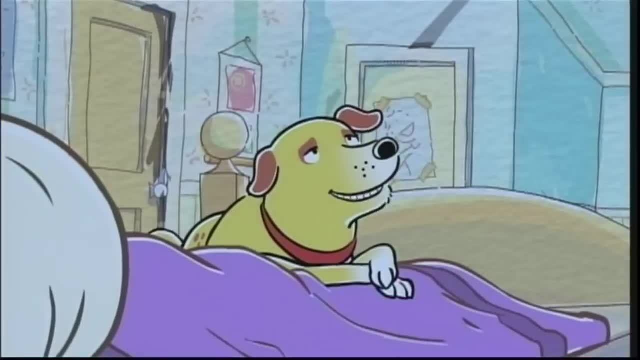 It's soup. A giant reptile did it. Ah, There's a poodle over on Circuit Street I'd really like to play with. I'm sure you're curious about the early days of my life. Let me tell you something about it. 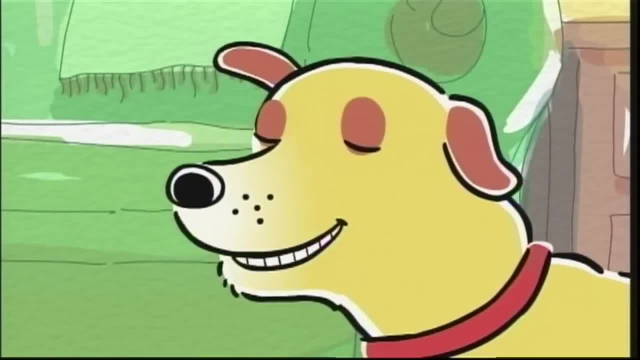 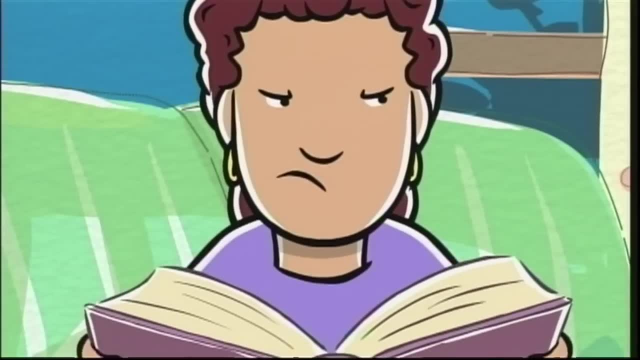 I was born in a back alley. I understand cat, but I can't speak. It's a nasal language. a lot of mama would tell us: You're dogs, not cat kibble. I really, I prefer soup Like here, boy, and I'm like hello, I'm a girl. 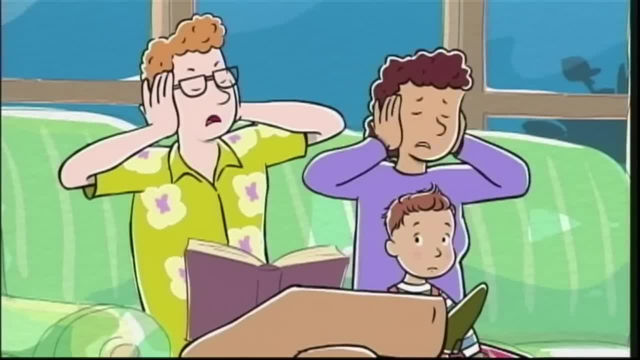 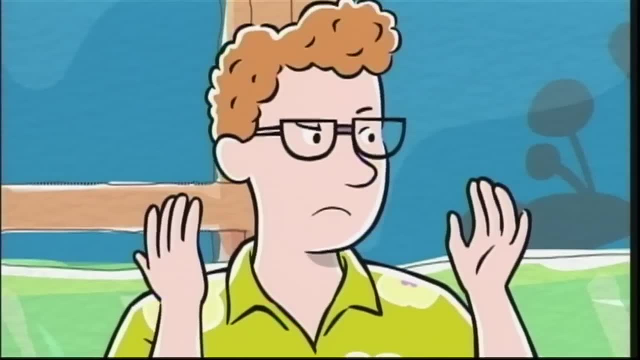 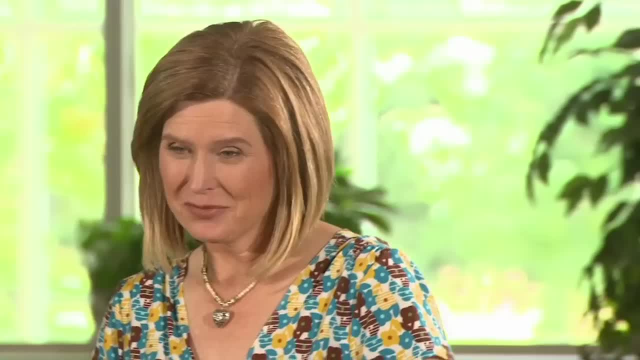 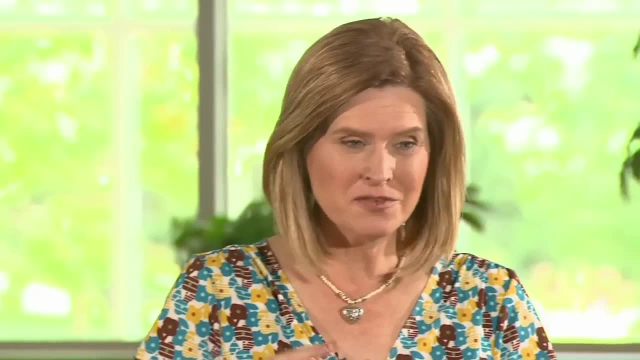 I don't know if any of you have felt like that. I know my older kids. with their little sister, they we would be watching a movie and she would need to be narrating or making a comment. That's very normal. Children need to talk. 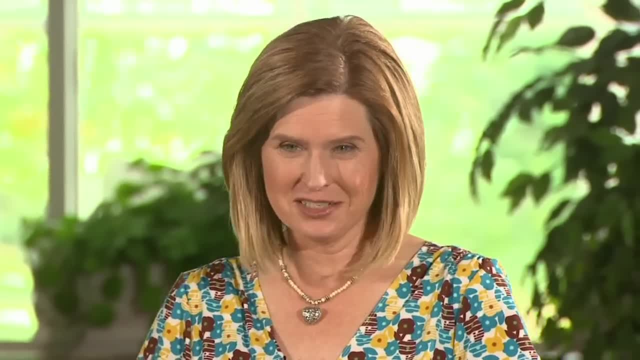 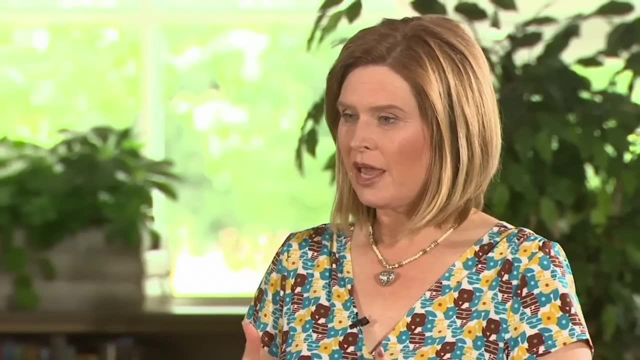 How many have children in the stage? Anyone has a child that's talking, talking, talking in the stage, Or a grandchild that's talking, talking in the stage. Remember that is normal and that as they talk, that they can learn. 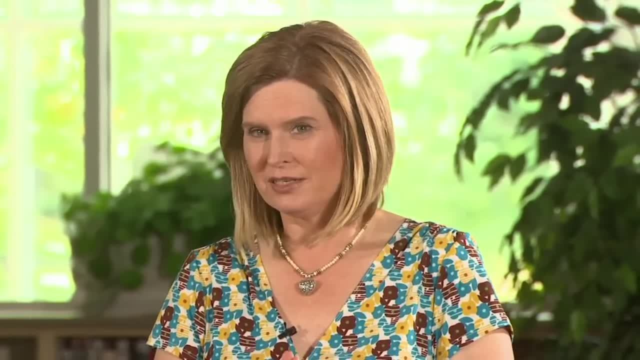 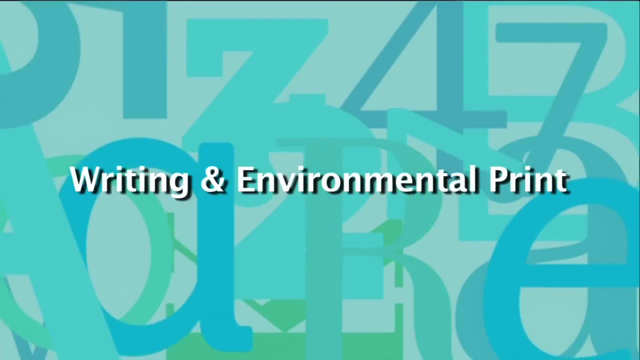 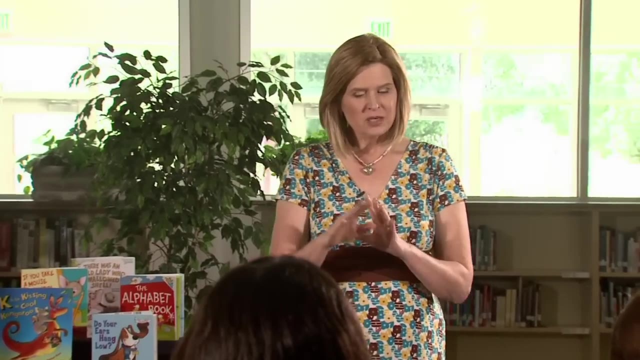 Find books that they can participate with you as you read. When I was asking you to put the emergent literacy skills in order, you know you mixed up writing and decoding And I didn't give you enough information, so I'm going to. 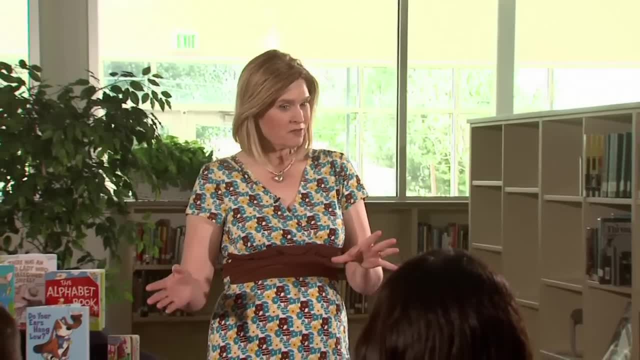 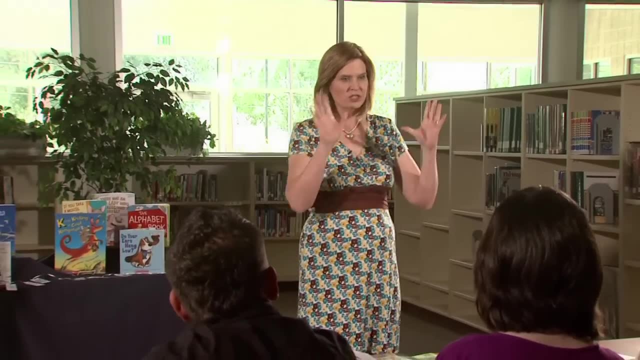 back up and give you some information. So I'm sure if you did this afterwards you would understand why writing actually comes before decoding. When we talk about writing, children start out with pictures or symbols And sometimes we think of writing as just writing letters and words. 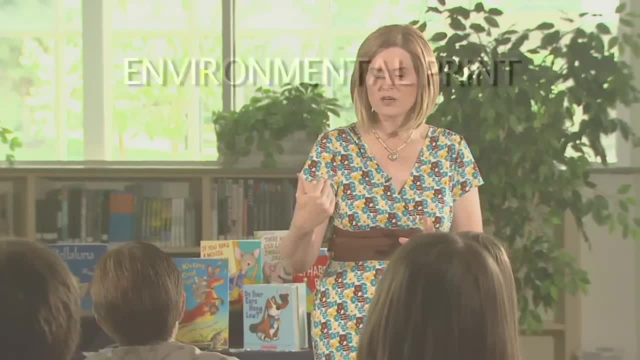 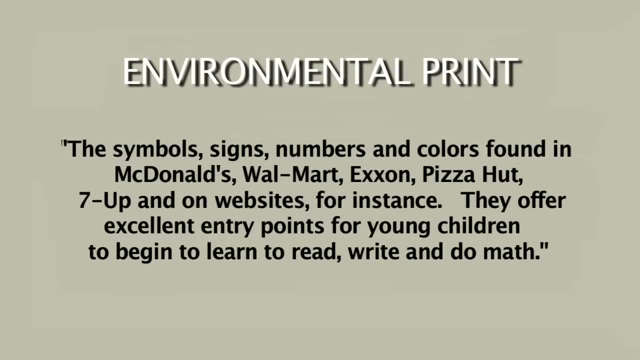 but actually the pictures come first And we that's what we call environmental print. And as you go about your days, you see environmental print that just comes very naturally and normally And you don't always, just you know, separate that. 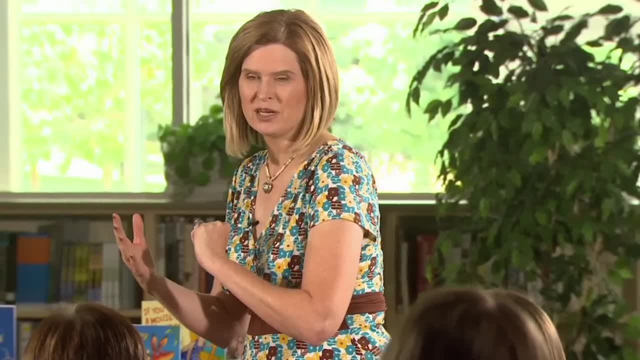 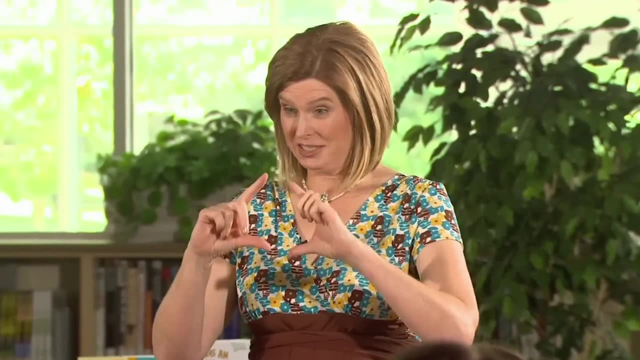 But if I'm walking into the ladies' restroom- especially when I'm in a different type of restaurant that might have a different way of saying women or ladies- I look for the symbol, to make sure there's a skirt there before I walk in. 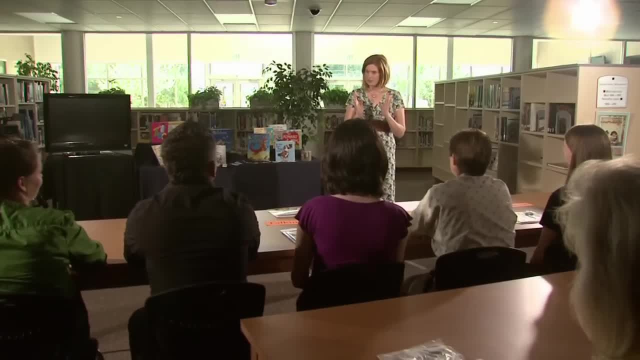 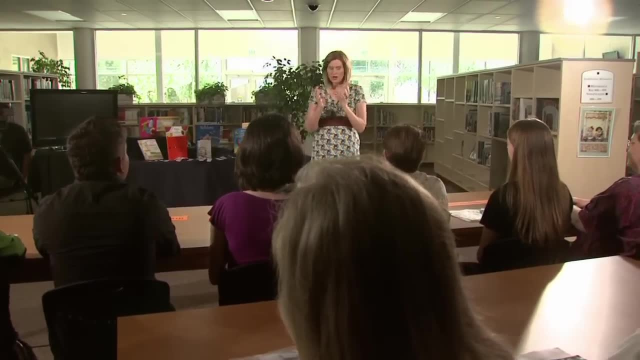 That's environmental print. A stop sign is environmental print. It says something. It's not always just the word S-T-O-P, It's the whole sign that has meaning. What does heart mean, Nancy? what does heart mean Generally- love. 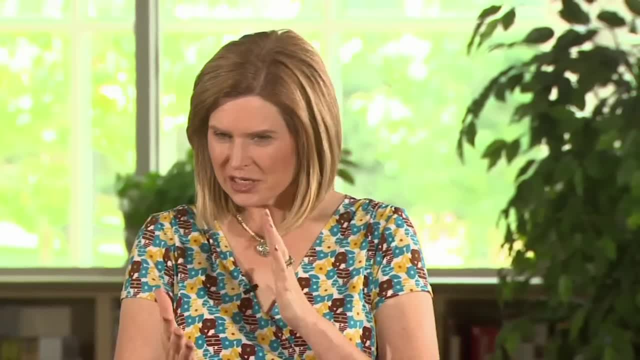 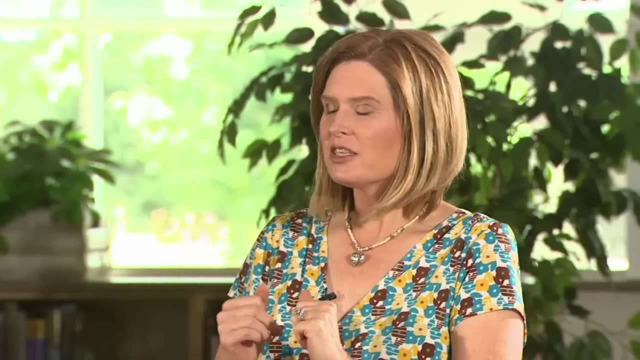 Love. Okay, So generally love. Candace, can you- I'm putting you on the spot- Can you think of any environmental print that children might see that they know the meaning as they're driving by a particular something? Can you think of something as they're driving? 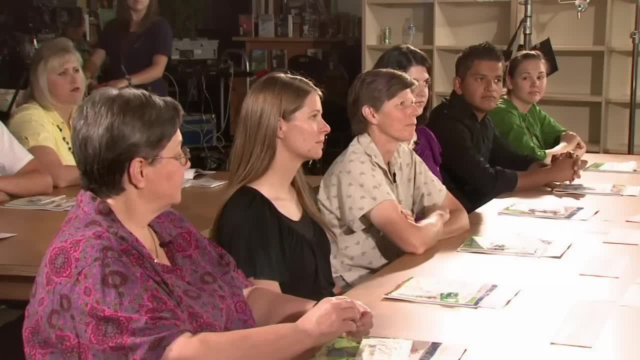 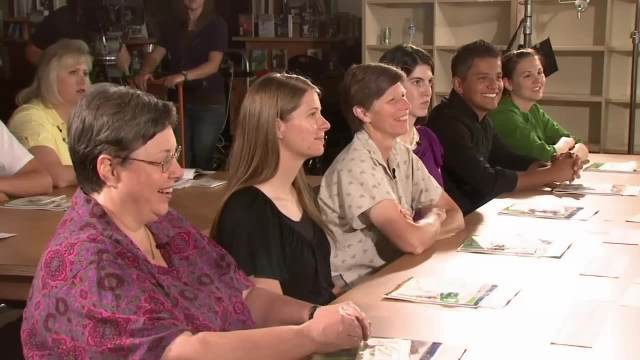 that they might see. that's environmental print. I'm putting you on the spot here. I think of golden arches. Okay, I know that there were some times that my daughter would go to the store and say my daughter would see those. 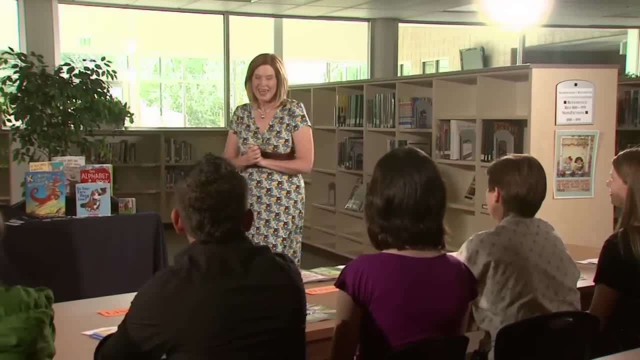 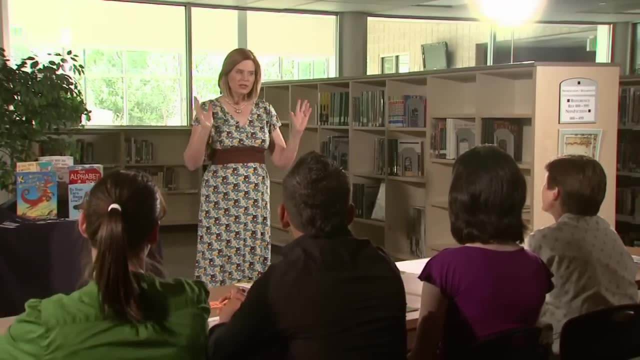 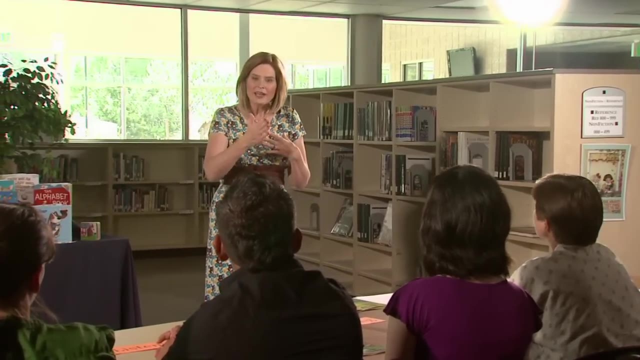 Did not know how to read but would want to stop. Okay, And so, as you're going through your life- that's the first part of writing- is environmental print? Please find lots of books that have that. Lots of bright pictures, Lots of pictures where children can go. 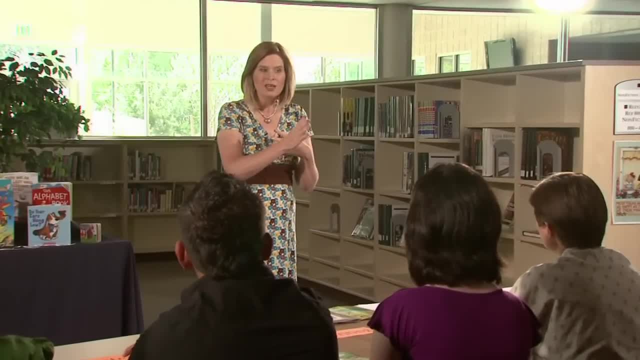 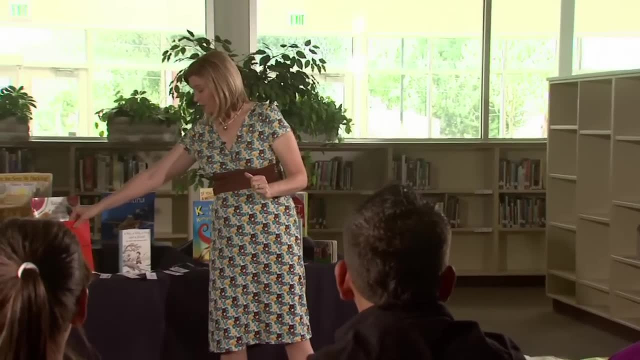 what happened first, What happened next, What's going to happen? Let them use the pictures. I have a couple books that I want to share with you. that actually, and so it will be very hard to read, because there's no words. These are wordless books. 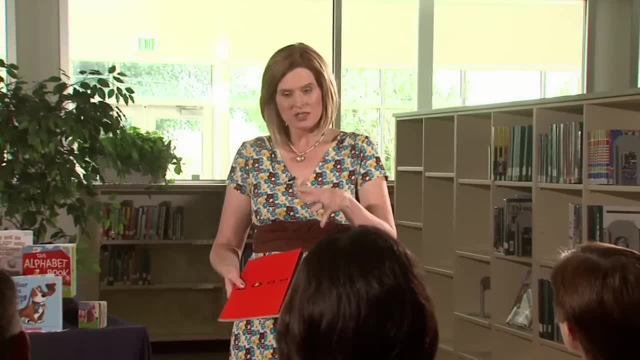 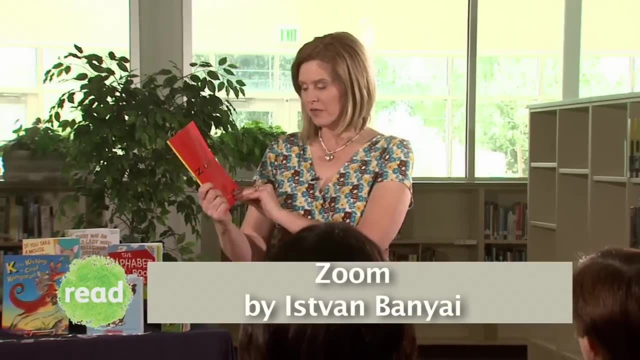 but they're great books for children that are in this stage, that quite don't know how to read yet, but they can look at a picture and tell you a story. When I first saw this title of this book by Zoom, I thought it was about zooming around. 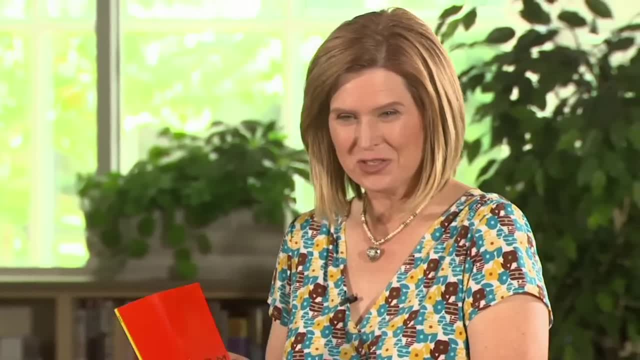 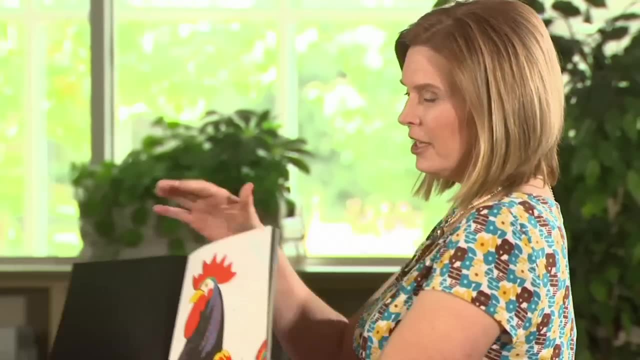 having three boys that were always moving, I thought it was about zooming around, but when I got it I realized it wasn't about zooming. It was about a perspective. Each page you see a picture and then they actually show you. 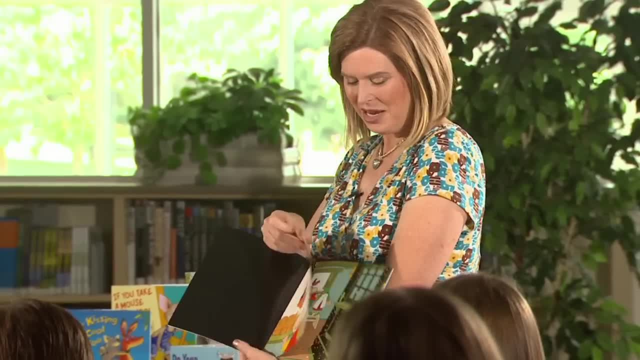 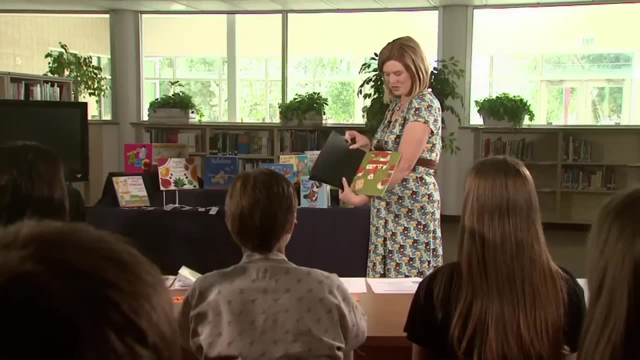 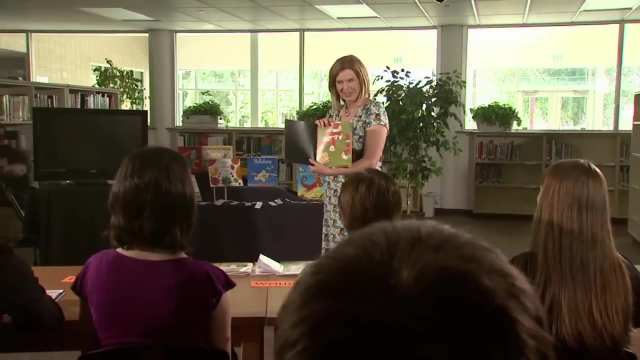 from a different perspective. Each page shows you more and more of the picture. until you see a different perspective, You can tell a different story. There's another book in this series called ReZoom, also that it takes that It just keeps going down and showing, and showing. 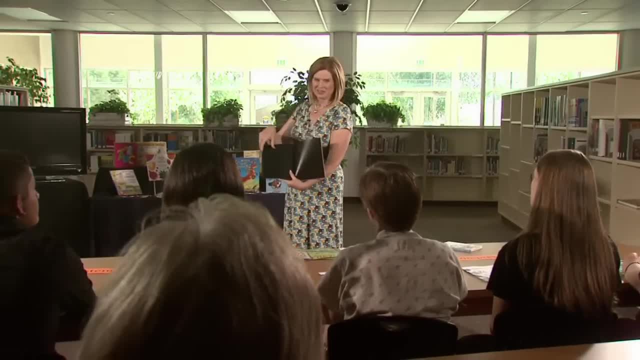 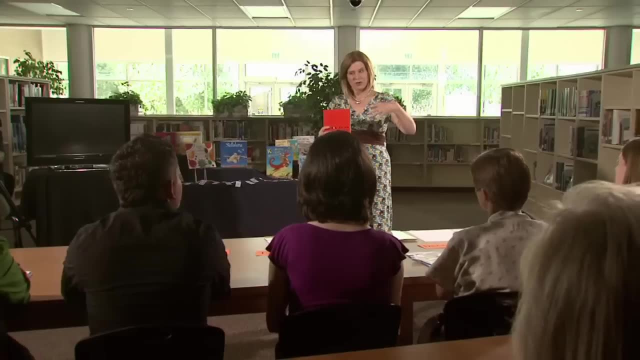 and then it takes that. Then at the very end you get to a small dot. It's a really fun book too. A child can read it to you, whether or not they can read or not. Another one is A Boy, A Dog, A Frog and A Friend. 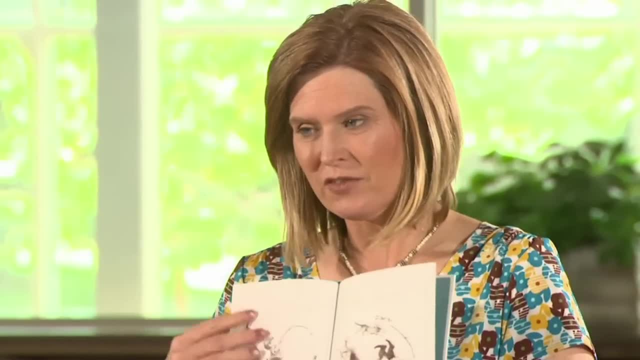 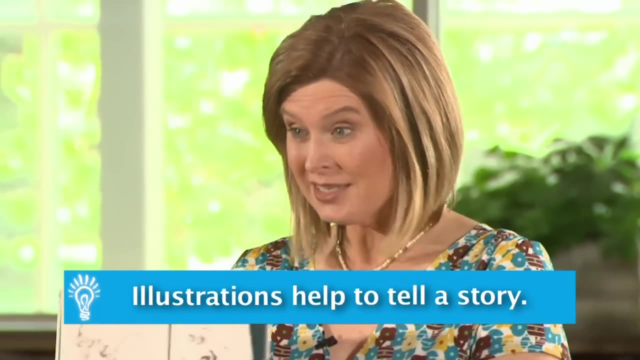 There are no words in this book. I like these kind of books, Having children when I would say, tell me a story or read me the book, and they would say: I can't, Mom, I can't read. Well, this is the perfect book. 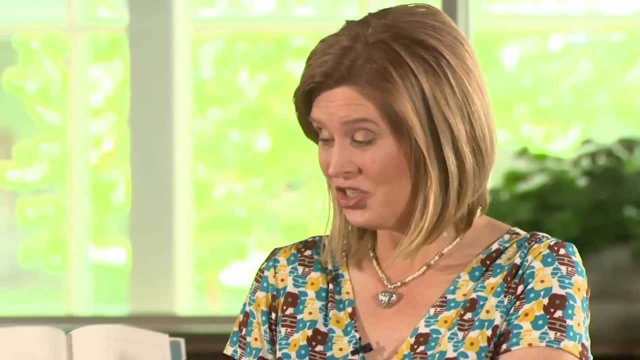 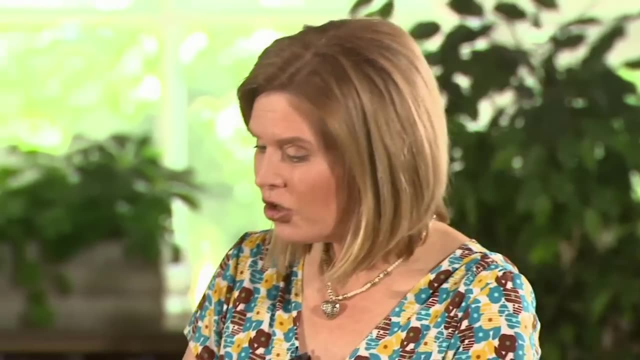 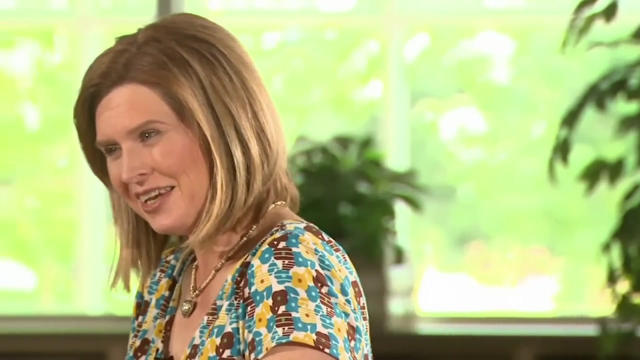 because there are no words. so it's your imagination, It's your story. Finding books that have a lot of pictures, where a child can tell a story, is very good in this pre-writing emphasis, where the pictures become symbols. Now how important are pictures? 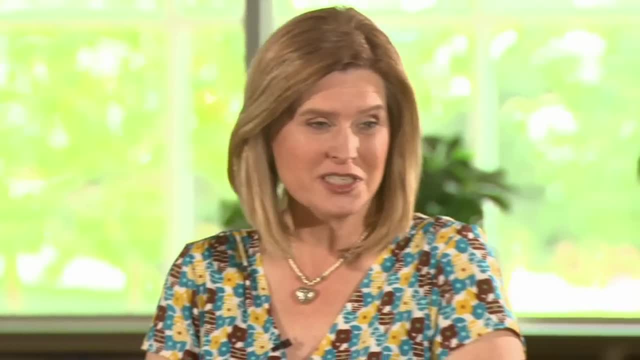 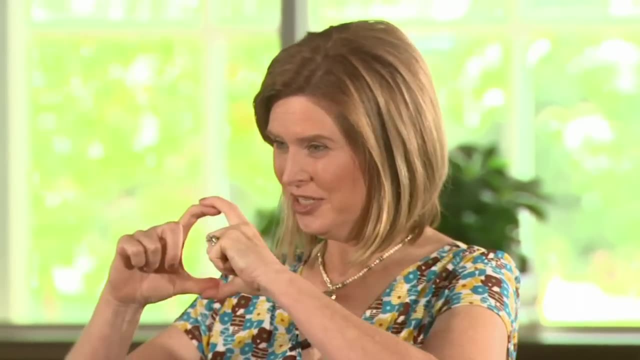 I would have to say I still I'll still read a particular book. There's a series of books that I like, and at the beginning of the chapter there's just a teeny, tiny little picture. okay, I'll look at that picture. 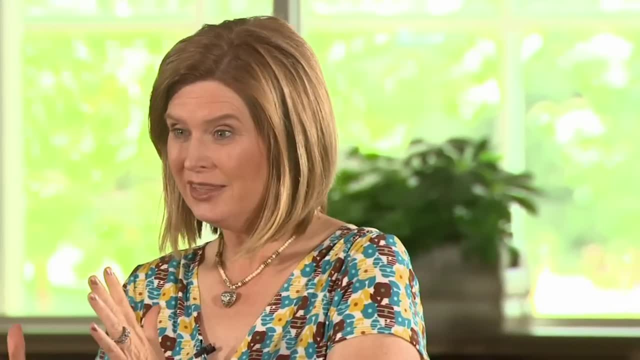 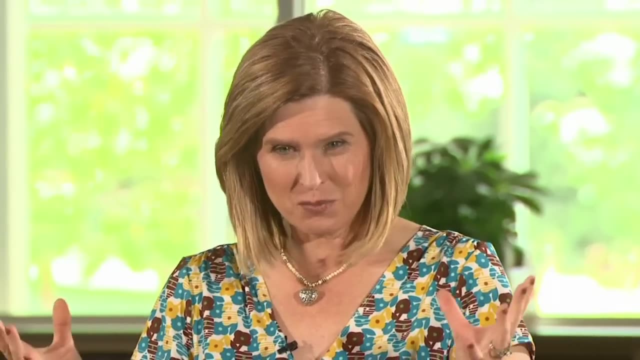 I actually will sort of study that picture, I'll read the chapter and then I go back and look at the picture and think, oh, that's what that meant. Do you see how much the pictures mean? You know when they say a picture tells a thousand words. 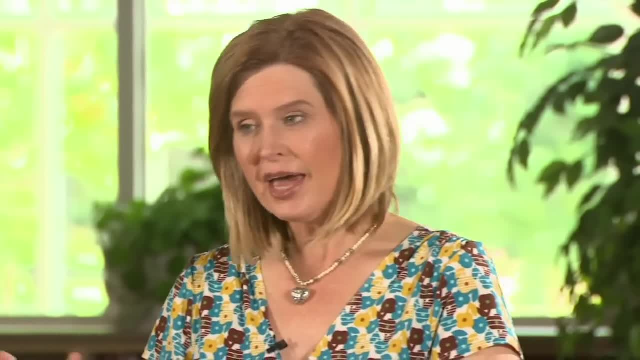 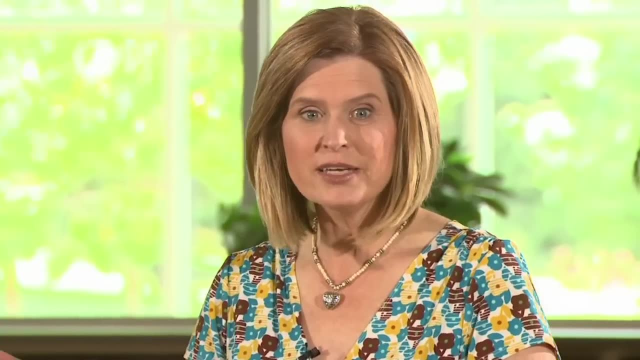 it's very true. It tells the whole story As you're reading a book. have you ever read with a child that you've finished reading the words? and you turn the page and they're like: wait, I'm not finished yet. 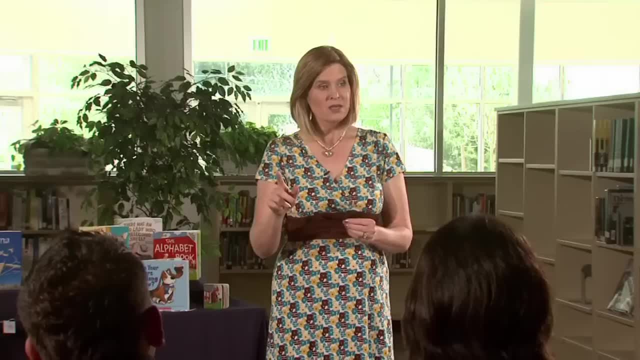 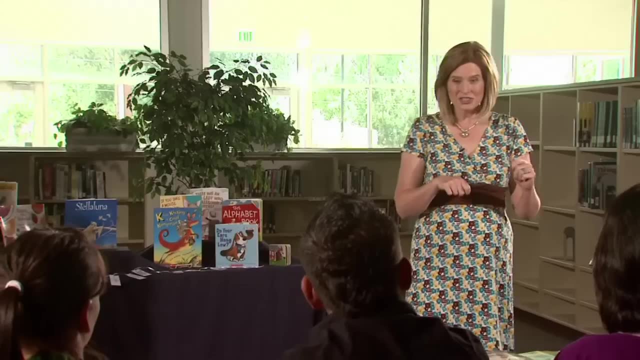 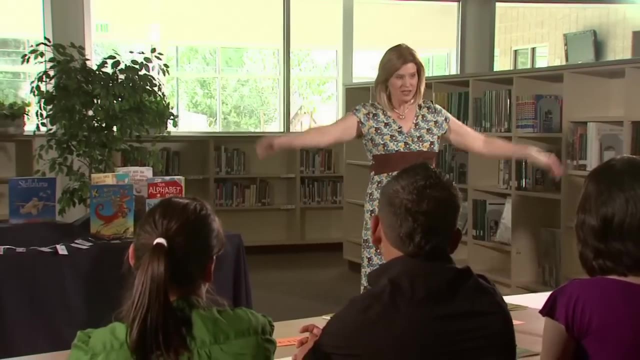 Because the picture tells the story. So remember, environmental print is the start of the writing process and a child will start to actually draw pictures to tell you a story. You might start out as a big blob, then you have little stick arms. 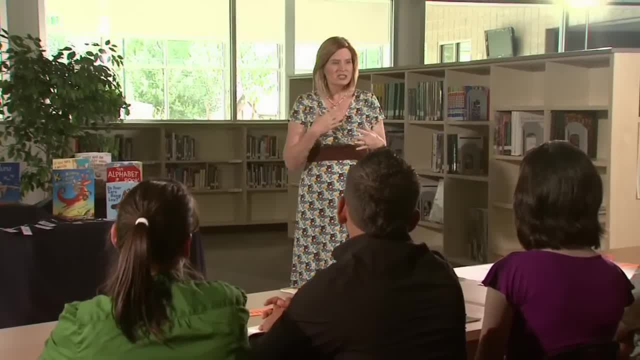 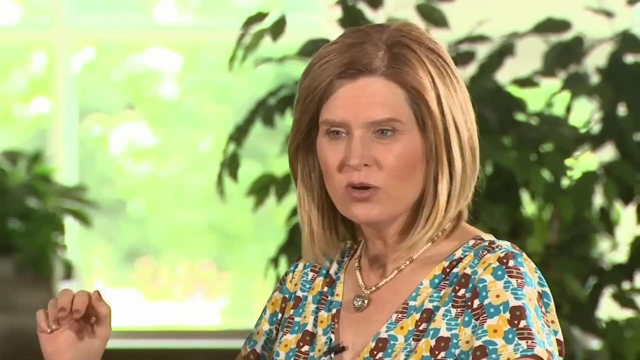 and sometimes you have eyes and then you add hair, but it actually tells a story. In this particular clip, a little boy is sharing a story of what they learned in school, and it's not with words, it's with pictures. It's an investigation. 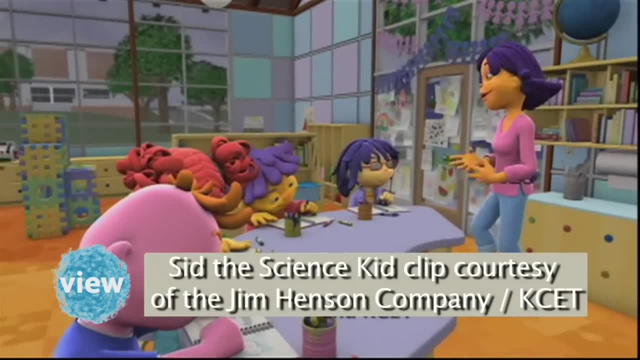 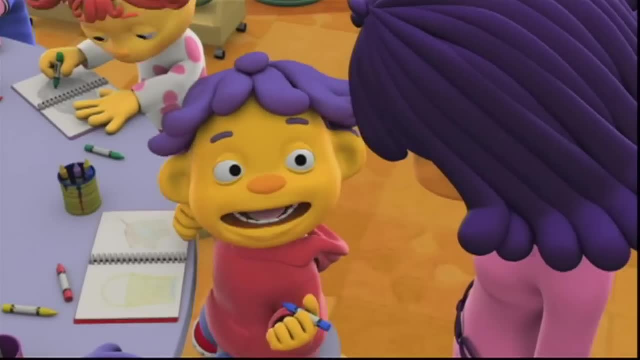 Our umbrellas kept the rain off of us and we're back inside, nice and dry. I can't wait to see the observations you made. Let's start with you, Sid. Okay, Well, here is my plastic bucket While I ran around in the rain. 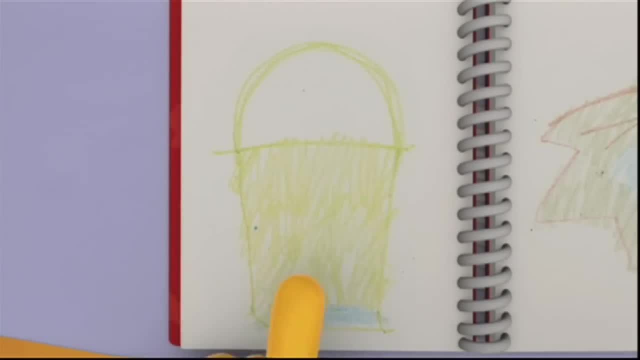 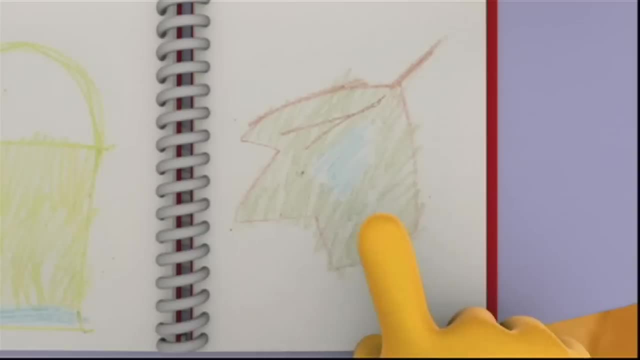 I left it in the sandbox. When I came back I found a little bit of water in the bottom. Then I found this leaf. It had its own little puddle inside. It was like um a little leaf bucket. Great observations, Sid. 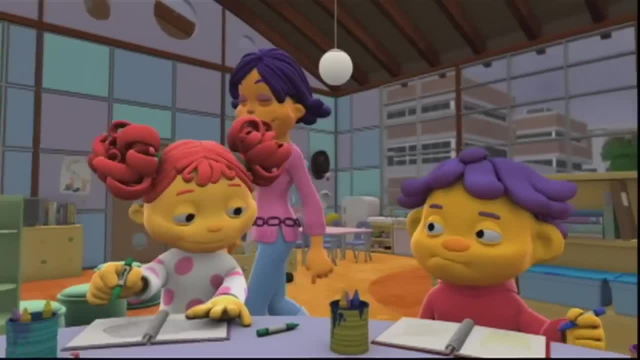 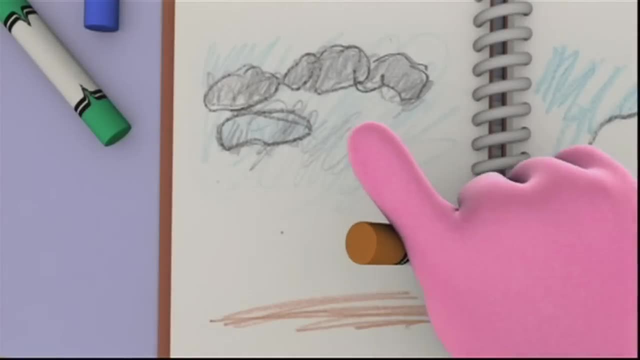 Yeah, Rainwater collects in lots of places. Hmm, Okay, Gerald, can we see your journal? Oh, yeah, okay. Well, I drew a picture of the sky and there were lots of dark, wet, rainy clouds up there. 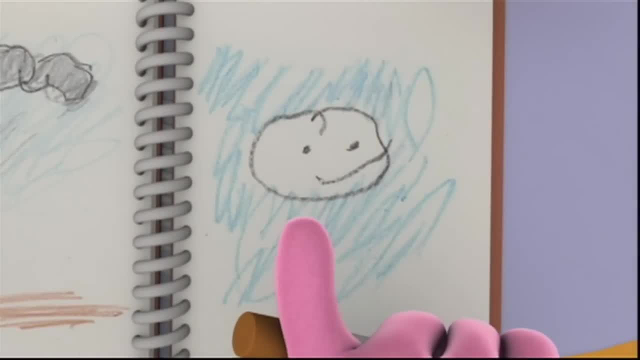 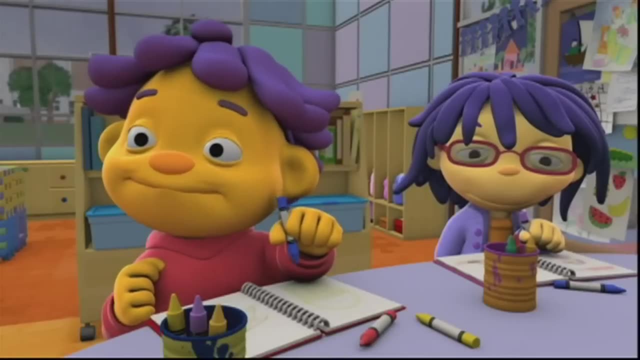 Um, okay, but then I saw one little puffy cloud all by himself. I named him Puffy And it looked like um. he was floating on the playground. Hey, you know, if he ever gets here, then I predict it'll stop raining. 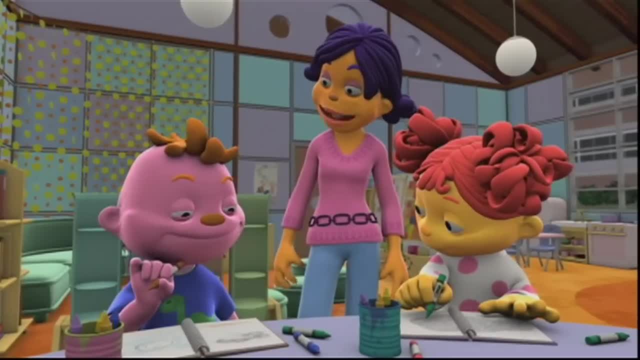 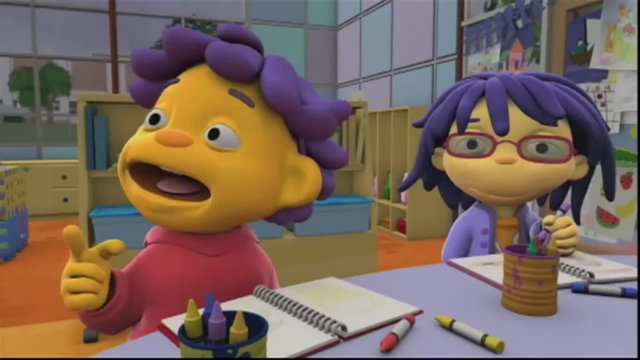 because he's not a dark rain cloud. Wow, Gerald, you made an excellent prediction. Thank you. You saw a white cloud and you predicted the rain will stop. Yeah, and I hope you're right, Gerald, because then we'll observe rain and sun today. 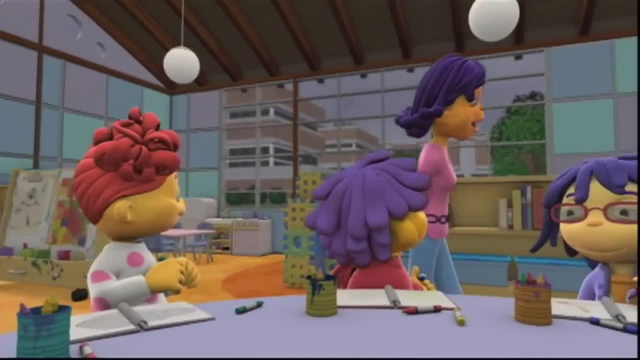 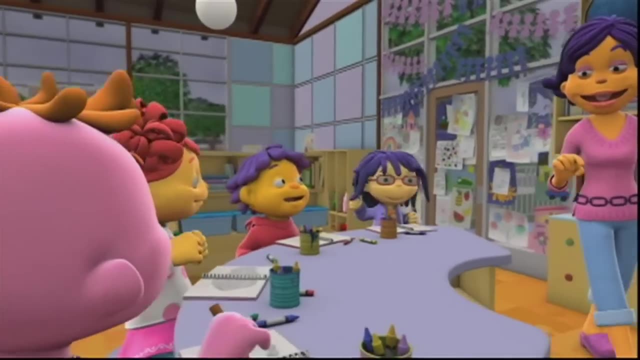 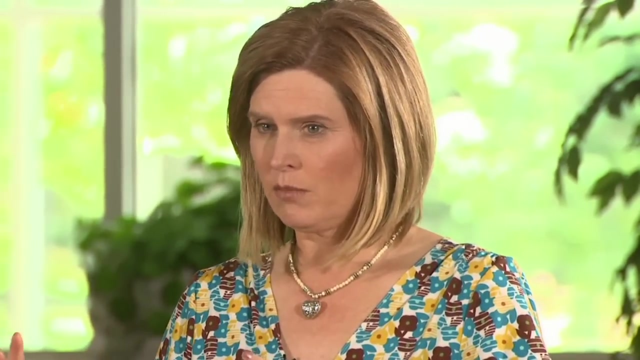 Maybe we will. Let's take a peek outside and see: Oh hey, look, the rain stopped. Oh, Oh, You can play outside with all your new ideas without your umbrellas. Okay, it was all their pictures that made meaning for them. 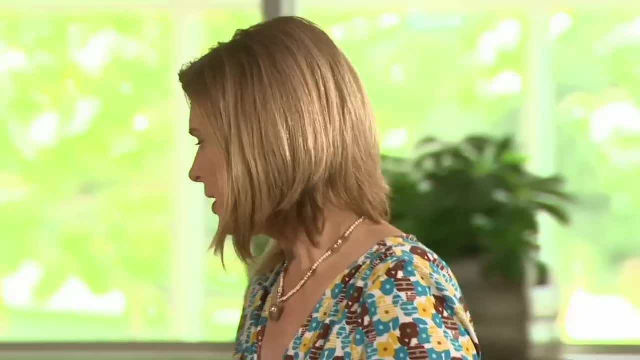 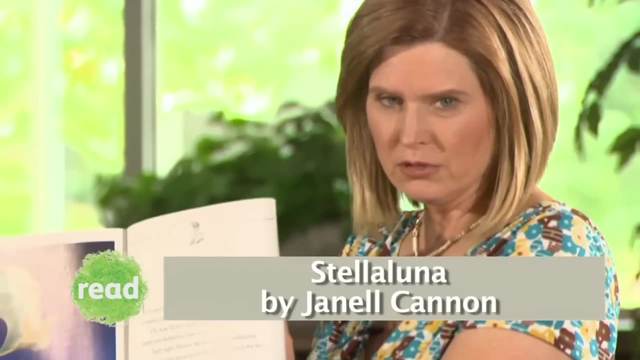 and they knew exactly what they were talking about. One last book that I'd like to share with you in this section about writing is a book- Stellaluna- and I just want to show you the pictures, Beautiful pictures, Just I mean, they're incredible. 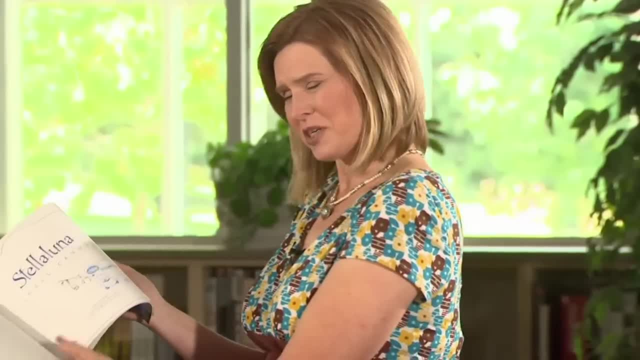 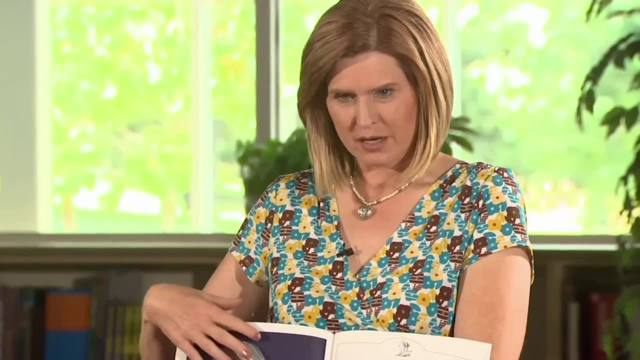 Um, what's interesting is- and I read this book several times before I noticed it- but in this story there's the words that tell the story of Stellaluna a bat, This little story that's right at the very top. 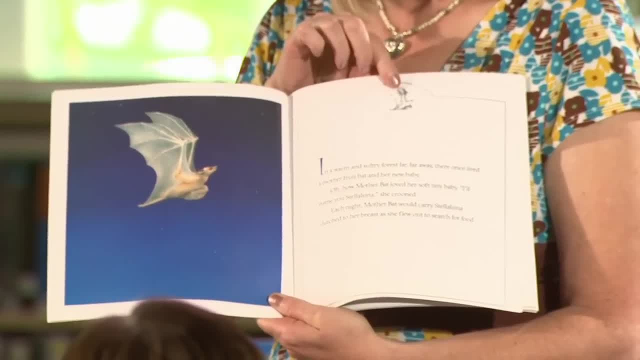 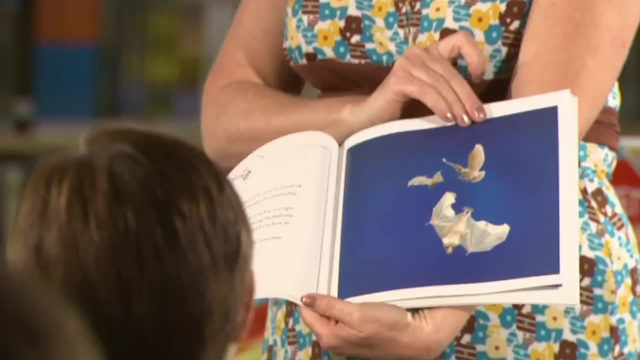 that's very, very small, tells a story of Stellaluna's mother. Now, when they're together, the pictures are the same and as they separate, because they are separated and Stellaluna has to go live with some birds- 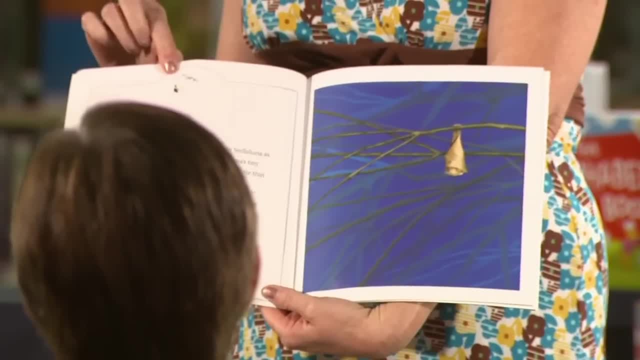 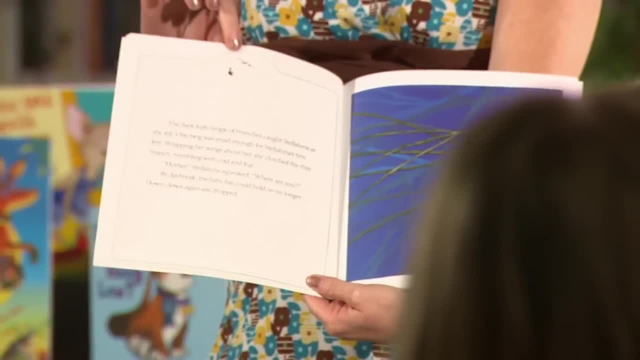 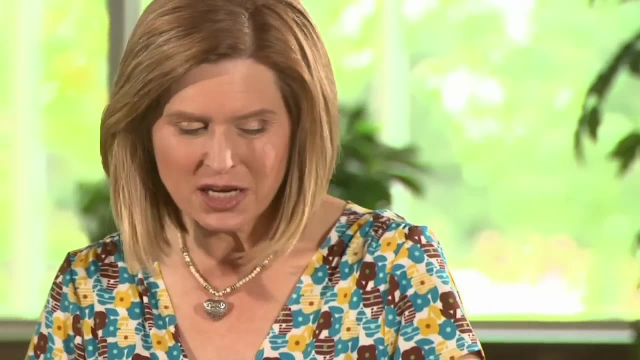 and here tells the story of Stellaluna. It's a fun story to read a couple times and then to show to children just this teeny little picture that tells a whole different story. Now, as we talk about writing, we do start include letters. 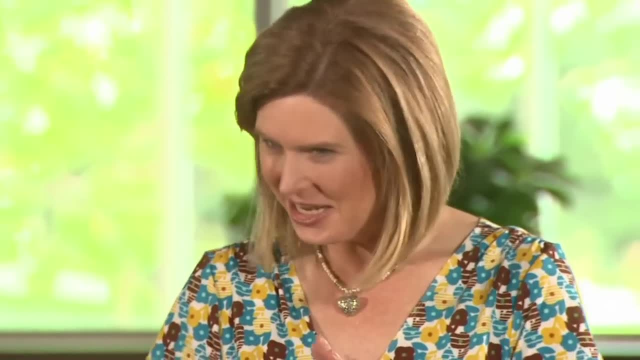 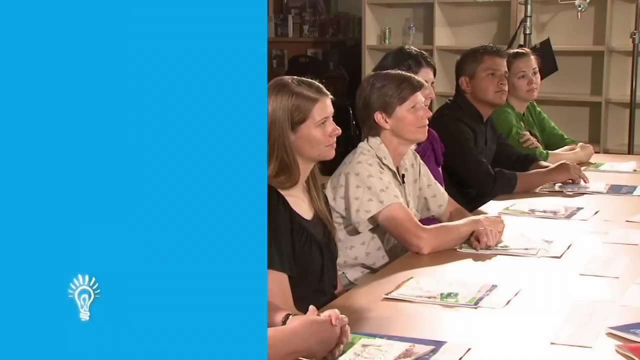 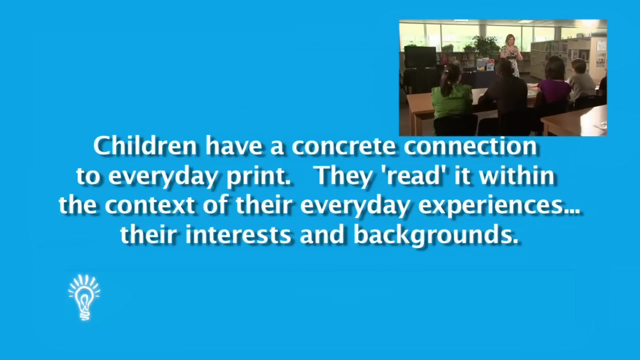 and the first letter that any child- any child- ever learns is the letters of their name. Those are the very first letters that they learn and, just as a heart or a stop sign or the lady's restroom, those letters don't have a sound yet. 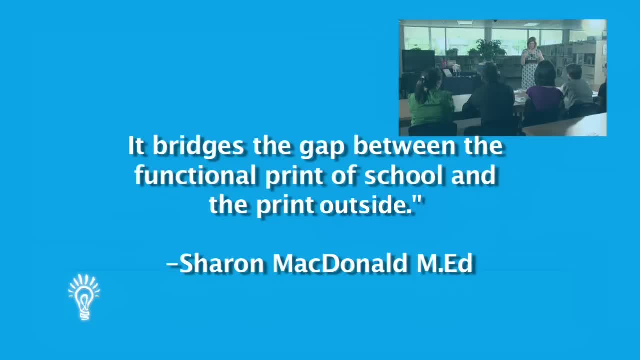 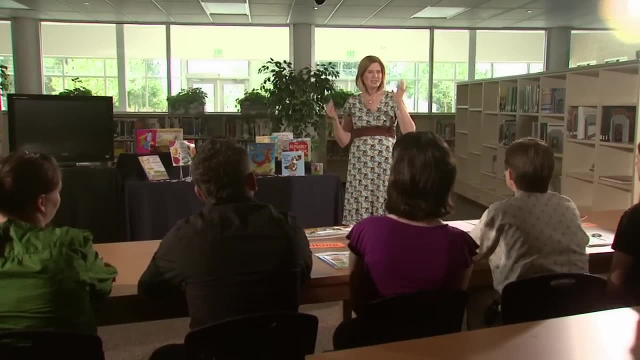 but they are a symbol of that's me, mom, that's me, And so they'll be driving around. and if their name is Tom and they see a T, even in stop sign, there's my name, mom, there's my name. 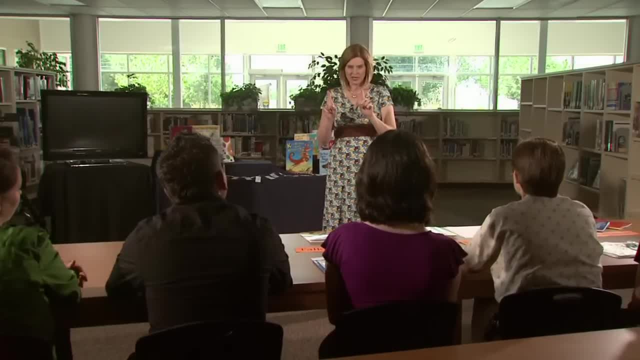 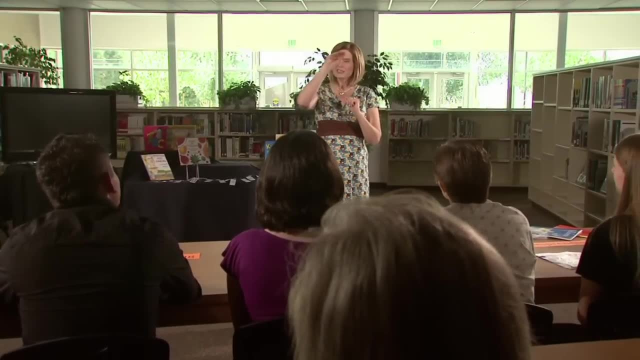 And it's usually the first letter and the last letter that they'll recognize, And then those other letters will come next, And that's where we get. we're going to, you know, just segment into our next stage of decoding. But remember at that point, 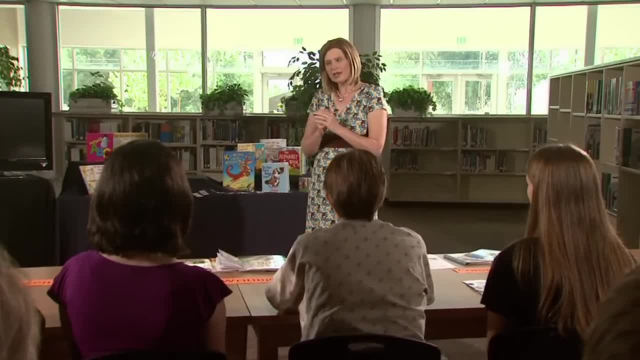 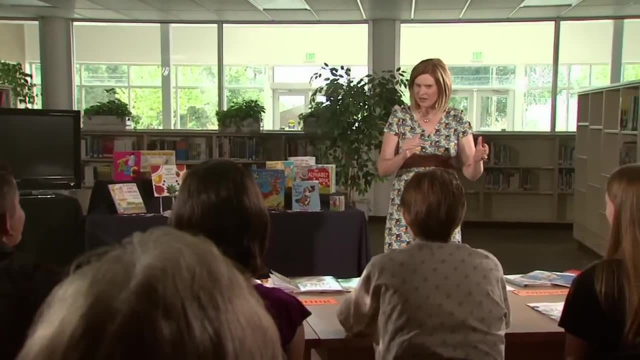 letters are still symbols. They have a meaning And that's why they write them all over your house and in your books and in your car, on your mother-in-law's brand new leather couch, because it symbolizes that is me. 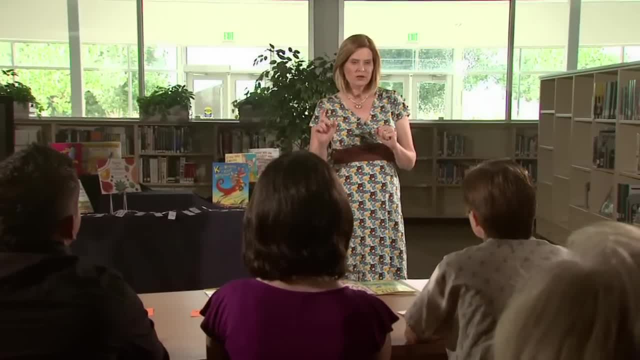 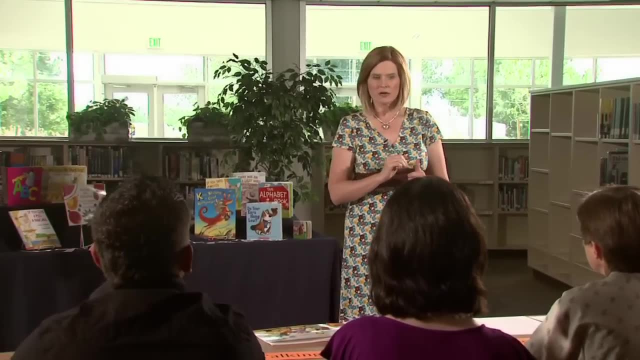 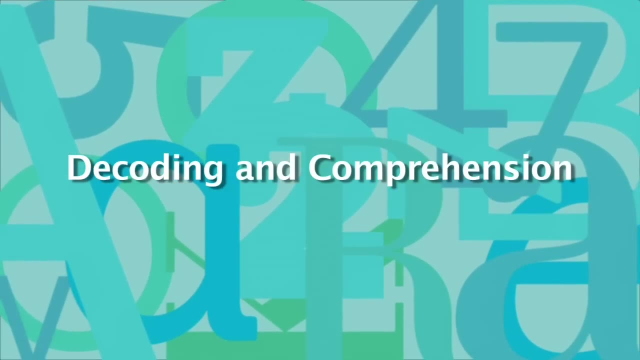 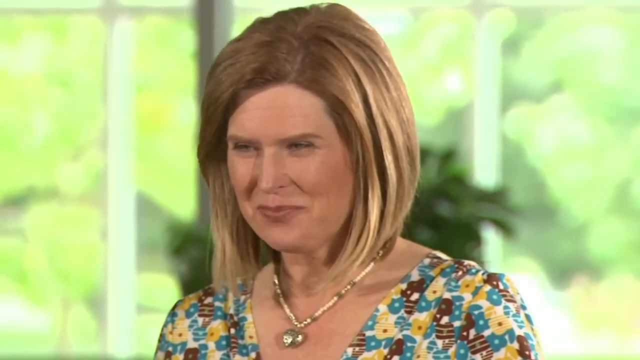 And so recognize that that is a very important part of writing. Let children know, let children scribble, let them draw you stories and then let them tell you That's part of writing. Decoding- Okay, decoding for me as a parent. 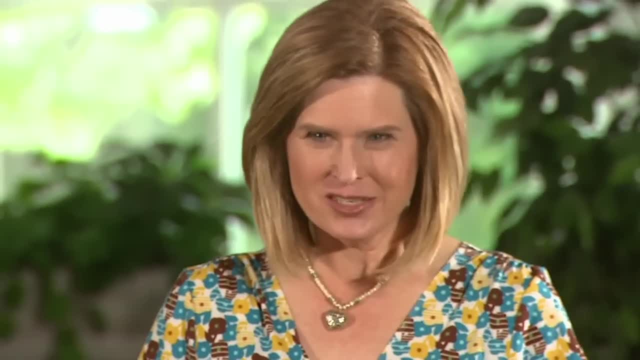 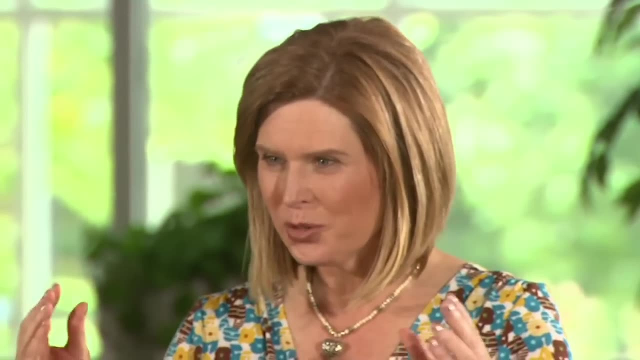 I have to say, was the hardest part of reading. It's where a child will actually take a word. they know the specific sounds of each letter and then they start putting it together Like cat and hat and fat, And they're not looking. 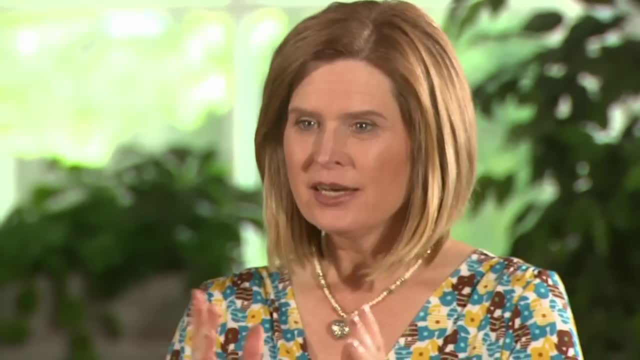 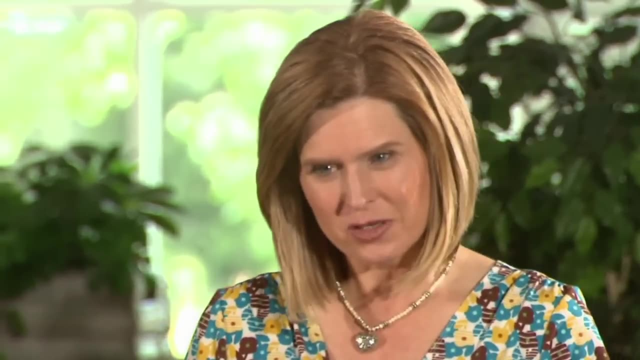 they're looking at each individual letter and they're putting it together. Now, the best way that I can describe decoding is: I want you to think- most of you in this room- if I ask Candice to read a page of a book. 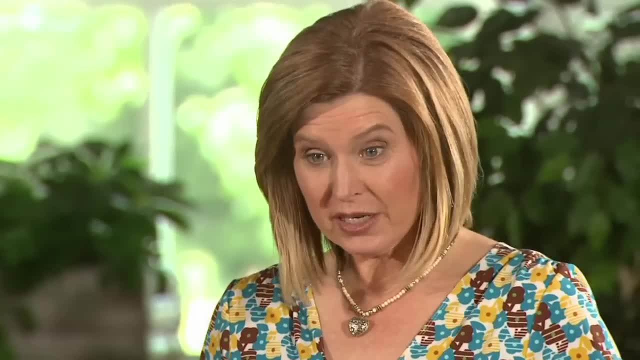 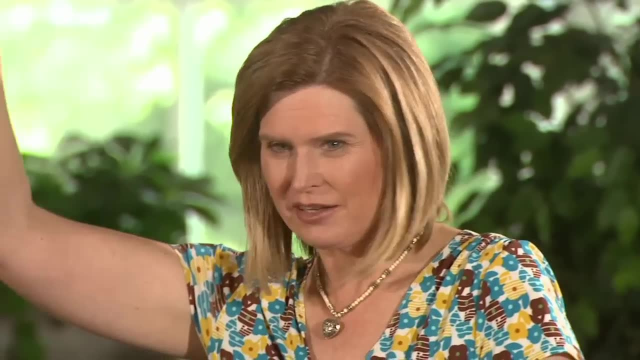 she's a pretty good decoder And she could probably read most pages on the book, right, Candice? okay, But how many have had that happen Where you've been asked to read something out loud by the raise of hand? Nobody's ever been asked to read something out loud. 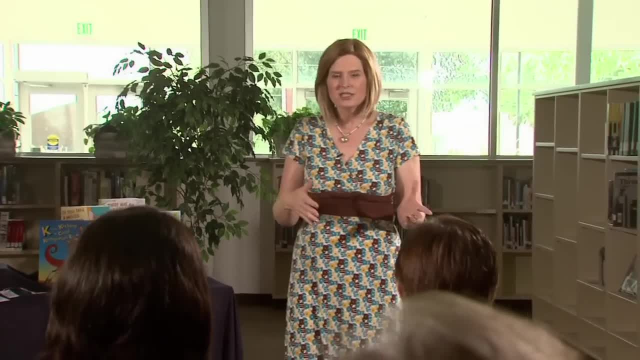 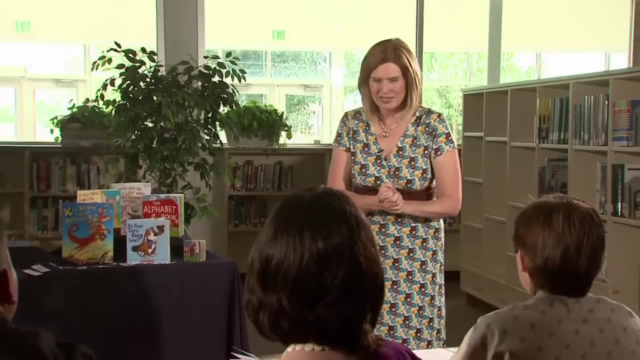 And so, as you've been asked to read something out loud, then you sit down and then the teacher goes on and says: now, Erica, could you tell me what that means And what usually happens? Erica, You have no idea. 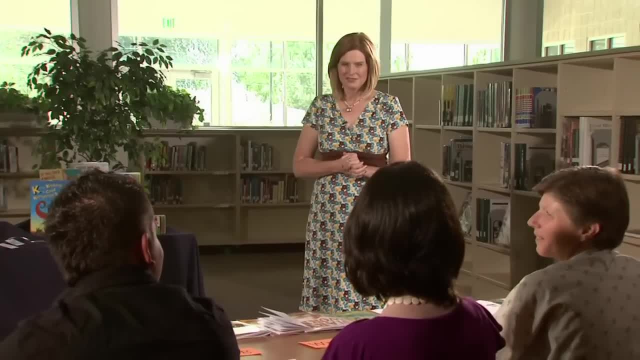 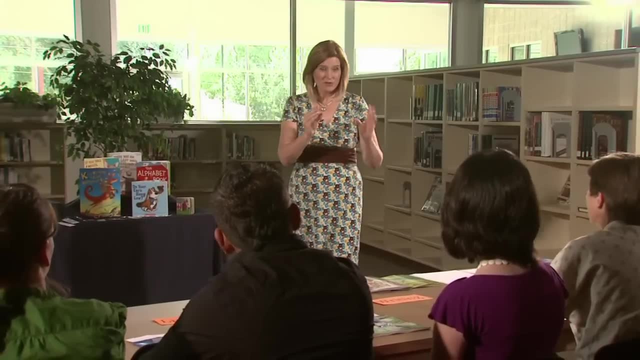 You're so focused on reading it and reading it correctly that all meaning goes out the door. Okay, and that's exactly what children are doing when they're decoding. okay, They are so focused on sounding out those words, on getting it right. 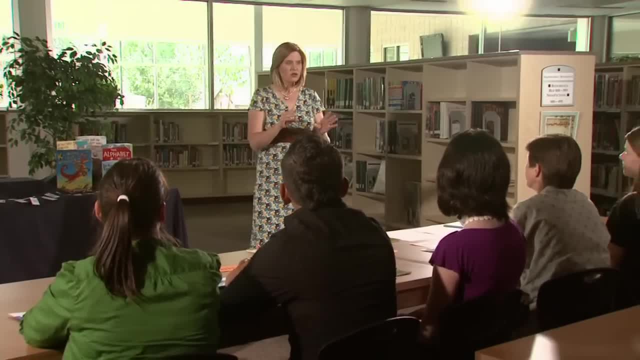 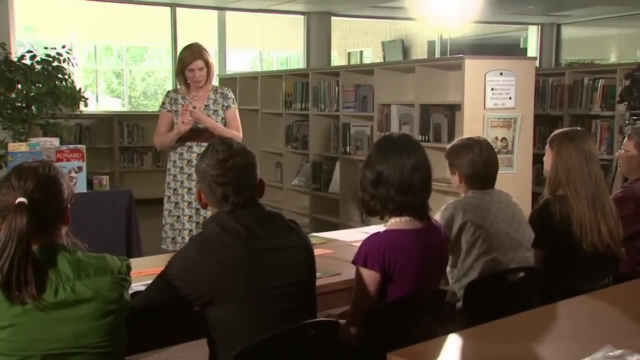 that the comprehension is not there. This is a good time when children are decoding or in a decoding stage is to read the book before they read it. You're not cheating, You're not giving away anything, but you're giving them. 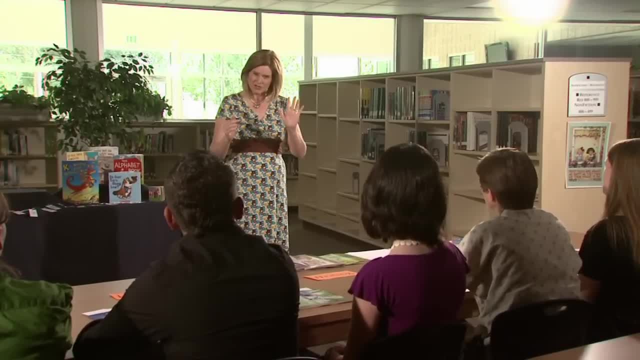 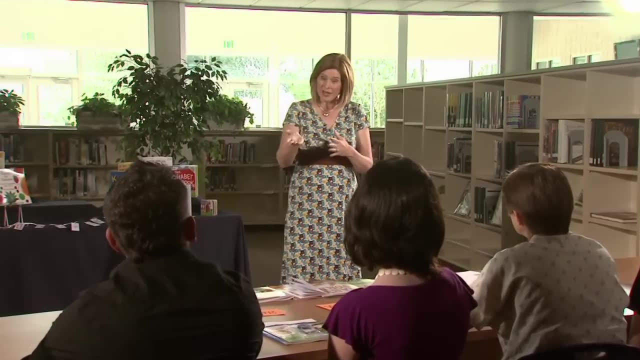 oh, this is what's gonna happen in the story, And then they can concentrate on decoding, or maybe, after they've decoded a few words, then retell what they've read. That is why reading to grade levels above where they are is a great, great idea. 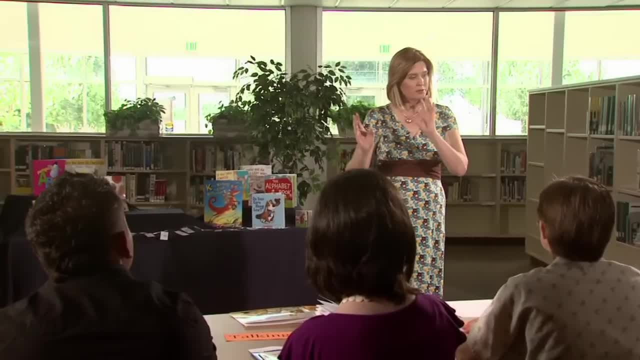 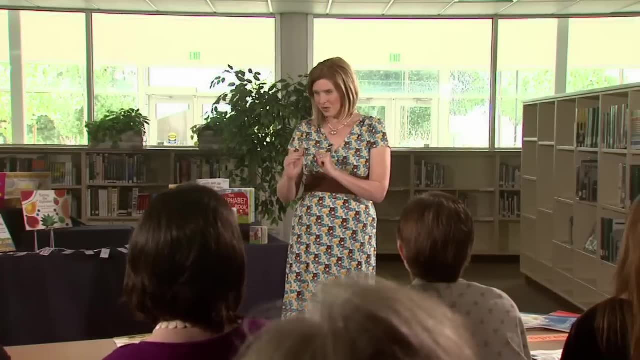 because it helps them still get new vocabulary words, helps them with the comprehension and they're not, so they don't have to focus on the decoding. Decoding is very difficult, It takes a lot of practice and we still do it as adults. 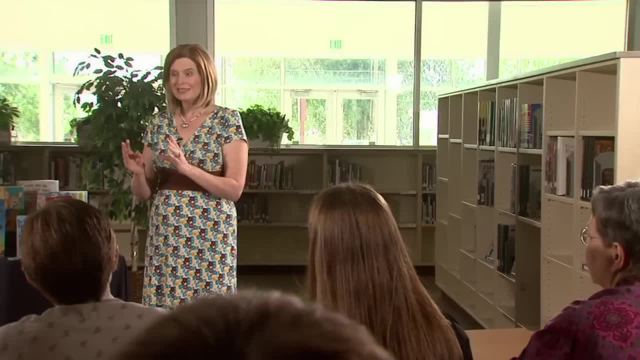 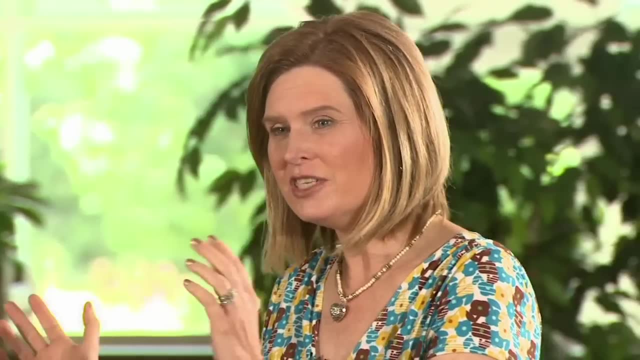 And so as you decode- remember decoding does not mean comprehension- I'm going to show you, okay. I'm going to show you okay. I'm going to show you a clip, or you're going to watch a clip of decoding where you take individual letters. 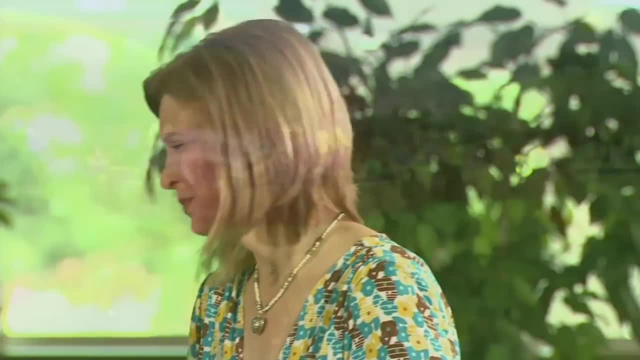 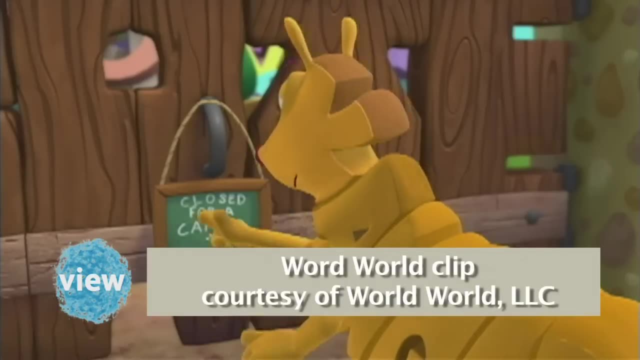 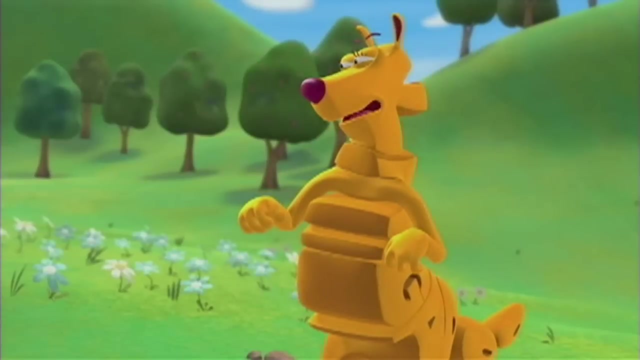 and you make the sounds, and then you make it build a word. Guru stopped by for a special delivery, G'day, g'day, g'day. What's this then? Closed for a catnip Signed Cat. Huh, crikey. 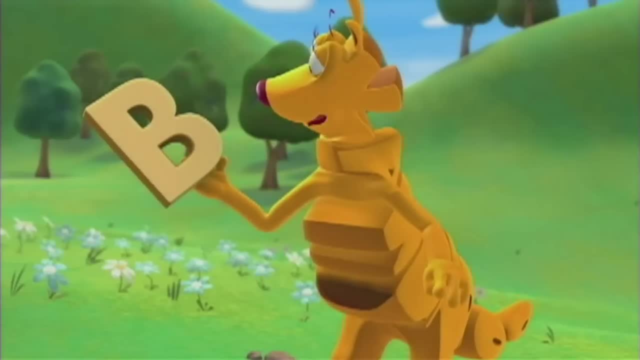 I'll just leave Cat's mail right here so she can see it when she wakes up: Mm-hmm, mm-hmm, mm-hmm, mm-hmm, mm-hmm, mm-hmm. Ooh, what could this be? 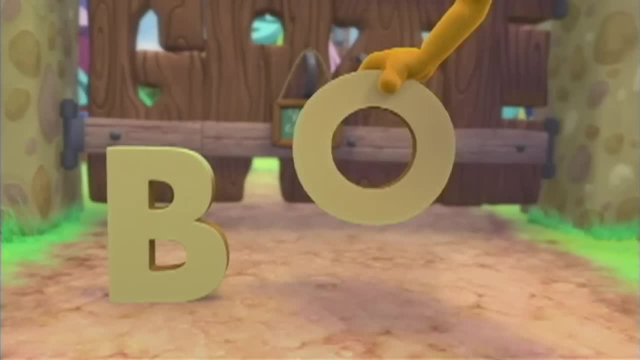 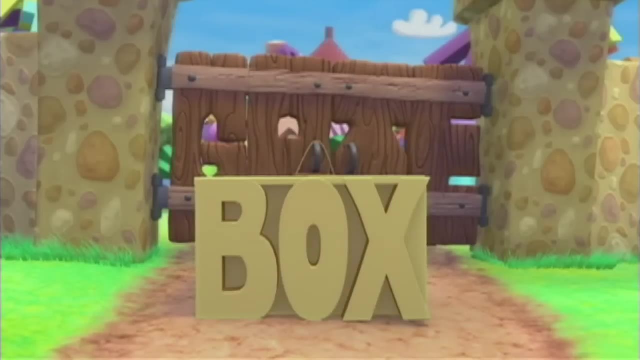 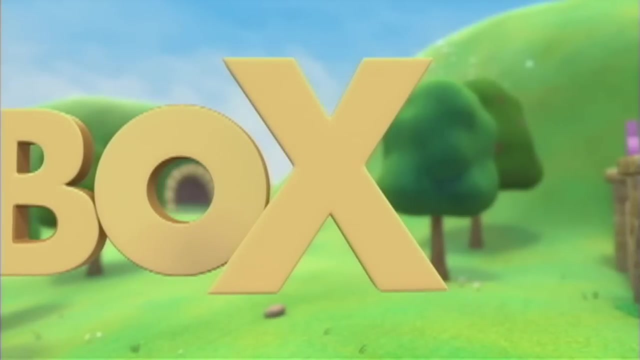 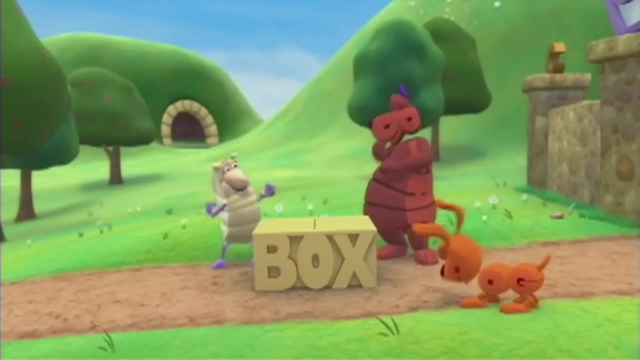 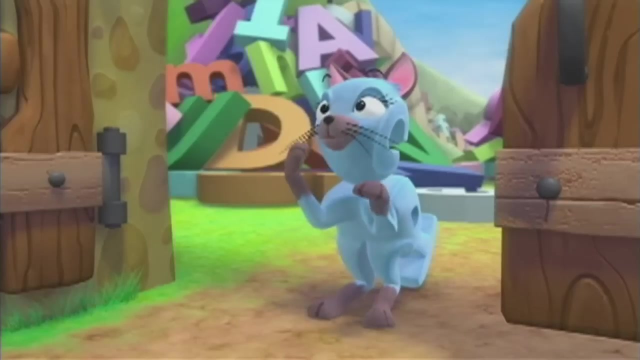 Let's see B-O-X Box. B-O-X Box. Yeah, we just built a word. We built it. we built it. Oh hello, What are all of you doing here? What's this? A box for me. 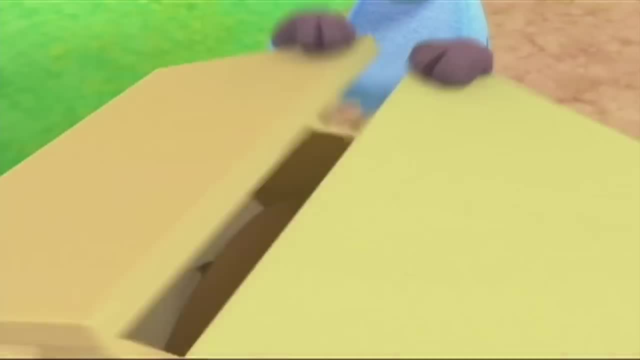 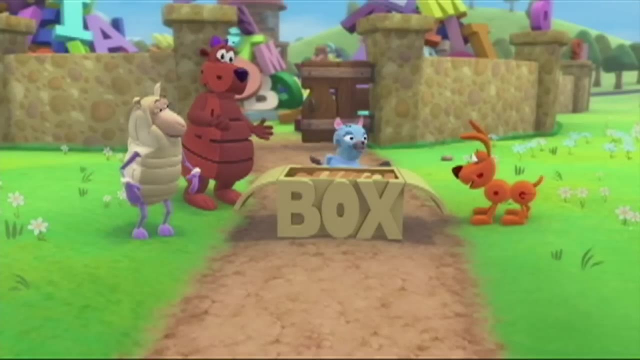 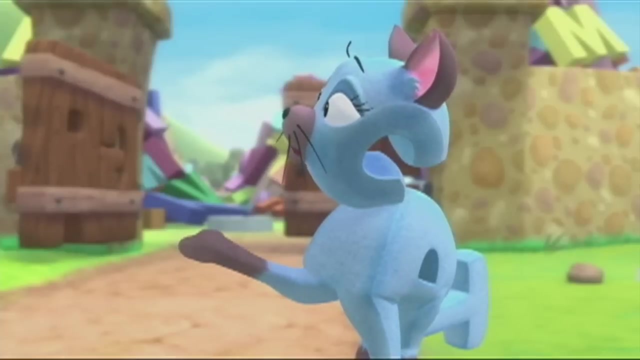 Oh, I'll just bet. I know what this is: My O's. They're finally here. I just ran out O's, Yes, O's, See Oopsie Runaway O's. Can you guys help me catch them? 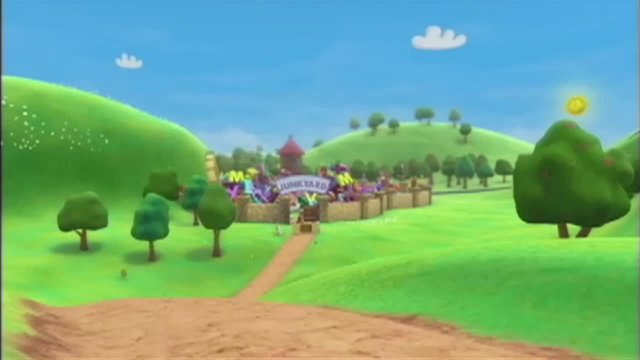 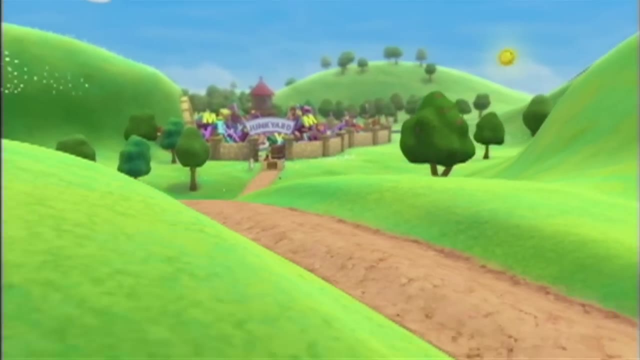 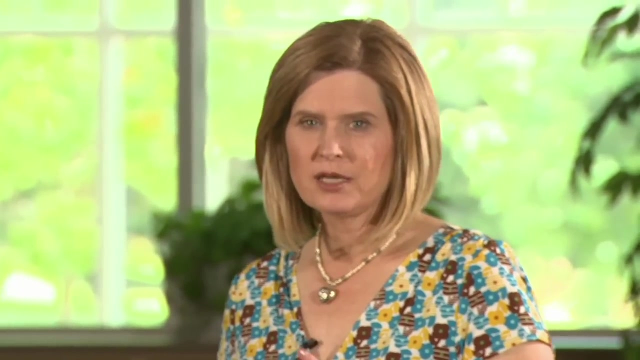 It's a long story, Cat, A story that it seems will continue to follow the further adventures of the round rolling runaway. letter O The end. So many shows that PBS airs actually has this decoding where you're putting words together. 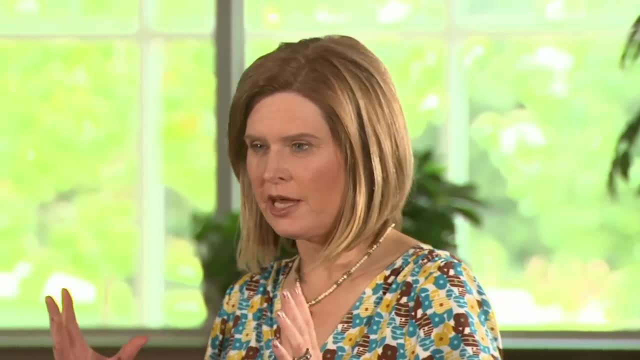 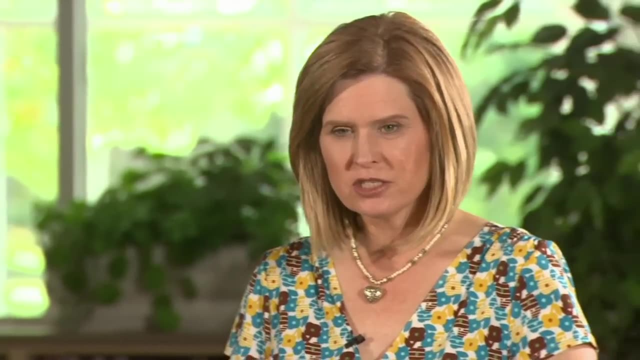 where you're actually shoving them together, and then we decode the words out loud for children and they're able to see it and hear it and do it. Remember in the decoding stages, make sure that your children are not reading. 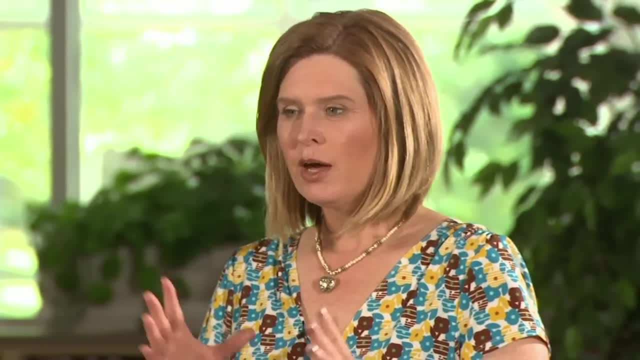 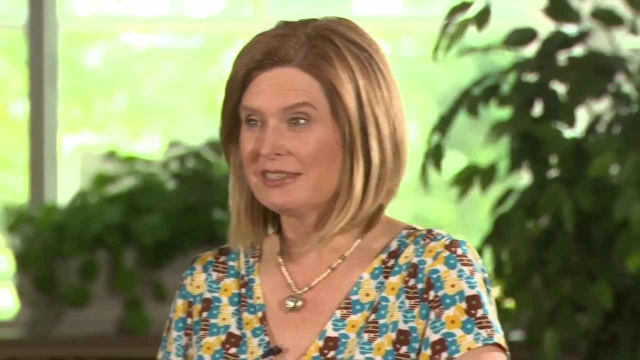 above their grade level, but they're finding words that they can sound out. Once again, this is the hard one for me as a parent, because I actually want to give the word away. you know when they're sounding that out. I just want to tell them what the word is. 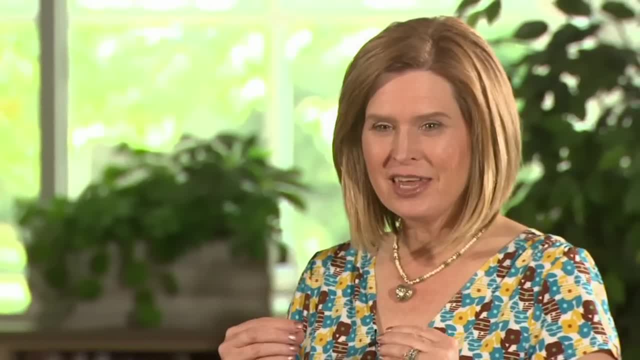 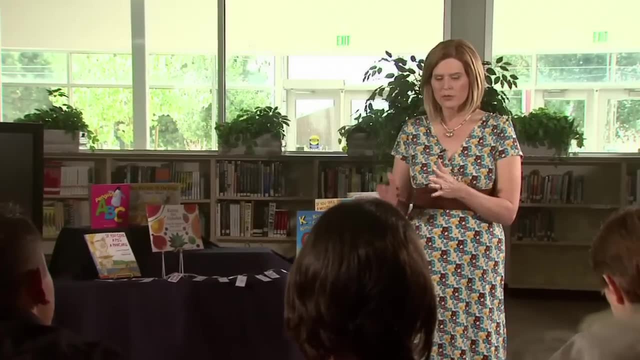 But sort of bite your tongue, let them decode and then they can move on to that comprehension stage. I really liked it when Nancy and all of you were talking and you said that that comprehension really goes between each one that we need to understand. 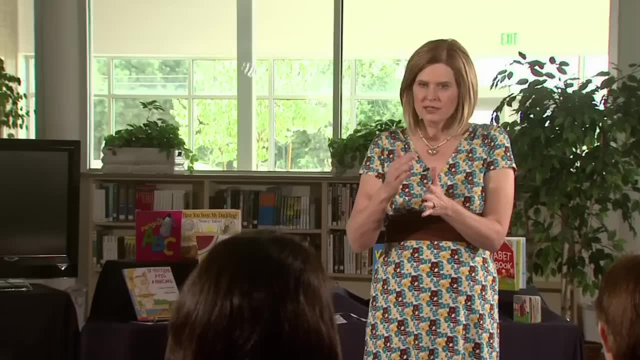 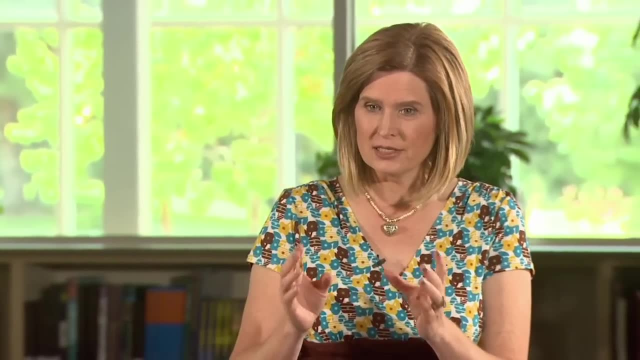 a child needs to understand what you are saying, and then they need to understand the words that they're saying- and we need to understand them too- And the writing, what that environmental print means and decoding In comprehension. this is where a child can read a book. 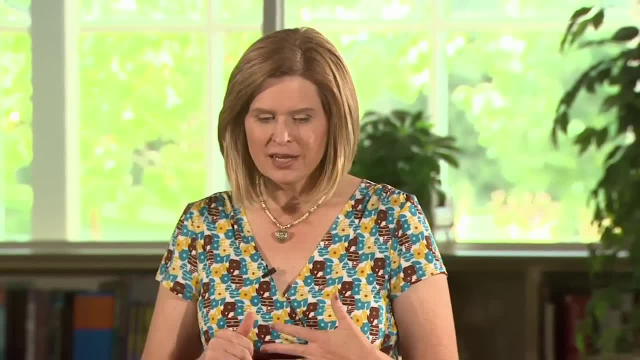 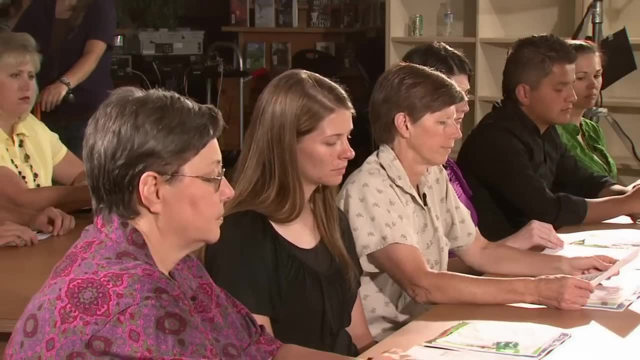 or listen to a story and understand what's happening Now in front of you. I have the paper. Then What Happened. Each of you have that And this is a great comprehension activity as a child, as you read to a child. 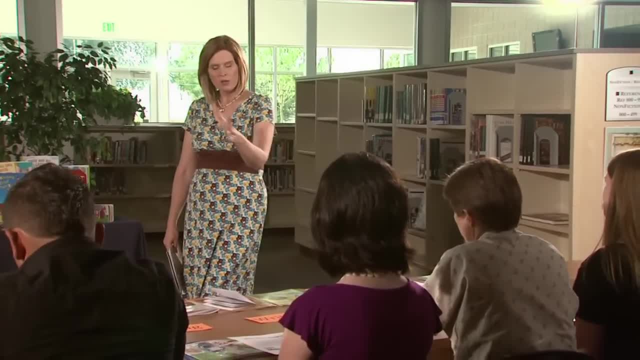 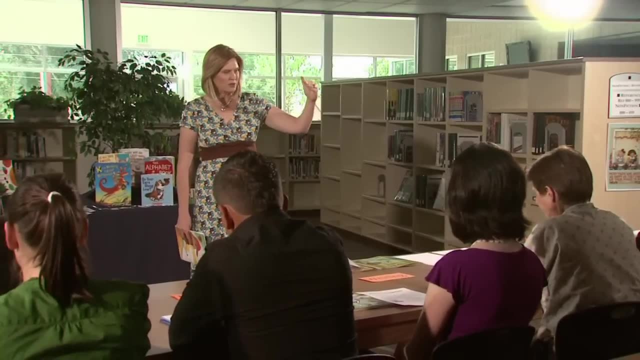 and then they try to figure out what happened next. Now we start this in kindergarten. A child might not have words in front of them. That way they would have pictures of what happened and then what happened: What was the beginning, the middle and the end. 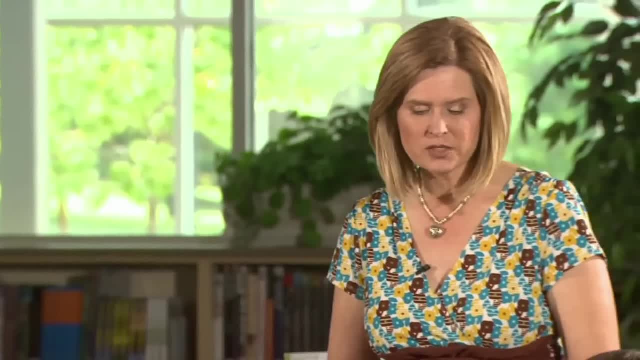 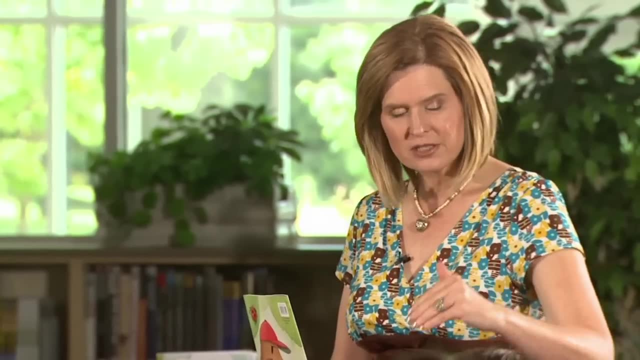 And that's story comprehension Here. these are words and so this would be for an older child. But as I read this book, I want you to sort of understand, sort of say: oh, this happened first, this happened second. 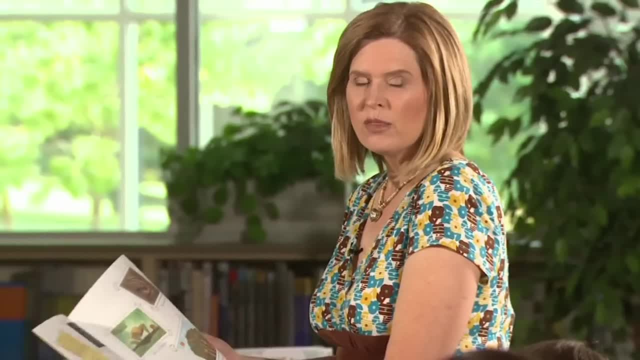 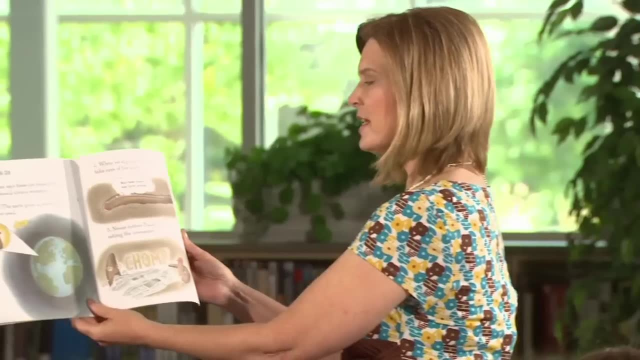 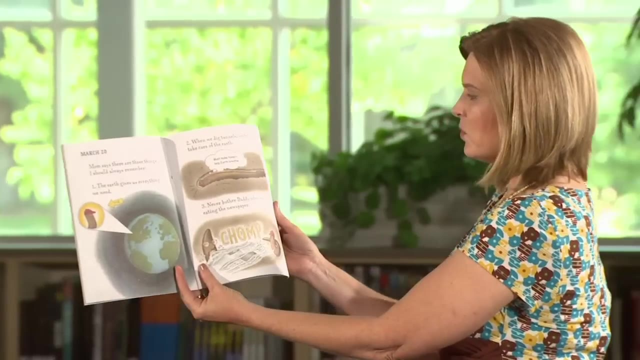 This is what we call story comprehension, when you know the sequence of the story. And this book is called A Diary of a Worm. Mom says there are three things I should always remember. The earth gives us everything we need. We dig tunnels. 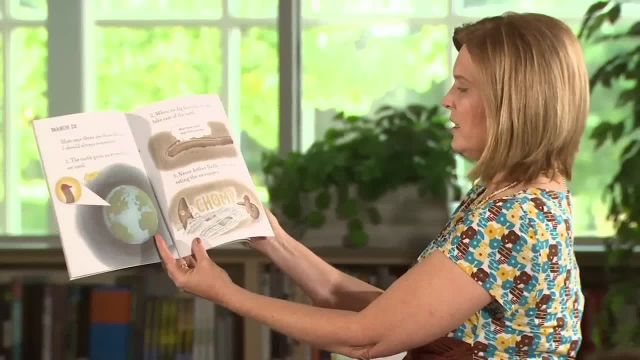 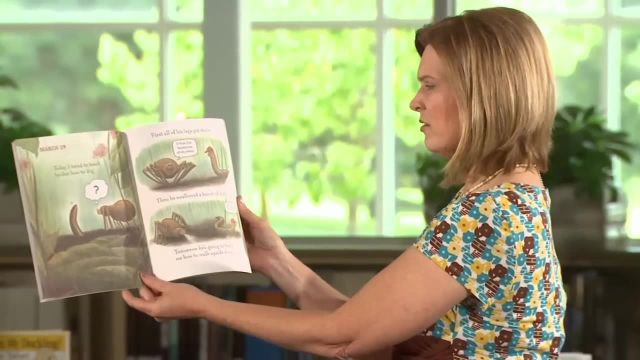 We can take care of the earth. Never bother Daddy when he's eating the newspaper. March 29th, Today, I tried to tell you, I'm going to tell you, I'm going to teach Spider how to dig. First of all, his legs got stuck. 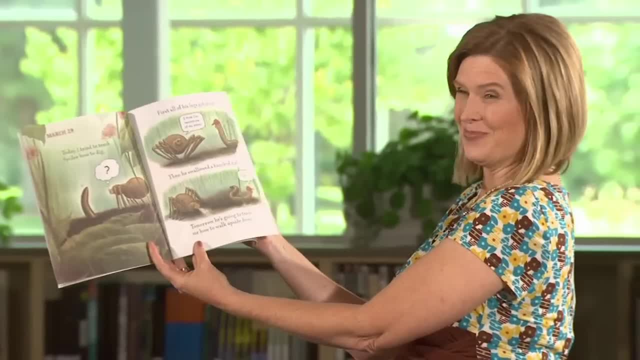 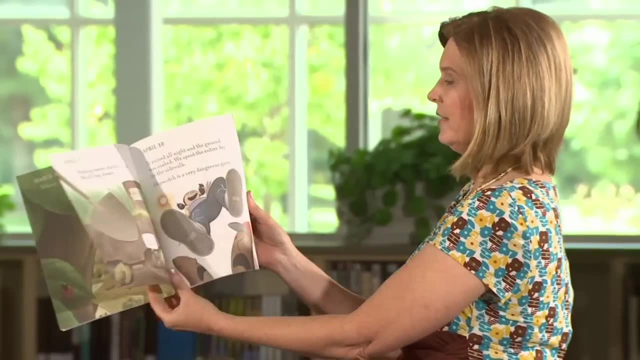 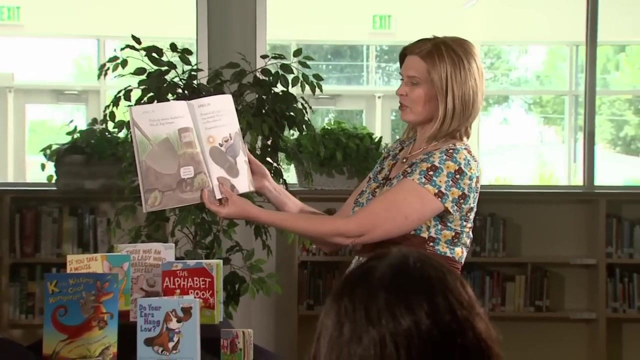 Then he swallowed a bunch of dirt. Tomorrow he's going to teach me how to walk upside down. March 30th: Worms cannot walk upside down. April 4th: Fishing season started today. We all dug deeper. April 10th. 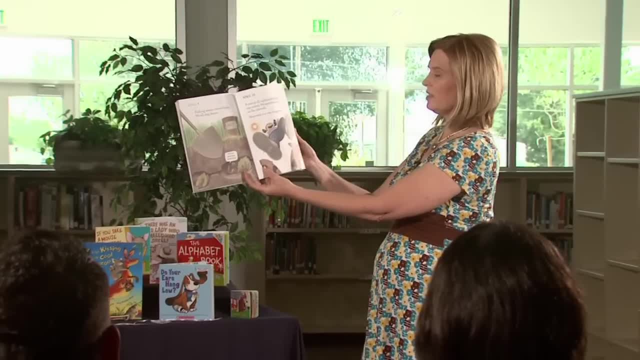 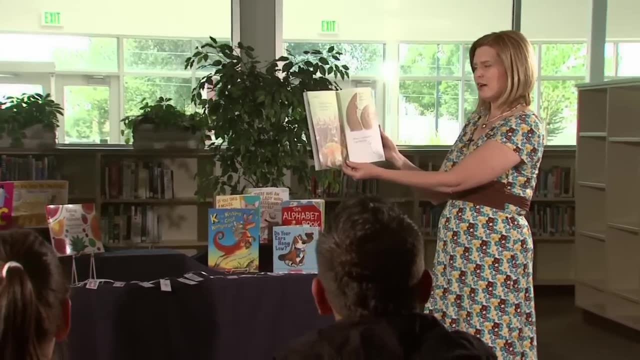 It rained all night and the ground was soaked. We spent the entire day on the sidewalk. Hopscotch is a very dangerous, dangerous game. April 15th: I forgot my lunch. today I got so hungry that I ate my homework. 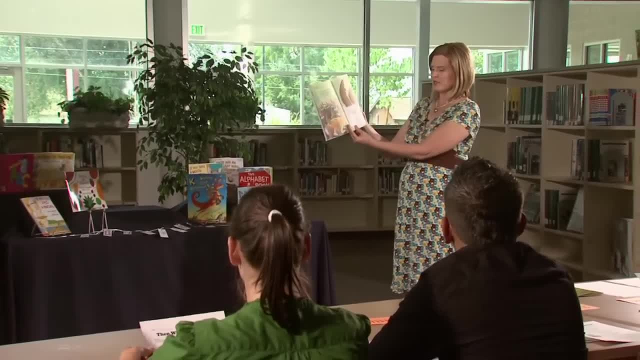 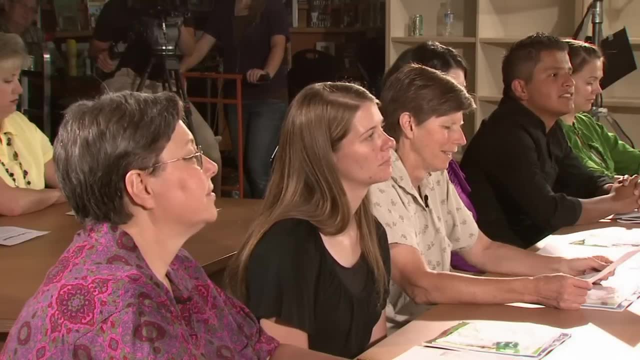 My teacher made me write. I will not eat my homework 10 times When I finished that. when I finished, I ate that too. April 20th: I snuck up on some kids in the park today. They didn't hear me coming. 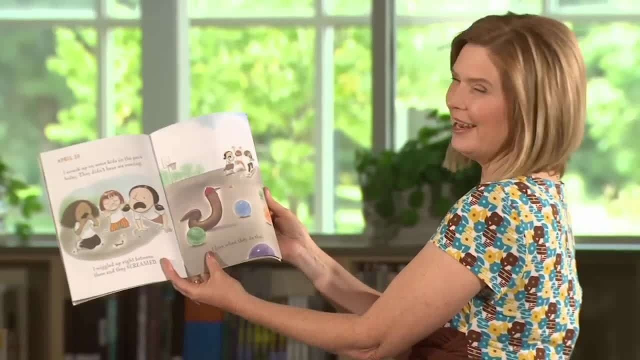 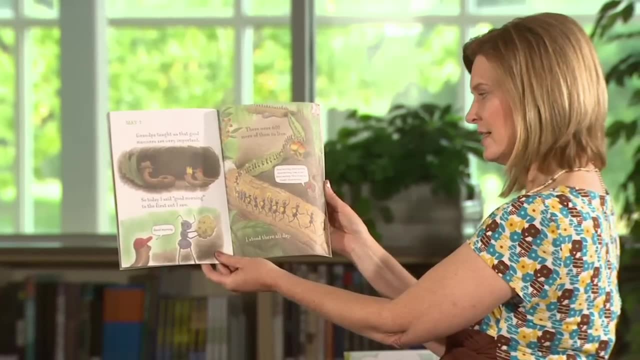 I wiggled right up between them and they screamed: I love it when they do that. May 1st Grandpa taught us that good manners are very important. So today I said good morning to the first aunt. I saw There were 600 of more of them in line. 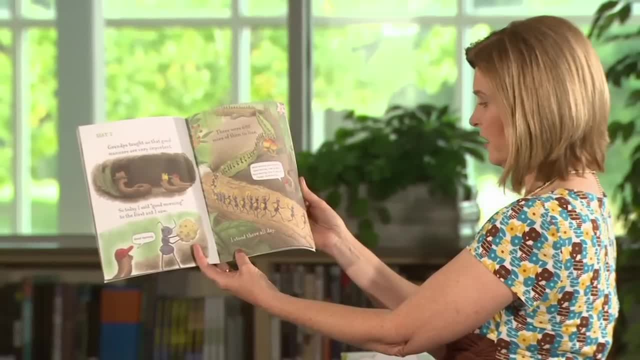 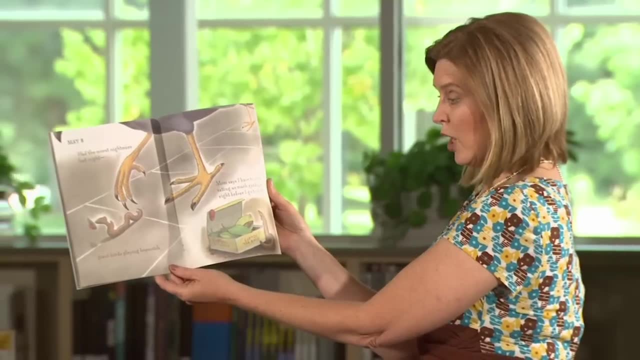 Good morning, good morning, How are you doing? Good morning, Nice to see you. Good morning, I stood there all day May 8th. Had the worst nightmare last night: Giant birds playing hopscotch. Mom says I have to stop eating so much garbage. 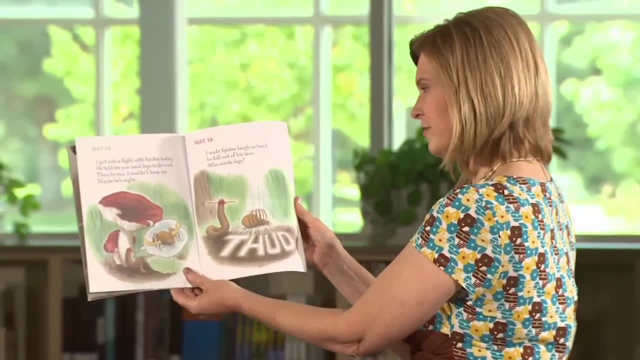 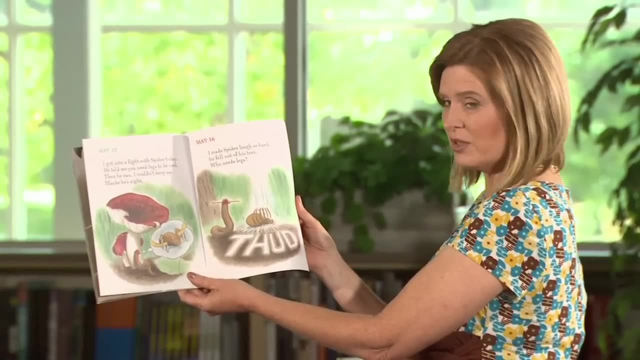 before I go to bed. May 15th: I got into a fight with Spider today. He told me you needed legs to be cool. Then he ran away. I couldn't keep up. Maybe he's right. May 16th: 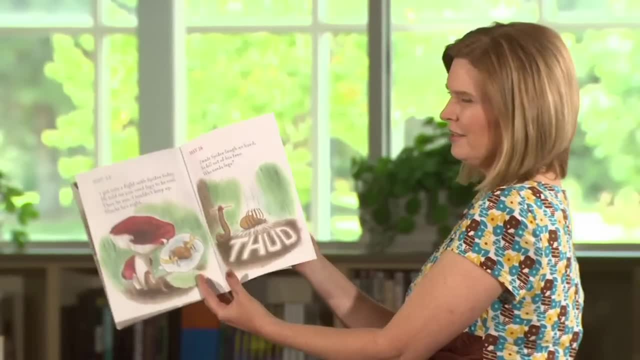 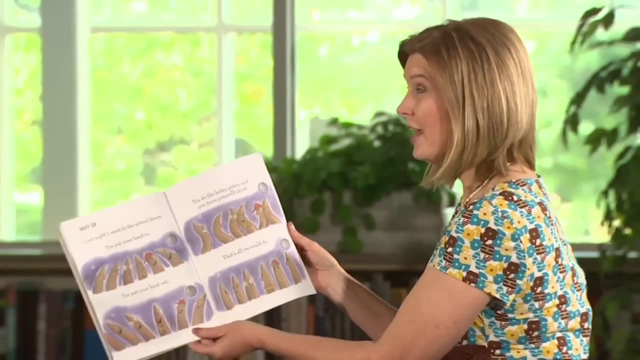 I made Spider laugh so hard. he fell out of a tree. Who needs legs? May 28th. Last night I went to the school dance. You put your head in, You put your head out, You do the hokey pokey and you turn yourself about. 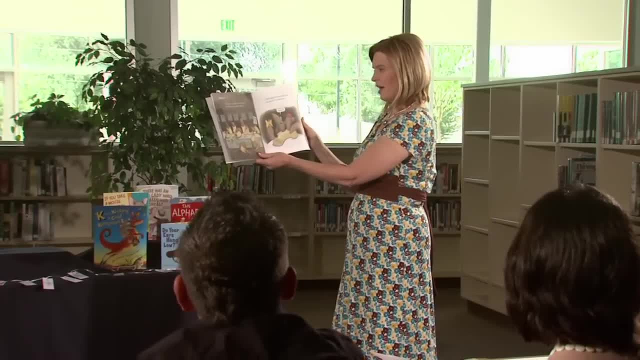 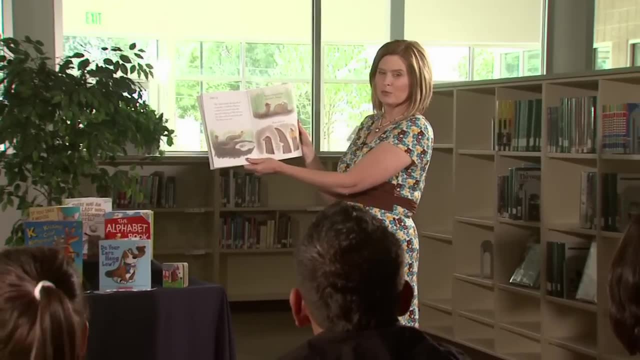 That's all we could do. June 5th: Today we made macaroni necklaces in class. May 16th: I brought mine home and we ate it for dinner. June 15th- My favorite day. My older sister thinks she's so pretty. 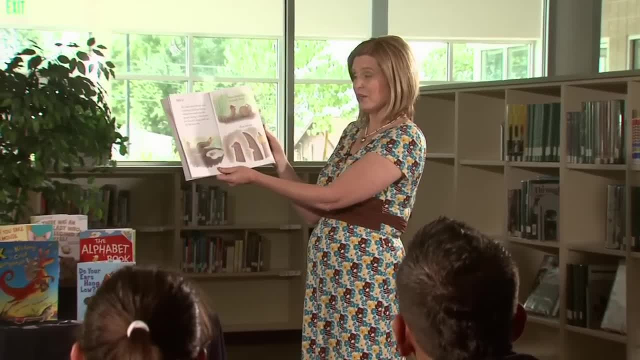 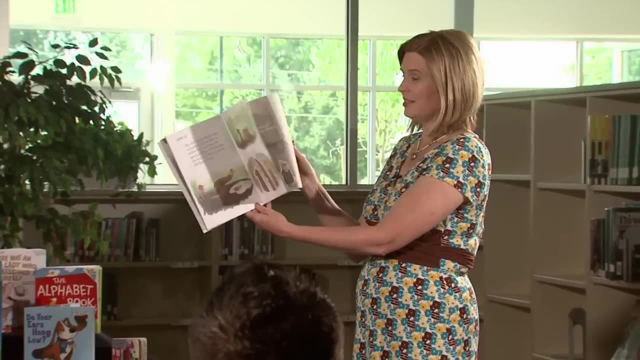 I told her that no matter how much time she spent looking in the mirror, her face always looked like her rear end. Spider thought that was really funny. Mom did not. July 4th. When I grow up, I want to be a Secret Service agent. 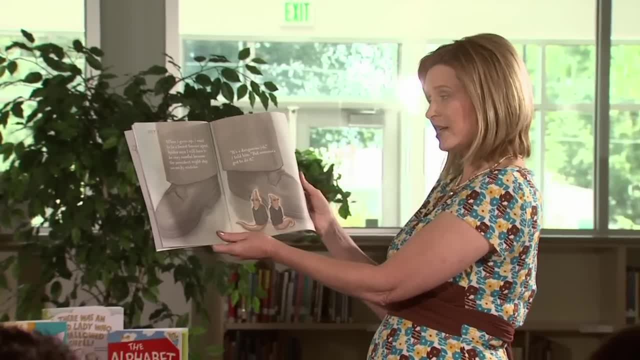 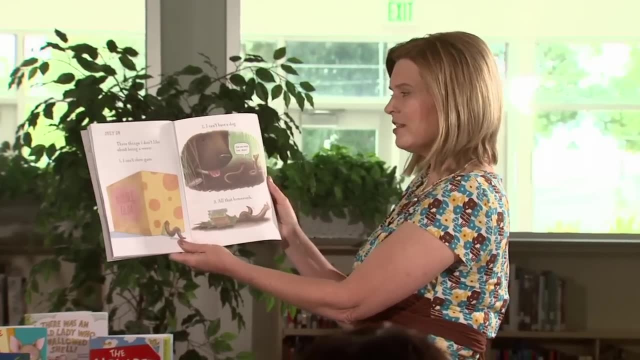 Spider says I will have to be very careful because the president might step on me by mistake. It's a dangerous job, I said, but somebody's got to do it. July 28th: Three things I don't like about being a worm. 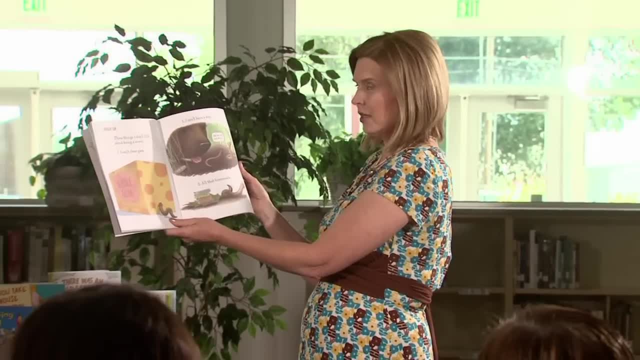 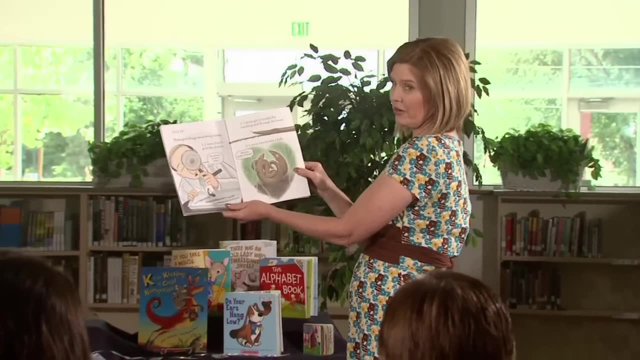 I can't chew gum, I can't have a dog- and all that homework. July 29th- Three good things about being a worm: I never have to go to the dentist, I never get in trouble for tracking mud through the house. 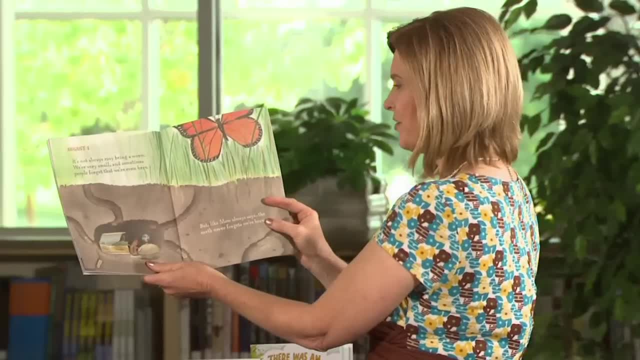 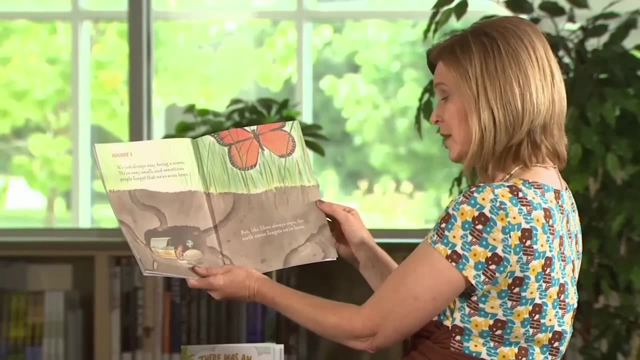 and I never have to take a bath August 1st. It's not always easy being a worm. We're very small and sometimes people forget that we're even here. but like mom says, the earth never forgets that we're here. 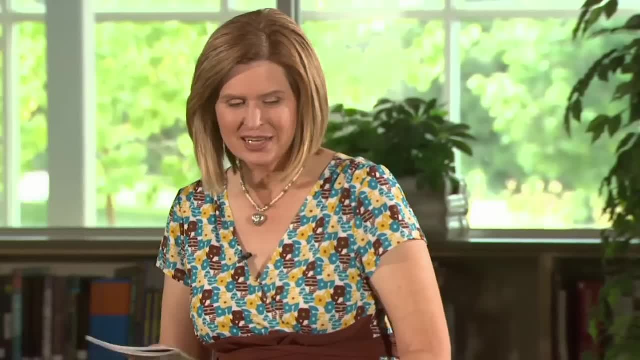 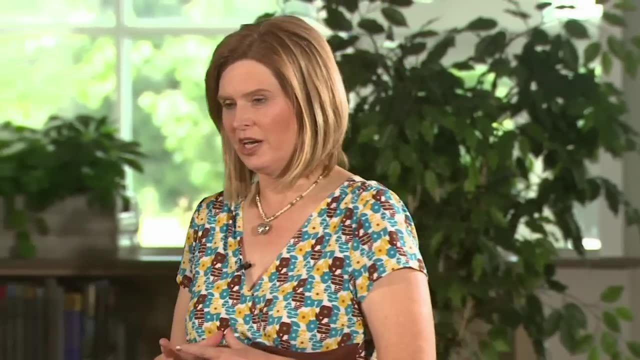 Okay, On your paper that the rest of the camera can't see is what happened first, what happened second, and then there's an activity of making your own story of a diary of a. you pick your own animal and then you create your own story. 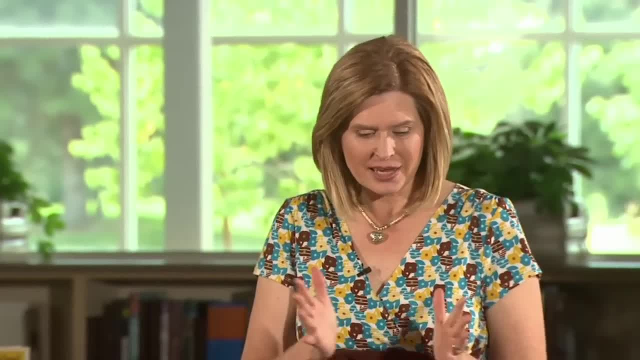 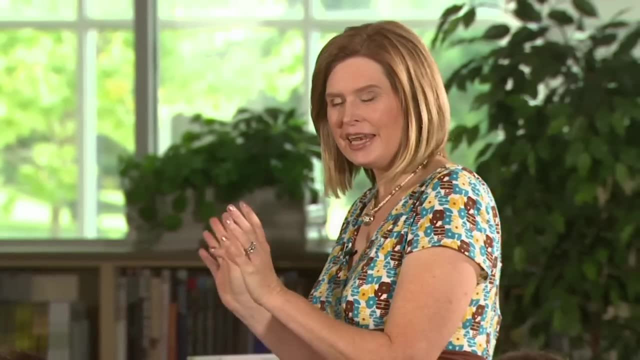 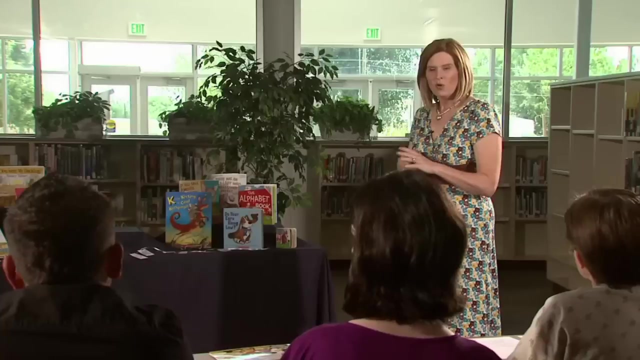 That's comprehension. Now, as we end this session, we want to see a little clip of comprehension, and it's from an almost an a-ha moment, or what does that mean? because that's what comprehension is. So, watching this clip as Word Girl gets that a-ha moment of 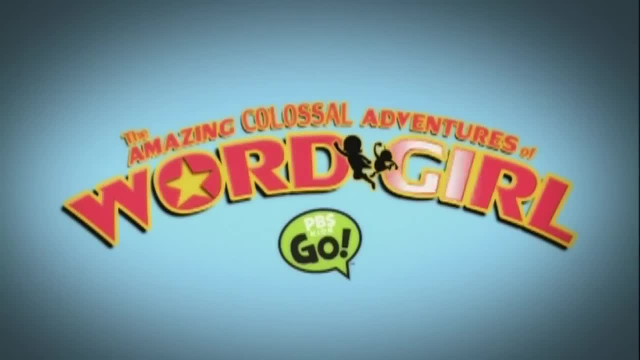 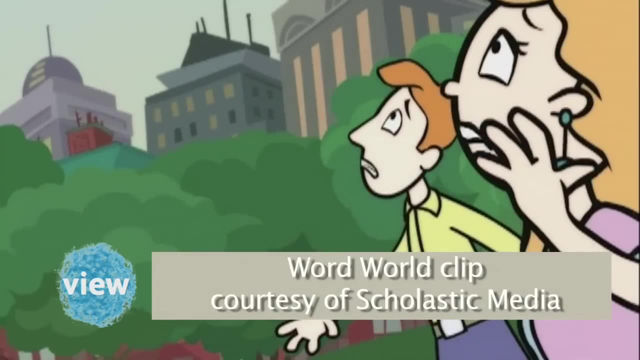 what does this mean, Word Girl? Deep in space, a chunk of space rock hurtling towards Earth at breakneck speed. Chunk of space Falling from the sky. We're doomed. Oh man, Couldn't this happen on a school day? 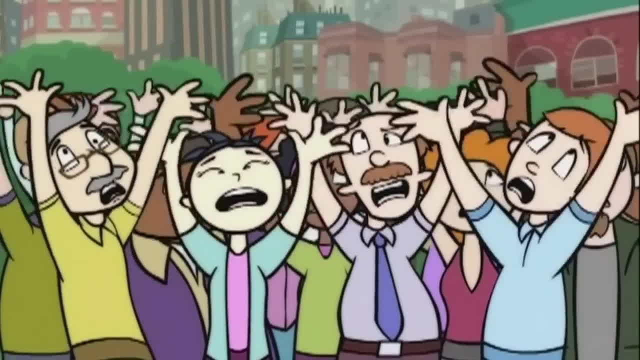 Who will save the city from this big hunk of space rock? Actually it's called a meteorite and I've got it Word up. It's Word Girl And Captain Huggyface. I know I don't like saying it either. 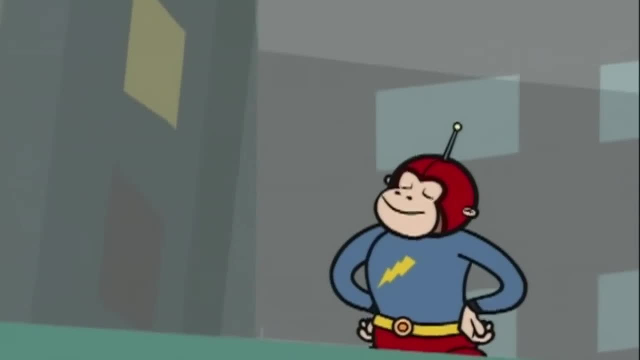 Intercept Hi Word Girl. Heck of a catch there. Thanks, I'm Scoops roving reporter for the Daily Rag. Mind, if I ask you a couple of questions, Shoot Great. First, how's it going Good? 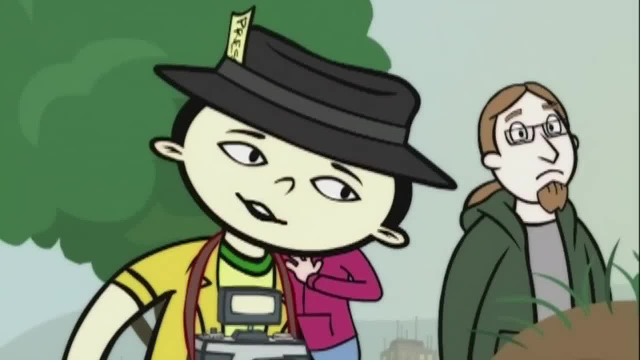 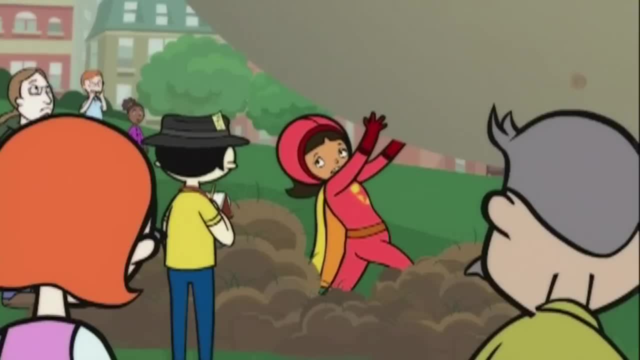 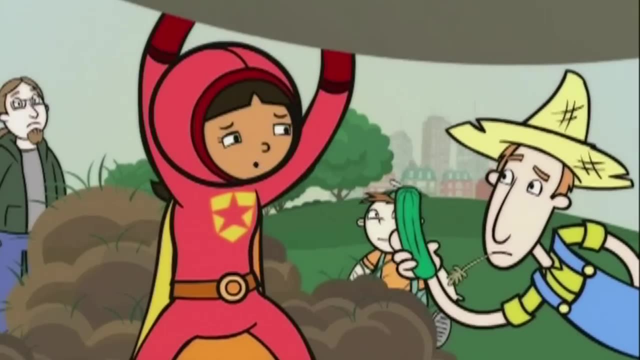 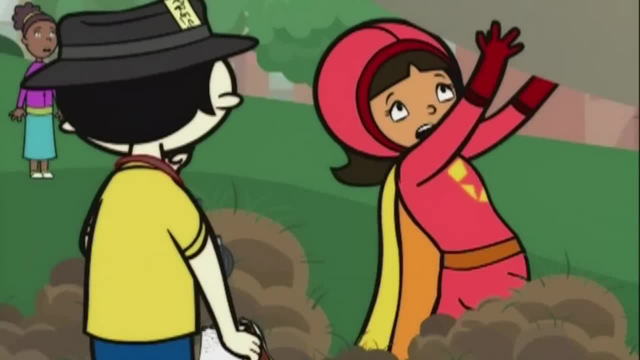 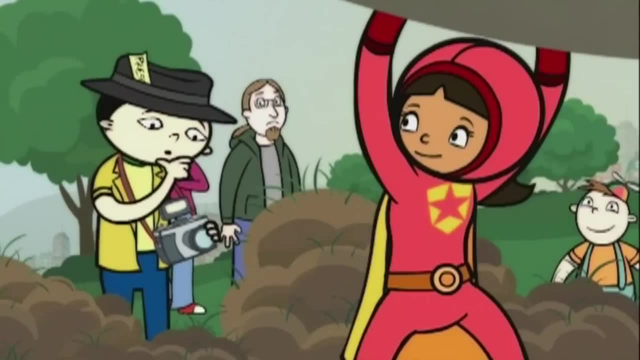 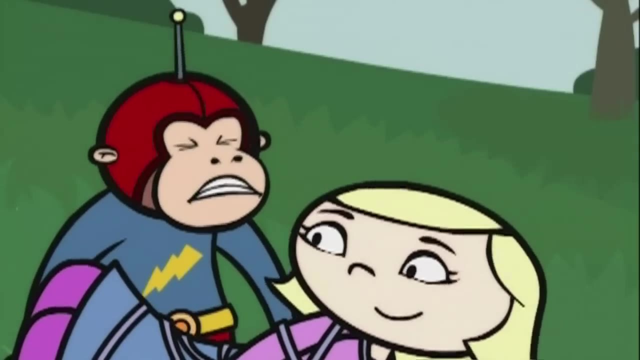 No, that's a cucumber. Cumbersome means bulky, heavy, hard to handle, Like that camera around your neck. Is that comfortable, Are you kidding? This pick clicker is breaking my back. Oh, cumbersome Right. And Captain Huggyface over there, he doesn't have super strength, so Violet is a little. 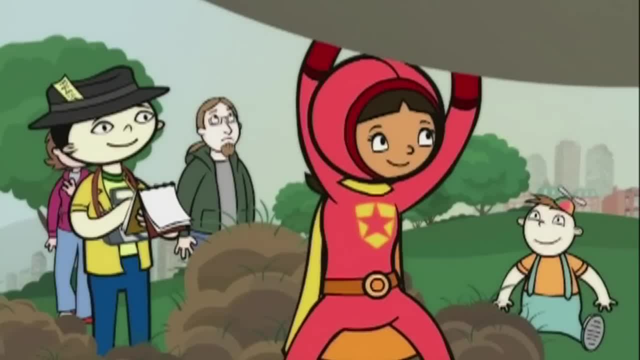 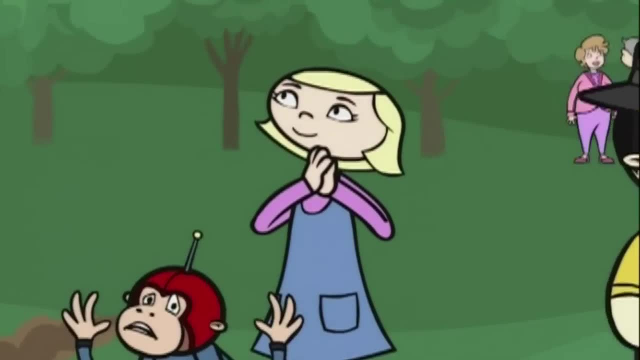 cumbersome. Oh, your fuzz tickles. I might as well get rid of this thing. My work here is done. Word up. Hmm, cumbersome Becky. Did I see what Word Girl? Oh no, I was um tying my shoe. 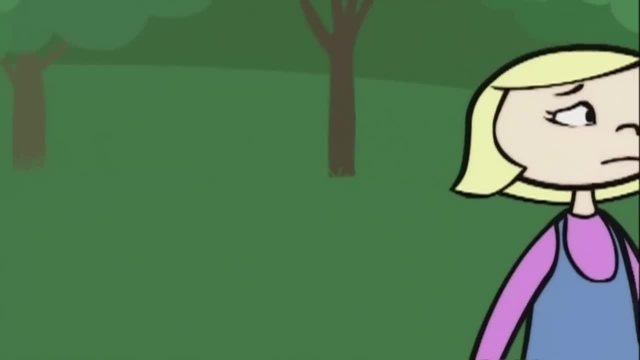 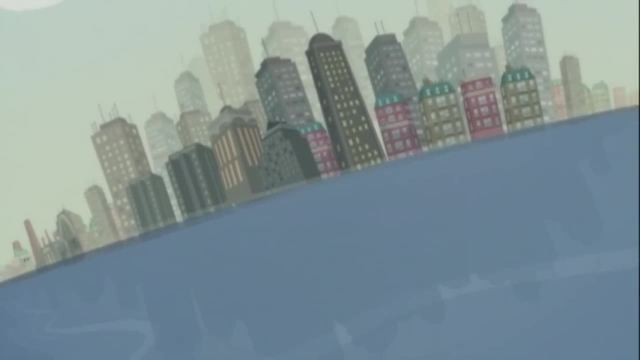 Come on, we're gonna be late for our art lesson. Who are you winking at? And so the city is saved from a cumbersome meteorite. all thanks to Word Girl. Oh, and Captain Huggyface. Tune in next time to the amazing colossal adventures of Word Girl. 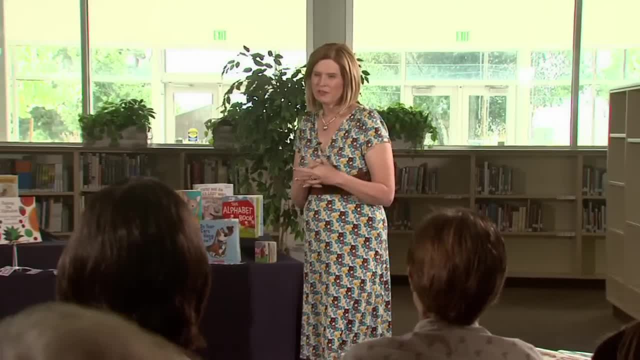 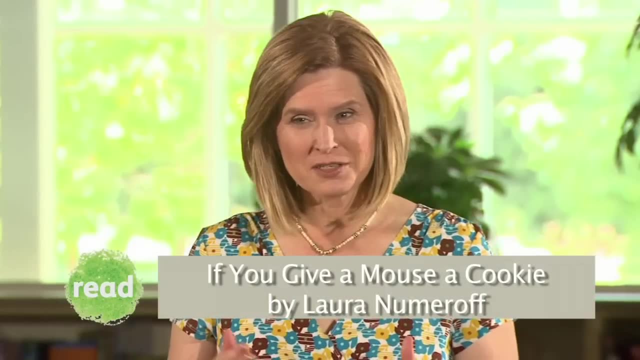 Hmm, that's comprehension, when you understand what you're either someone saying to you. you're reading or you're being read to. Most of you have read the book. If you give a mouse a cookie, he's gonna want a glass of milk to go with it. 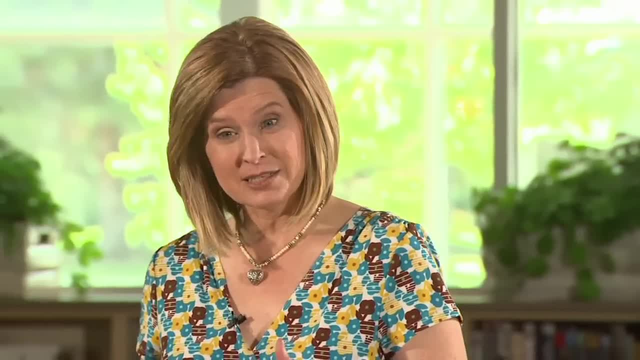 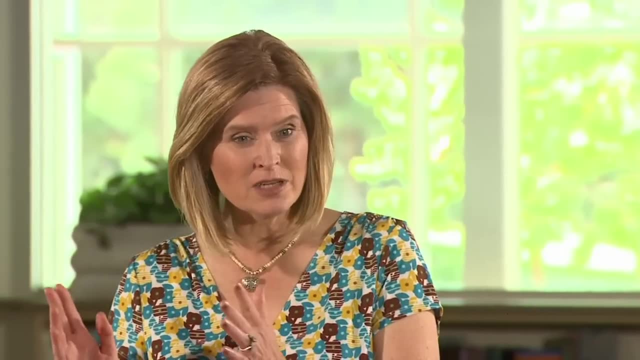 and then he needs a napkin to wipe his face, and then he noticed he needs a little haircut, and on and on and on. The one thing that I want to reinforce with that same thing: that if you talk to your children, if you let them talk, 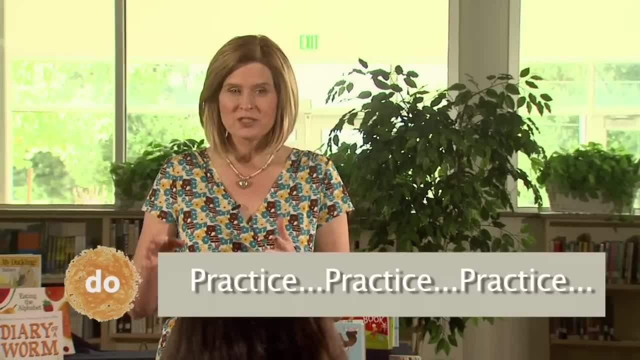 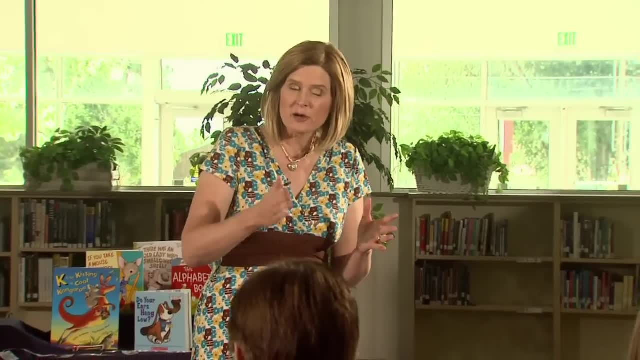 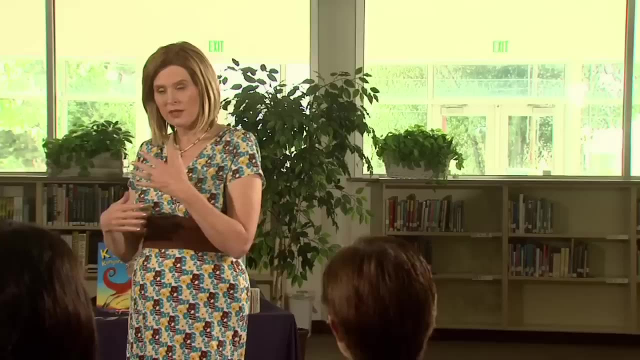 if you give them a lot of experience scribbling, looking at pictures, learning to write, then decoding, then those emergent literacy skills will have that domino effect of learning to read once they go to school. And so, as you do that, that sequence of one thing following another, 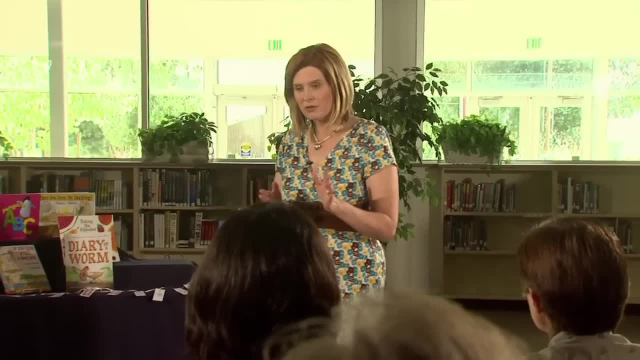 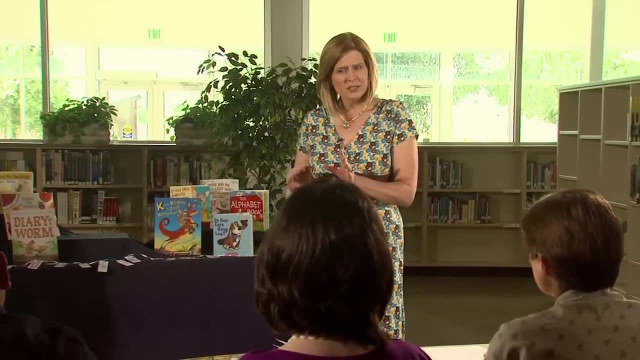 really reinforces the next: Make sure that you do that. You can start out with your children from the very time they're born, to talk to them. You've got about three years before they start talking back, so you've got a good, a good foundation of talking to them. 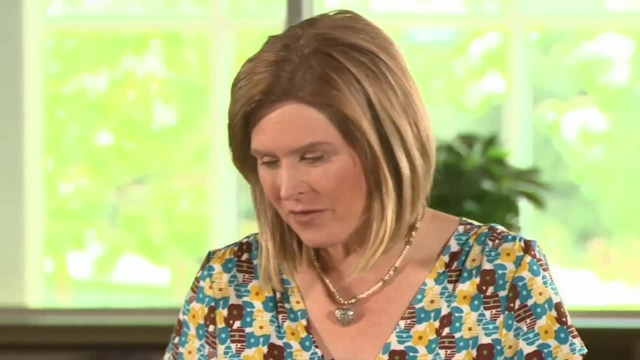 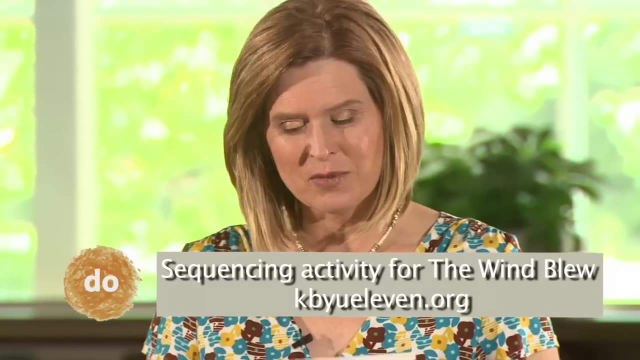 Don't forget to do that. Your last activity that you have in front of you is from the book The Wind Blew, and it is another sequencing story, just like if you give a mouse a cookie. My advice to you is to go to the library, find this book. 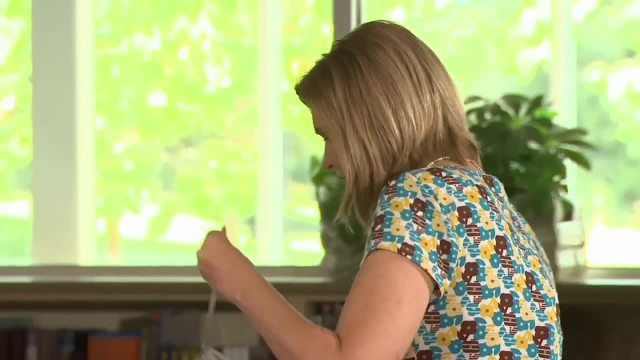 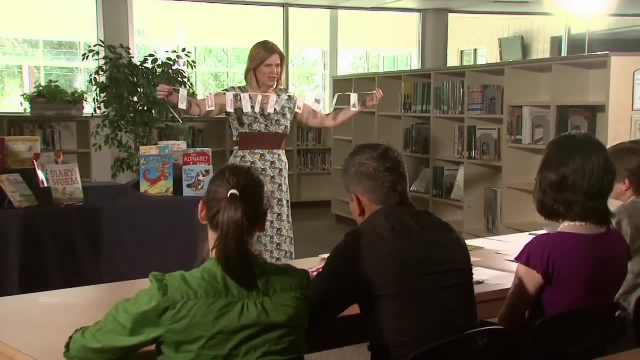 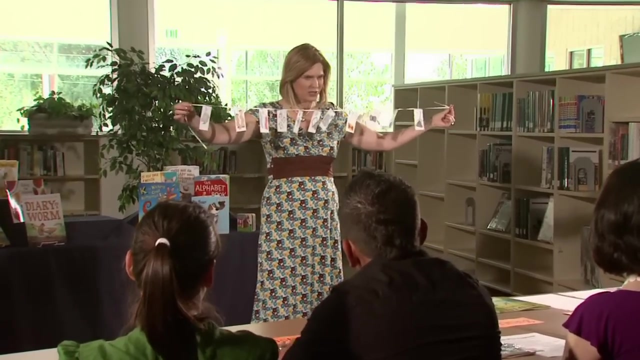 check it out and then, as you read it, you're going to see a sequence of events that happens when the wind blew. And as you read this to your children or your grandchildren, they can find the picture, the environmental print that goes with the story, so they can comprehend it. 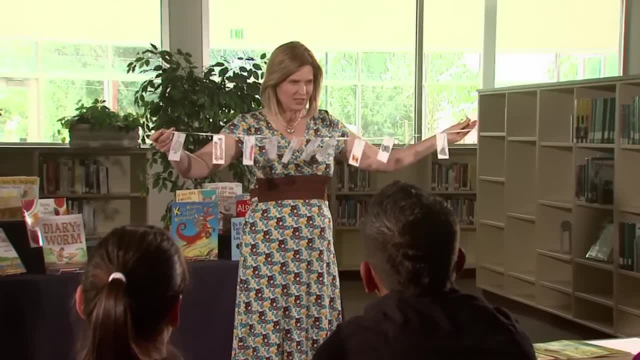 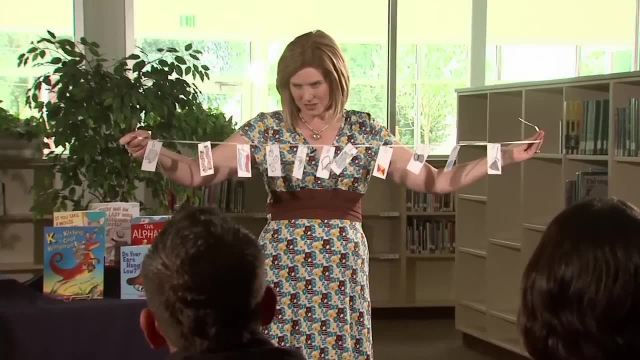 And it's a really fun activity. One thing that I would mention here is we do have paper clips that could be a choking hazard for a very young child, so be very careful with the age of the children that you're doing with this. If you're worried about that, then just let them have the pictures. 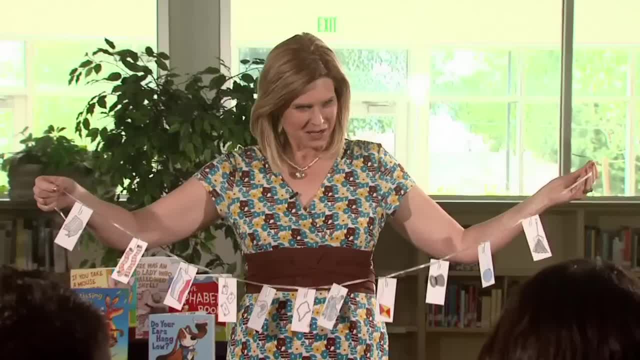 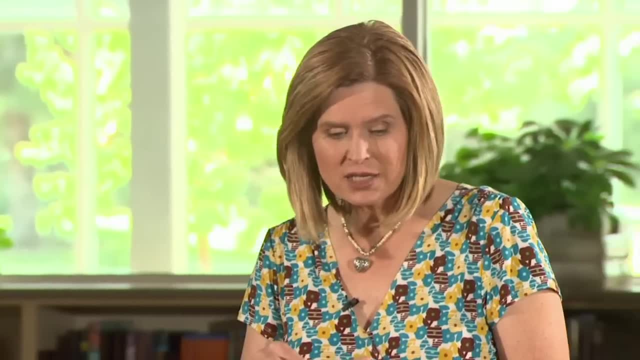 and let them say: then what happened? then what happened? That's a comprehension kind of story that doesn't need any words, like we did with the Diary of the Worm. As we've talked about our emergent literacy skills and as we've talked about Ready to Learn, 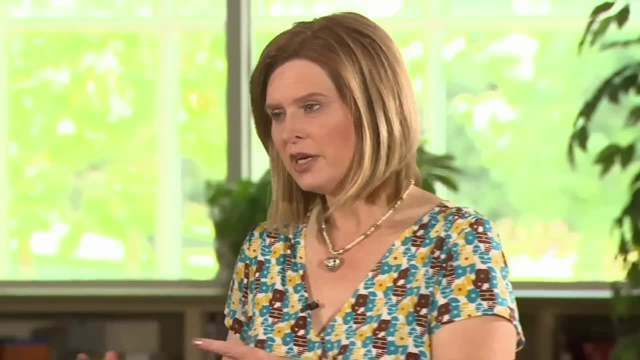 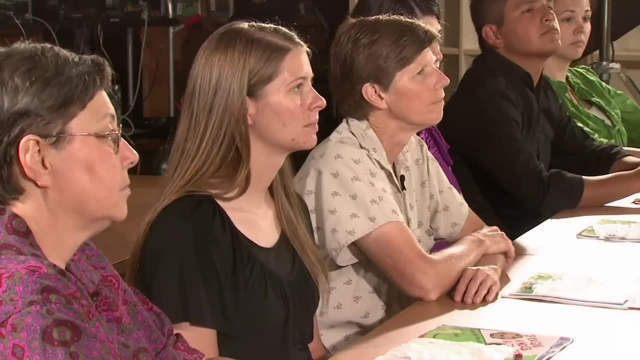 and we've talked about the best things that you can do with your children. remember, television is a tool, it's not the teacher. Use it as an educational resource, but don't think it's going to be the only thing that teaches your children. 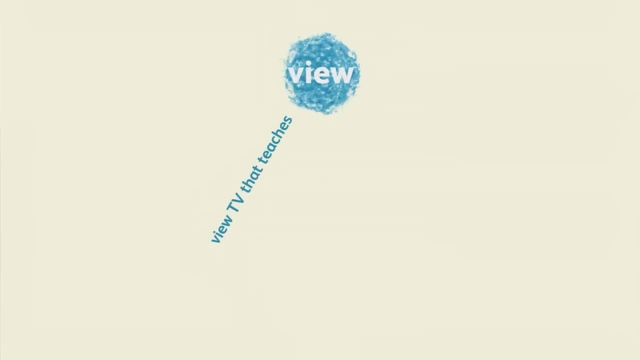 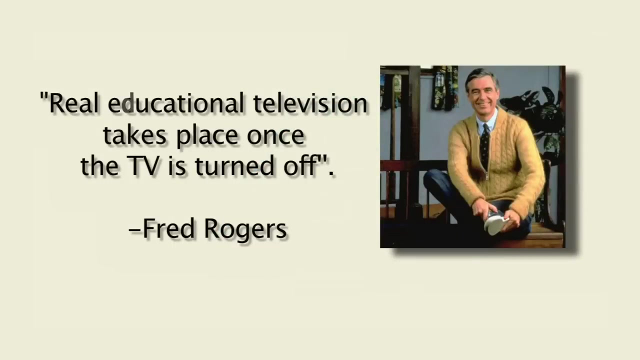 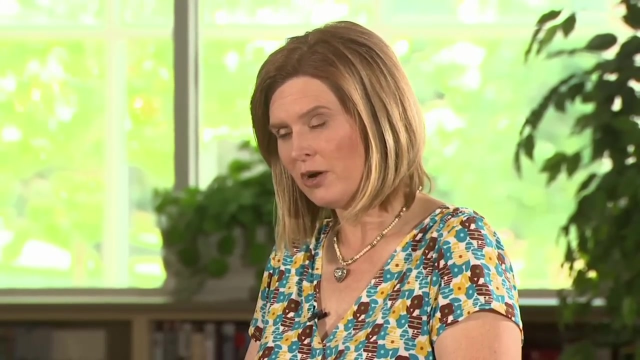 Remember the learning triangle: View a program, review the concept with a book and then do an activity. That's when television becomes educational is when you do something with it after it's turned off. Use television as a support for what you're teaching your children at home. 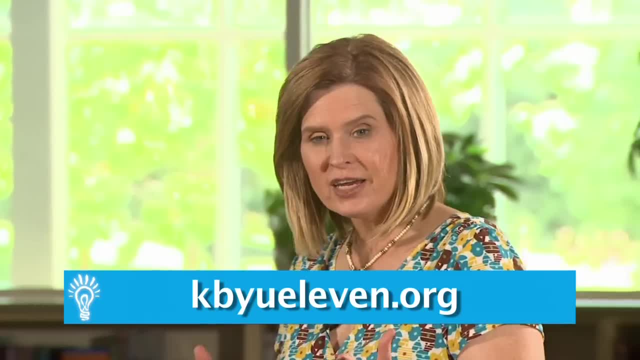 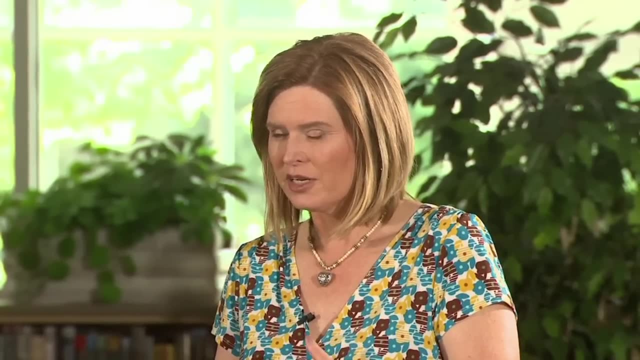 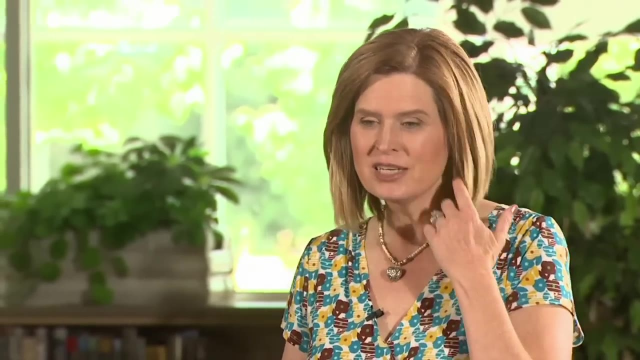 Go to kbyu11.org. find the shows that are appropriate ages for your children, and that will be the best experience that you can have with television. Television can be a wonderful teaching tool for you. It can also be a great source of entertainment.